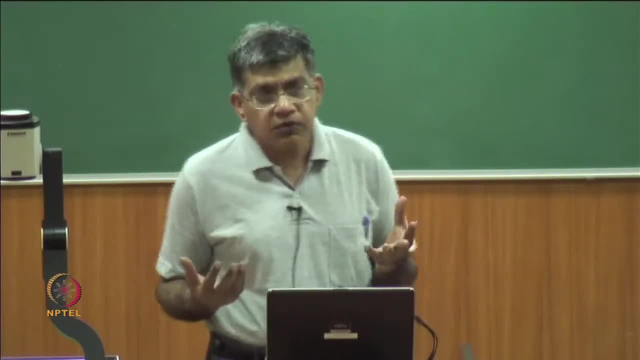 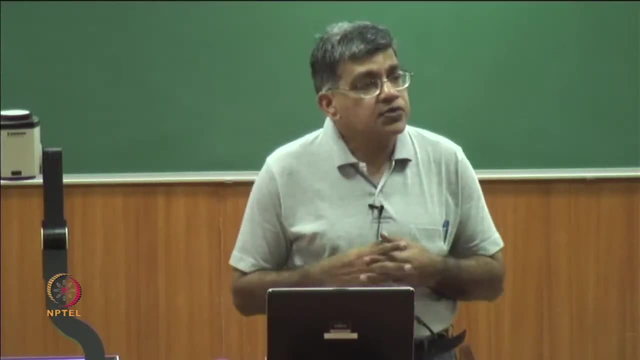 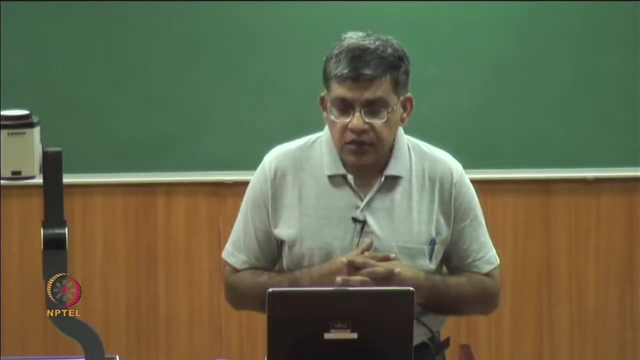 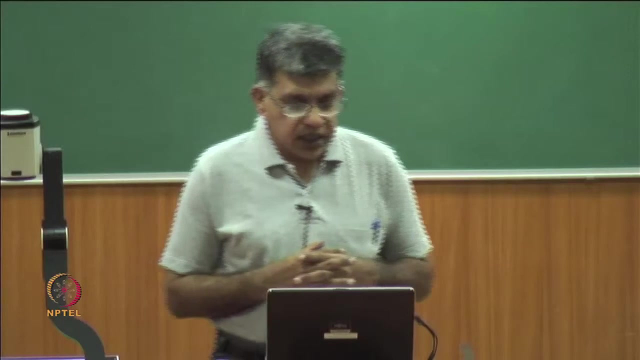 and it is not clear whether lots of new theorems have been proposed. lots of new proofs have come up And lots of generalizations, especially like in analysis and algebra, and the important question that was that was bugging Hilbert at that time was: that is all of mathematics. 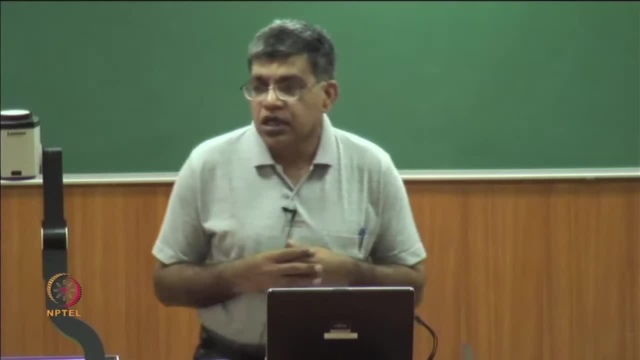 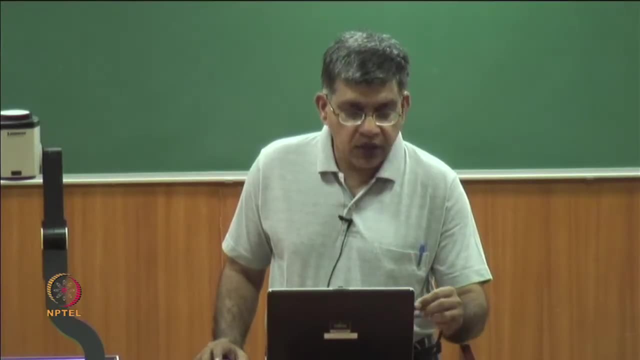 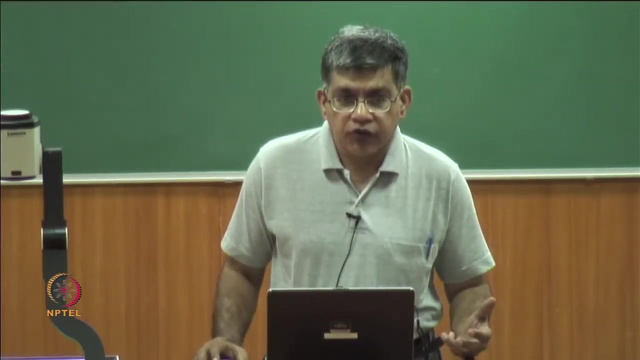 somehow internally consistent, And Hilbert's program was designed was essentially a question wanting the mathematicians to address this question of: is all the mathematics that we are developing actually consistent, Because there is a danger that you can prove a lot of theorems. 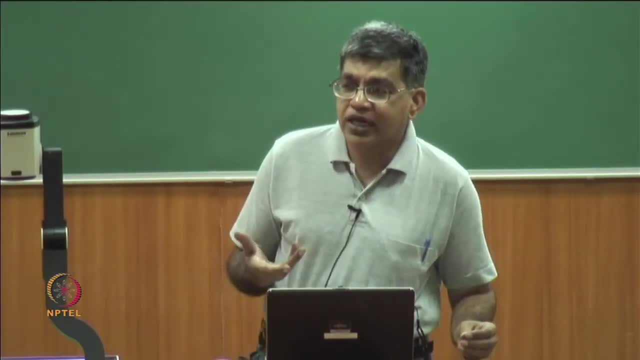 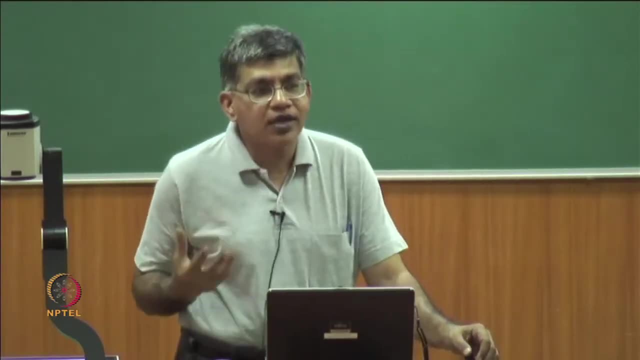 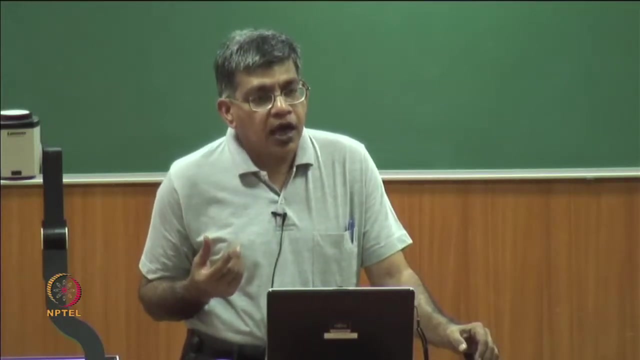 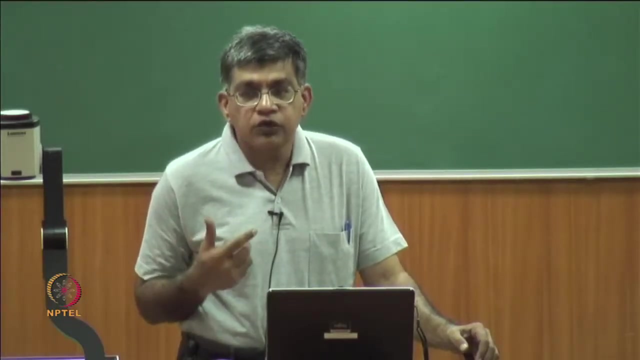 if you are internally inconsistent. In fact, you can prove practically anything you want if you are completely inconsistent. So the over writing question was whether mathematics was internally consistent And therefore the over writing question was: as a consequence of that was to actually axiomatize mathematics In such a way that you could rewrite and reformulate. 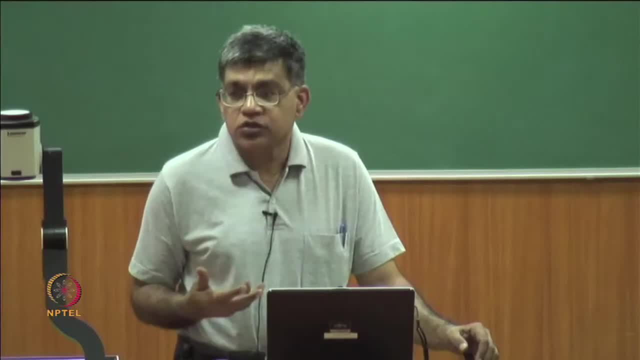 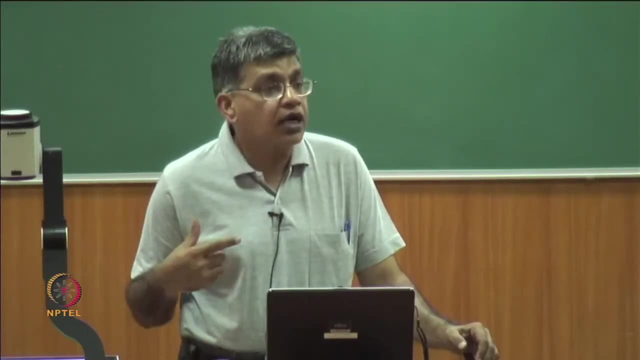 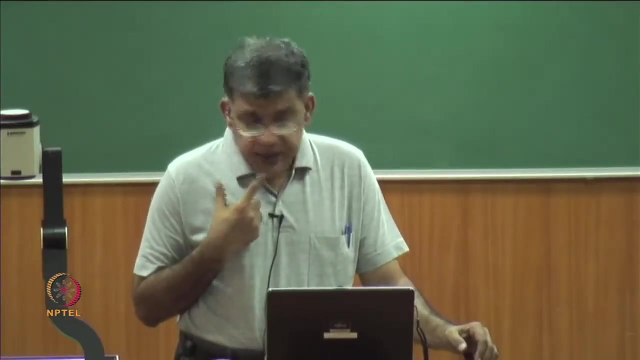 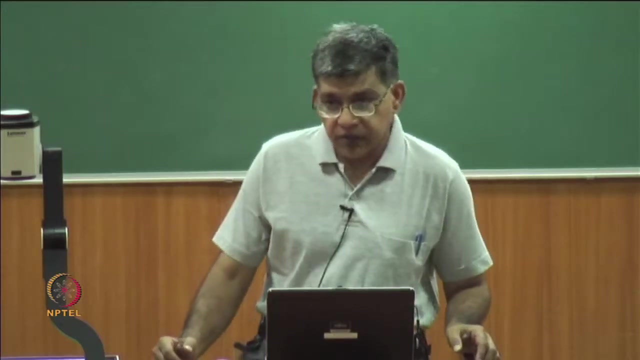 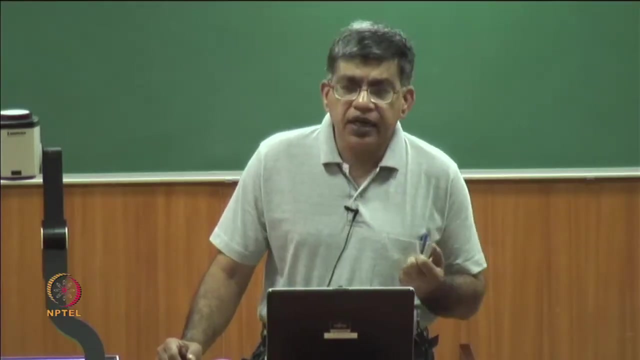 all the branches of mathematics starting from some foundation in a non circular fashion And therefore and then at least establishes consistency in some way. So that was one. that was one thing. and the second question of Hilbert's program was, if you were to algebraize mathematics, how much of it can actually be done in some mechanical? 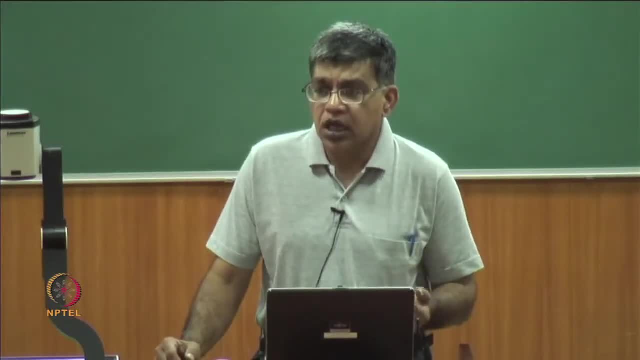 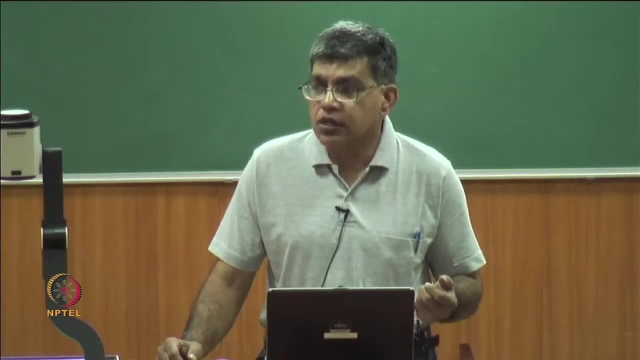 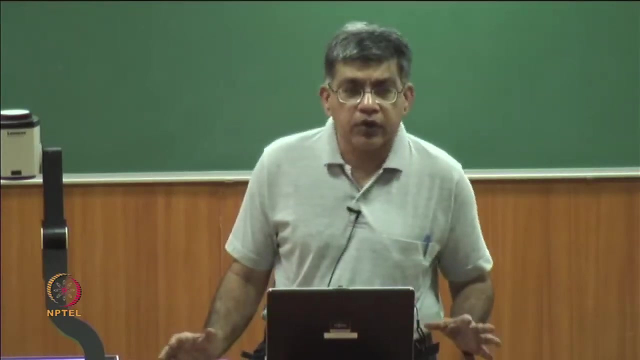 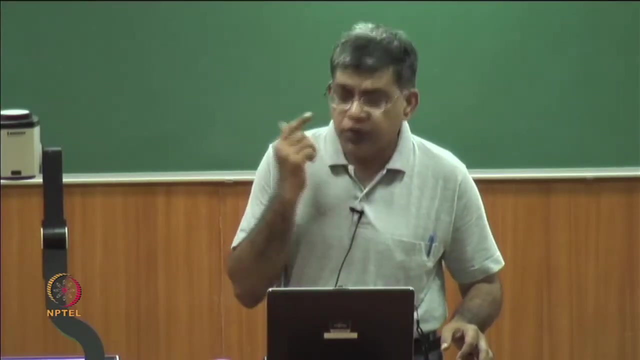 fashion, essentially by a machine. How much of it can actually be automated? the, what can you prove? So these are the theorems in some automated fashion, both the notions of, So both of these questions which formed important parts of Hilbert's program of about 20 questions, Hilbert. 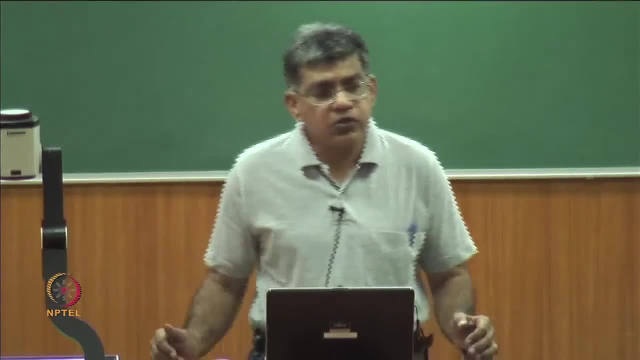 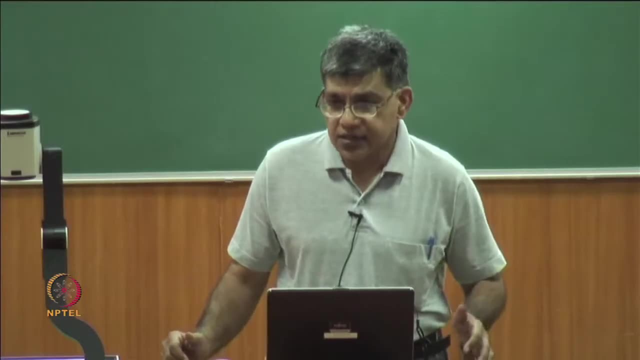 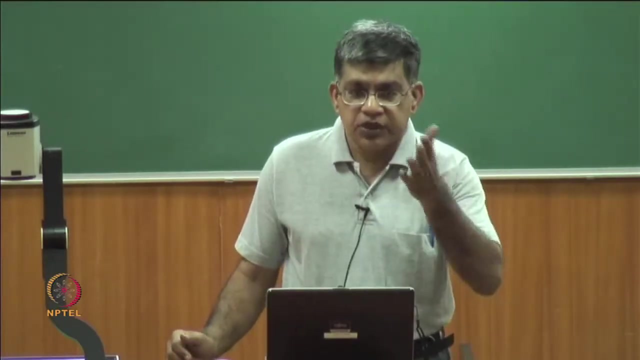 of course, was a great, all rounder kind of mathematician, So his 20 questions addressed to the world congress of mathematicians included problems from other areas right like So, ranging from number theory to algebraic geometry, through and differential geometry, all though way through. 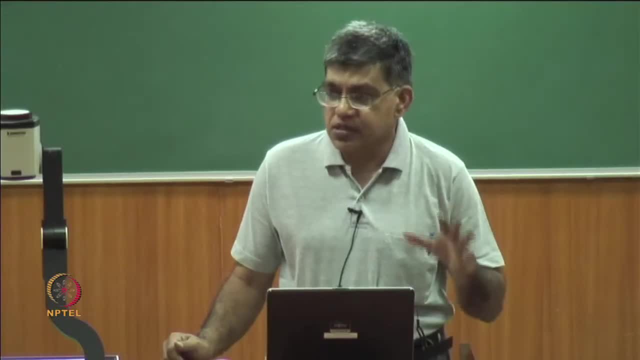 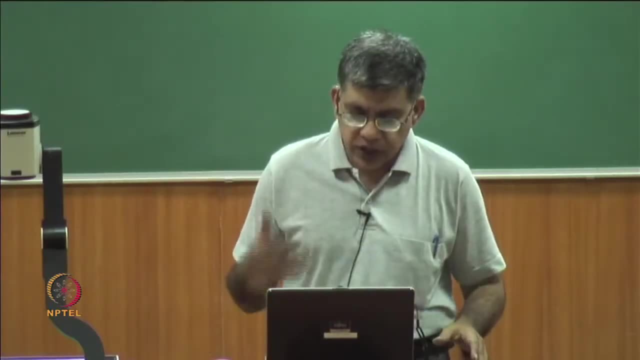 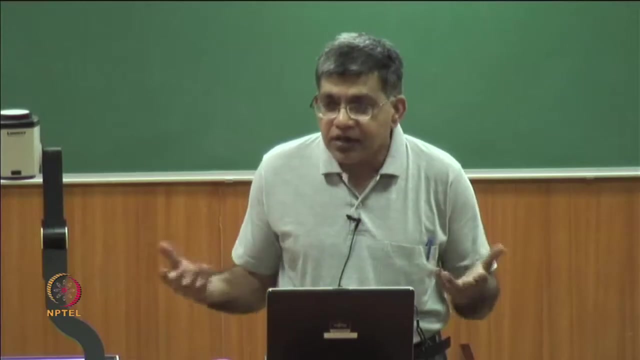 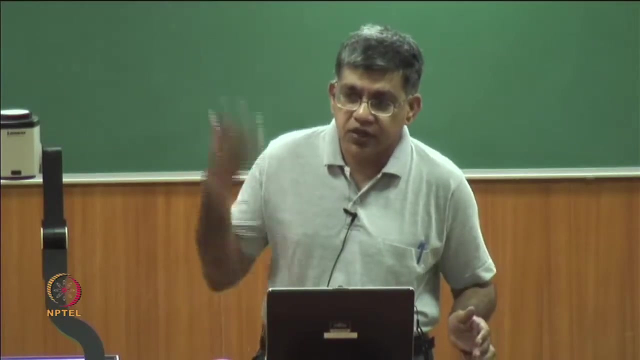 Hilbert spaces, on and so on, so forth, And thus included things like rainbow and the continuous hypothesis. He including a lot of starts, and Hilbert, as the mathematician, was actually empowered because of his all round contributions to various branches of mathematics, starting from number theory to algebraic geometry, to Hilbert spaces and 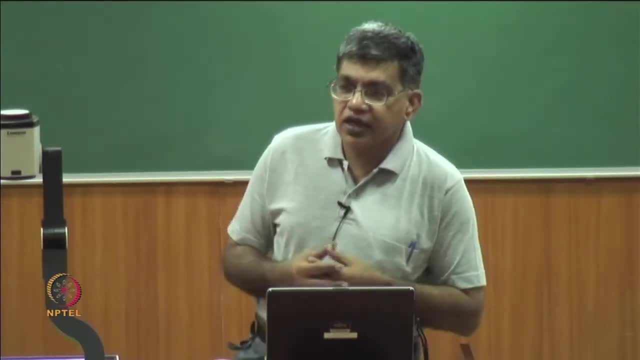 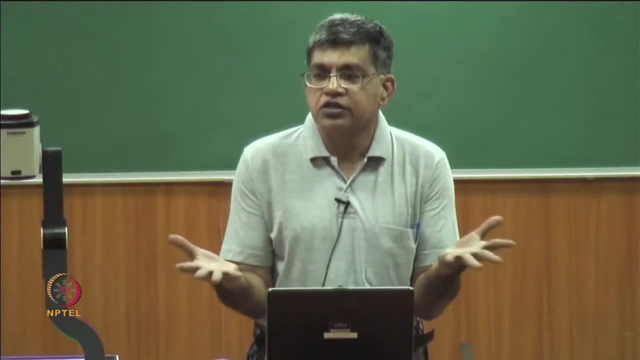 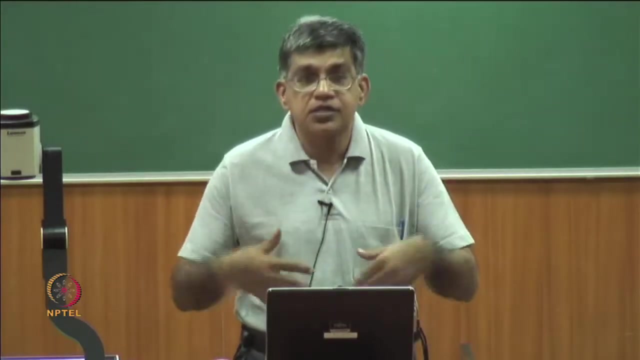 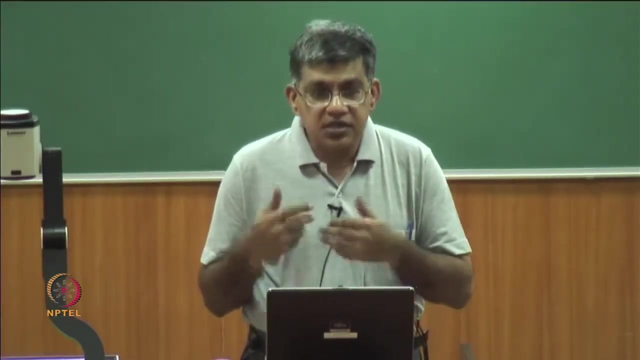 to parts of physics. So he was peculiarly situated and able to address the question of whether this entire body of knowledge is consistent. is it possible to give it a consistent formulation So that no inconsistencies can be shown? firstly, is it consistent? secondly, can it be reformulated in such a way that no inconsistencies can? 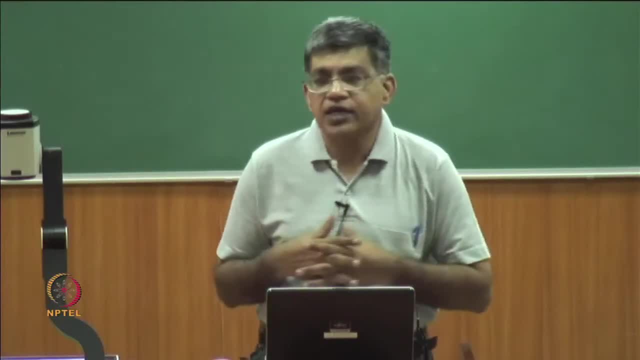 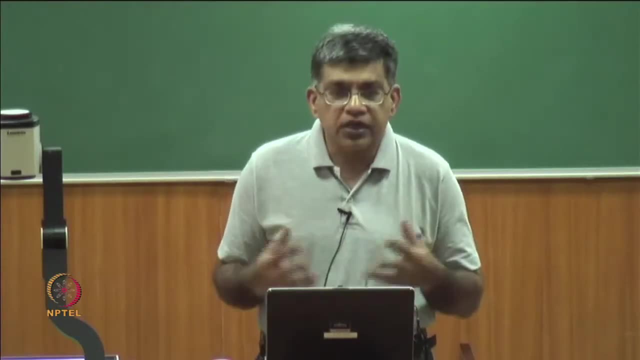 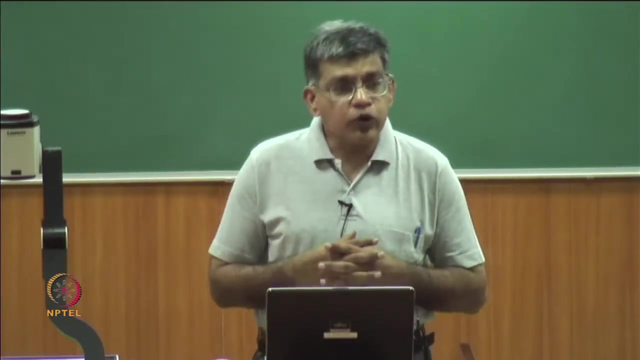 be shown. And thirdly, the question is how much of it can actually be automatable. I mean, is it possible that if you can automatize, you can automate the, if not the stating of theorems? can you automate the proofs of theorems and 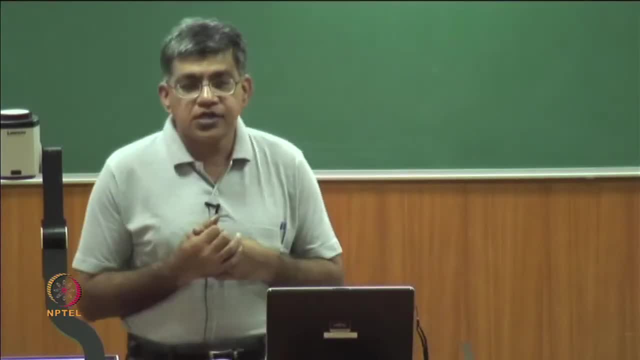 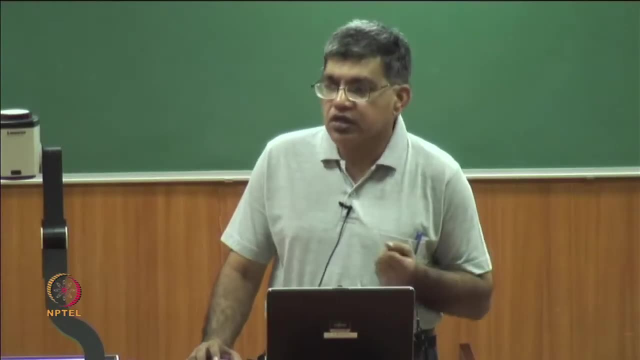 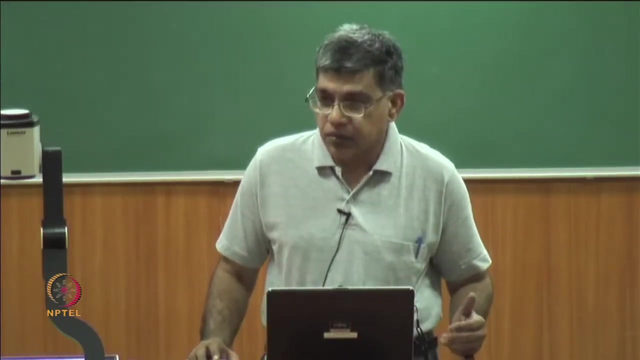 can the question of proof be automated, Since a large amount of proving of an algebraic nature involved essentially symbolic processing? the question of whether it can be mechanically evaluated and proofs- whether proofs can come mechanically- was a question that bothered Hilbert. The result of Hilbert's program and the questions. 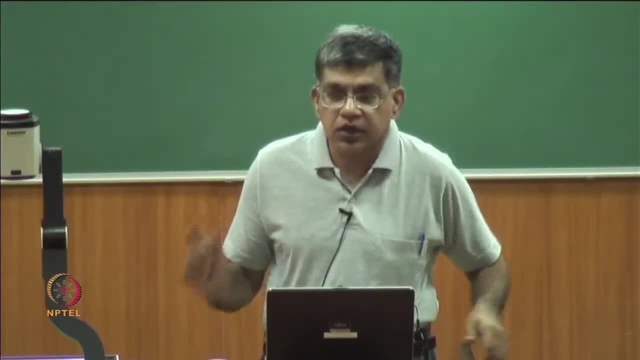 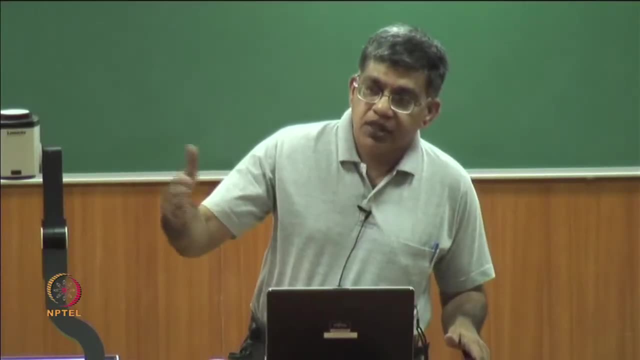 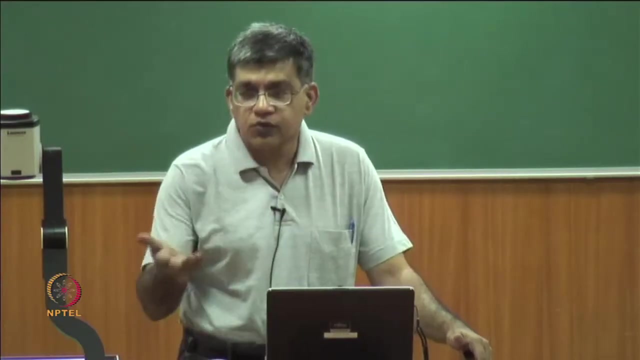 he raised in 1901, 1900 or 1901 World Congress of Mathematicians was actually that it did guide the development of logic and mathematics essentially through the 20th century. So and it gave rise to these notions like computability. So one of the most important 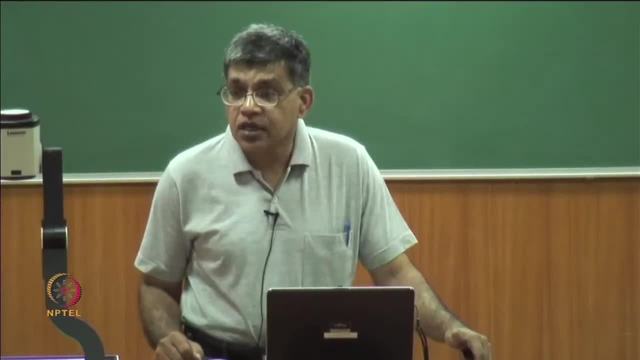 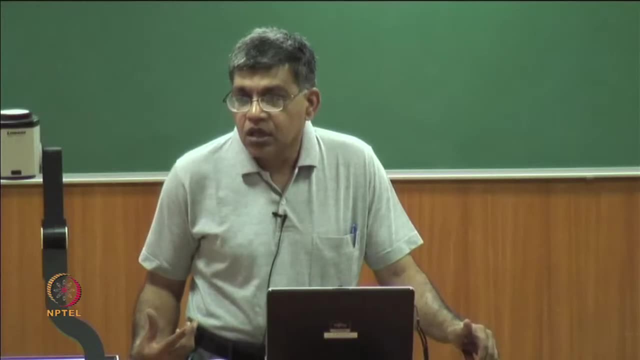 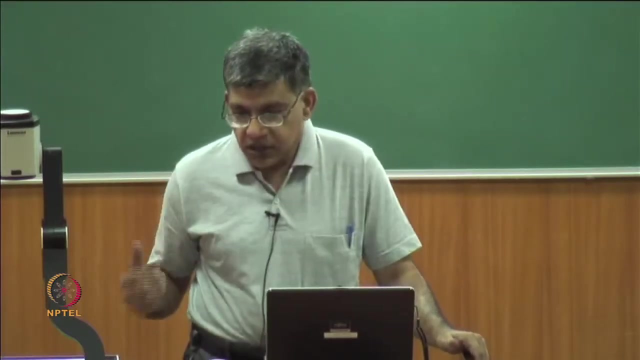 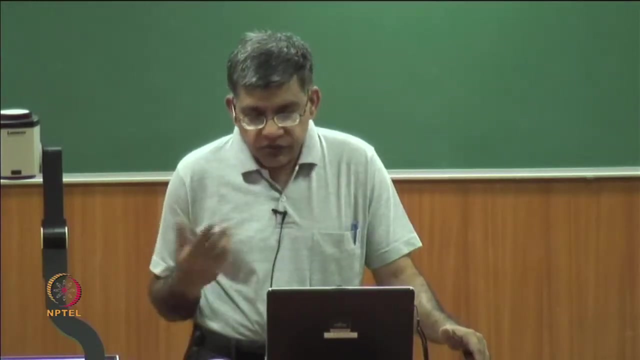 and landmark results was assuming a notion of mechanical evaluation without actually having any formal model of it. except what was? It was made very difficult historically through, let us say, the works of Babbage and Pascal and Leibniz, except for that, So there. 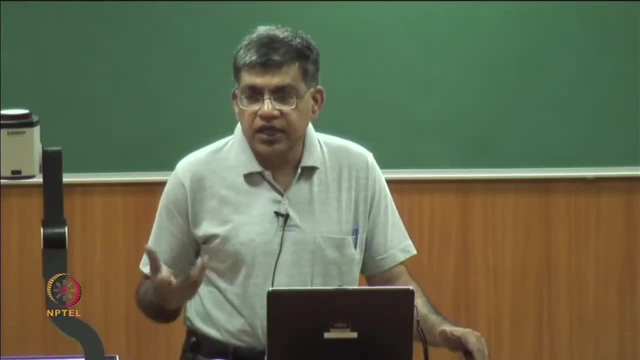 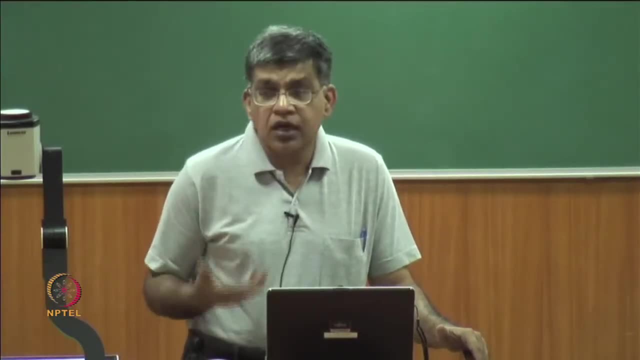 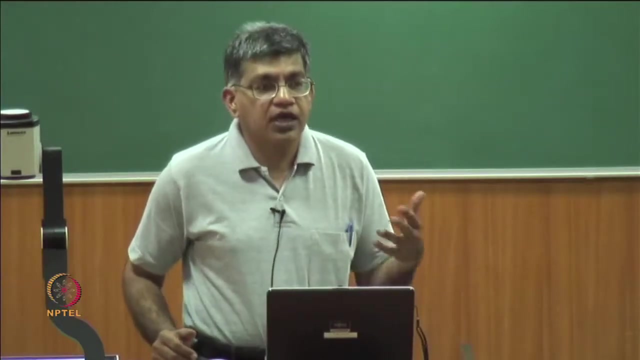 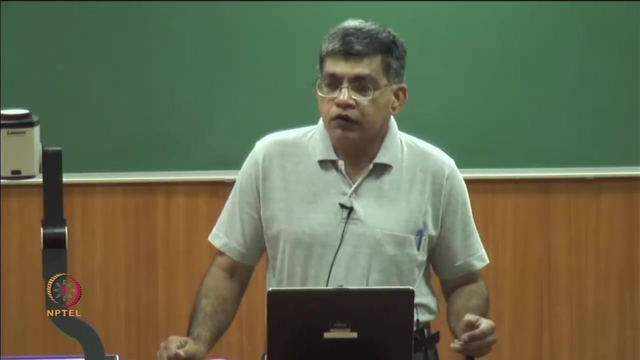 is the famous proof by Kurt Goodale which first showed that first order logic is the Hilbert proof. system for first order logic is essentially consistent and complete And when you apply it to something like number theory, essentially through piano piano arithmetic, there are propositions which cannot be decided by machine. basically, 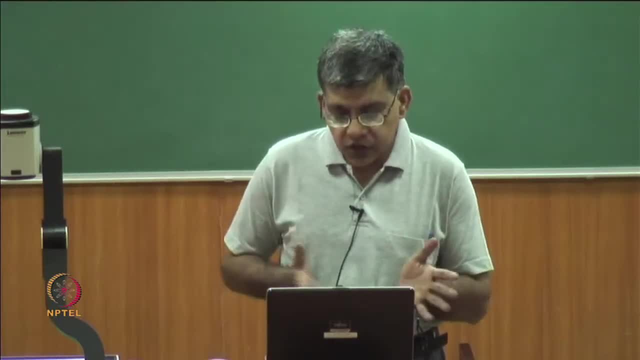 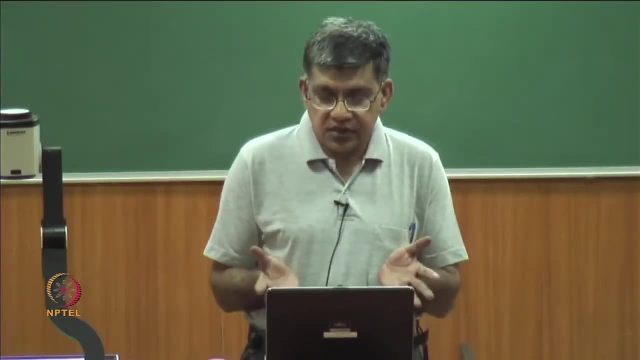 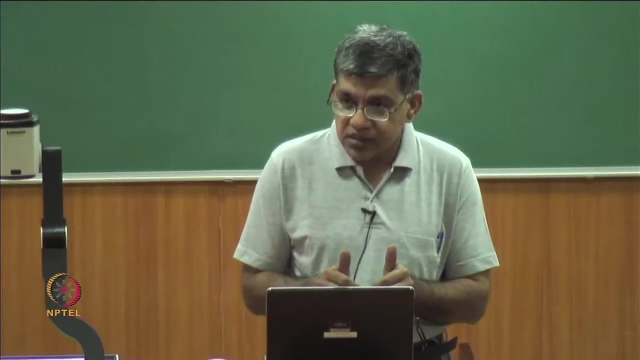 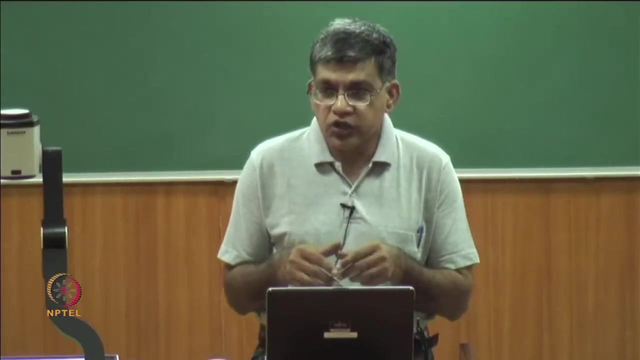 And that there are theorems. so he linked the notions of consistency, completeness and decidability in such a way that if number theory is consistent, then it is not complete. and by using a technique known as arithmetization he also showed that if number theory is, 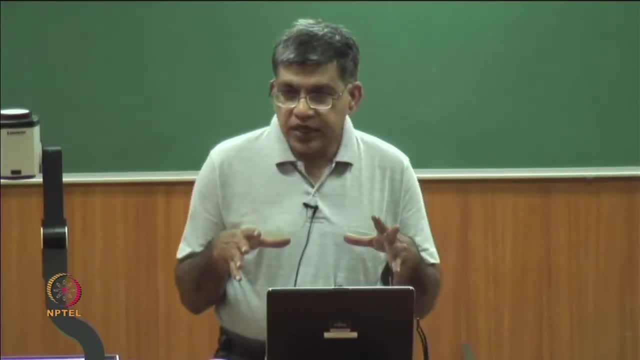 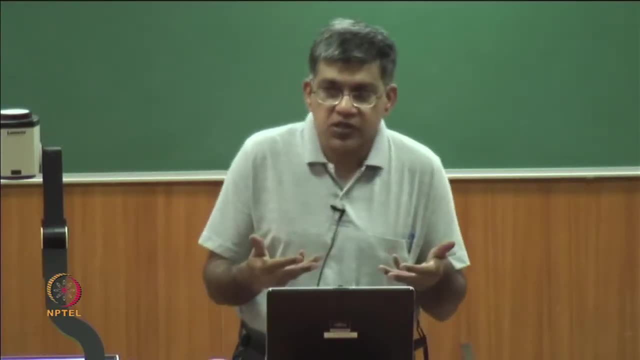 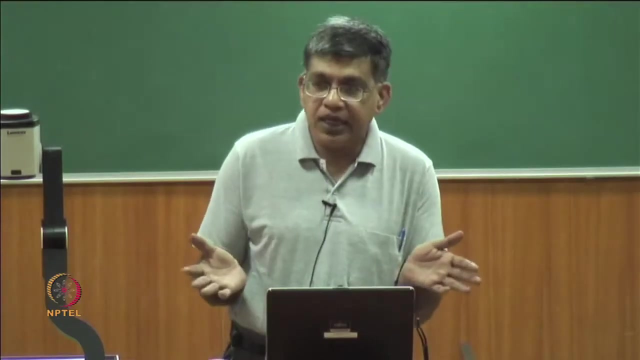 consistent. so the consistency and completeness of first order number theory was dependent on whether the first order logic that was used to describe number theory is itself consistent and complete. So Gödel proved that first order logic itself. if you looked at it independently of its application, its axioms are consistent and complete. but when you 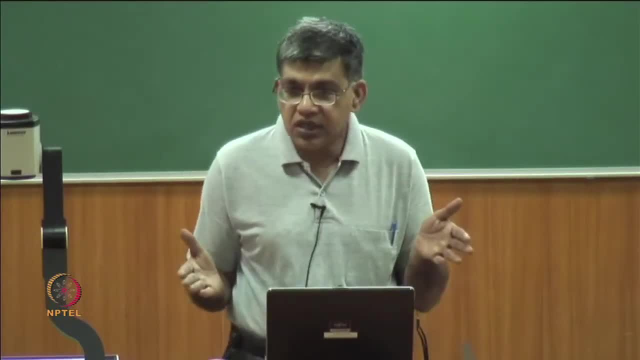 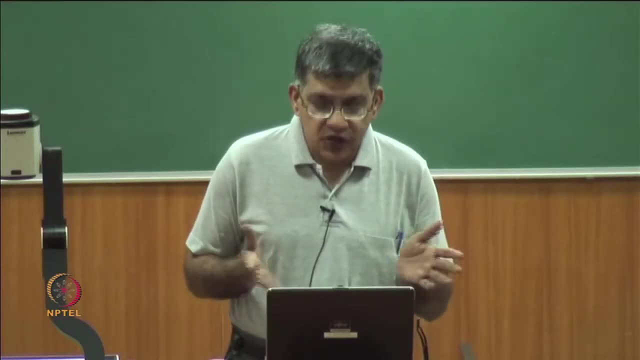 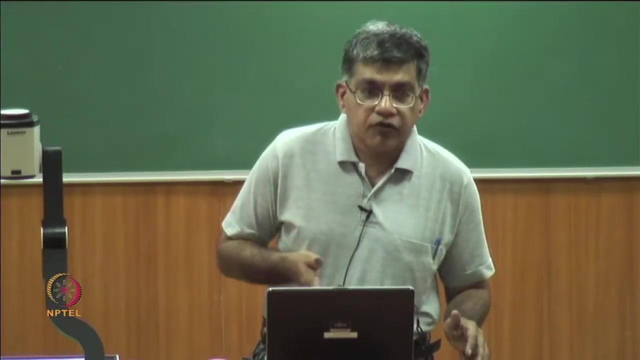 applied it to number theory to get what is known as first order number theory, that is, if it is consistent, then it is not complete, And by a notion of arithmetization of syntax, he essentially showed that it is possible to have theorems in first order number theory which cannot be, which are not decidable by 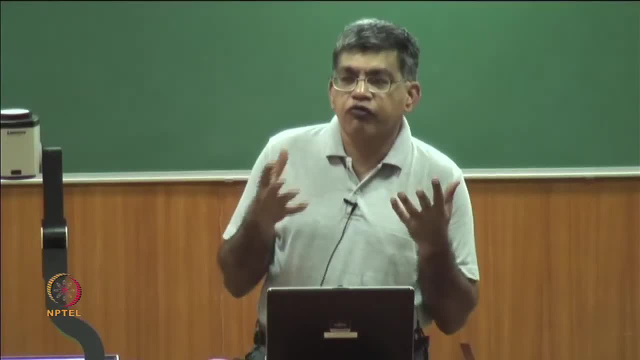 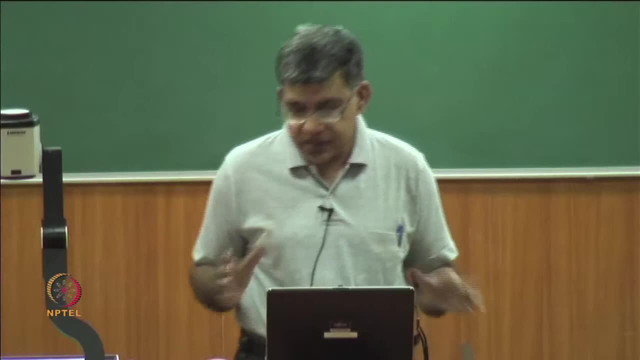 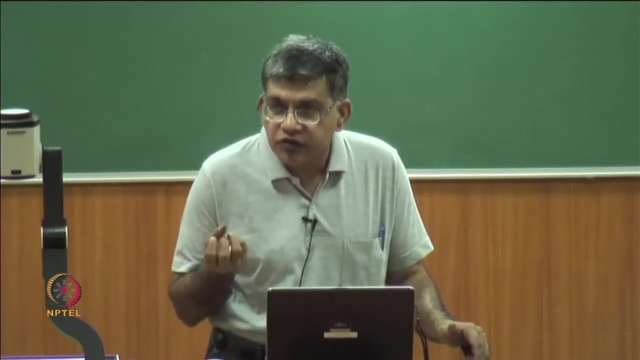 any mechanical means. I mean so even before the notion of, even before the formalization of exactly what is a mechanical means of computing, Gödel could actually come up with this landmark kind of result, And after that came the notion of formalizing the notion of computing from. so the works. 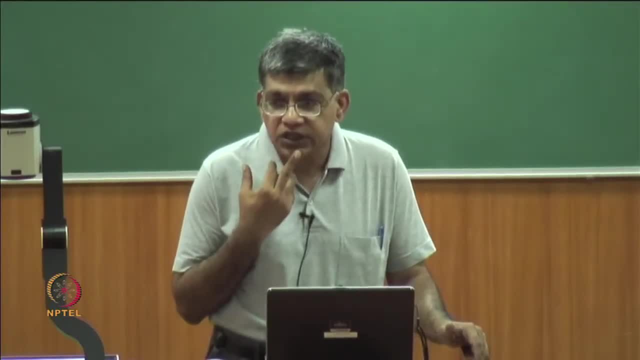 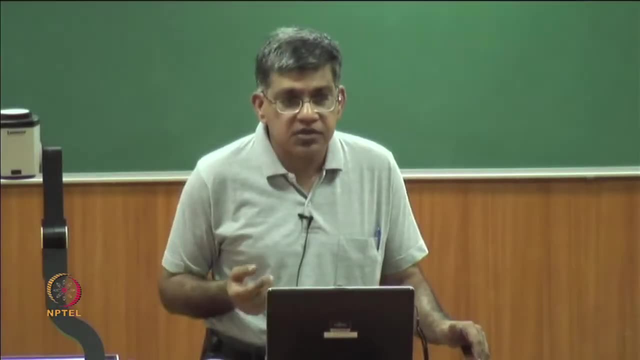 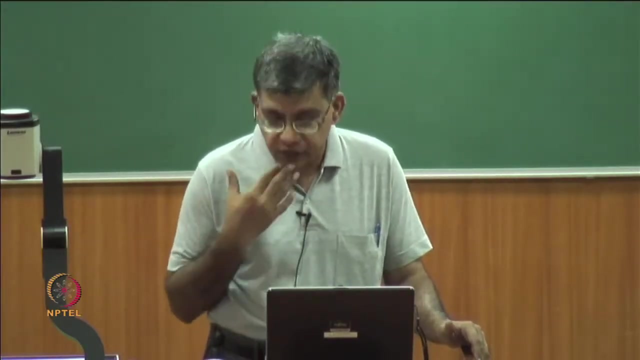 of church, basically the lambda calculus and combinatory logic, and after that the Turing machine, after that the proof that all these different model Markov algorithms, after that the proof, The proof later, that all these machines, all these models and machines are actually equivalent in their power of mechanical evaluation and therefore, so you can see that it has actually 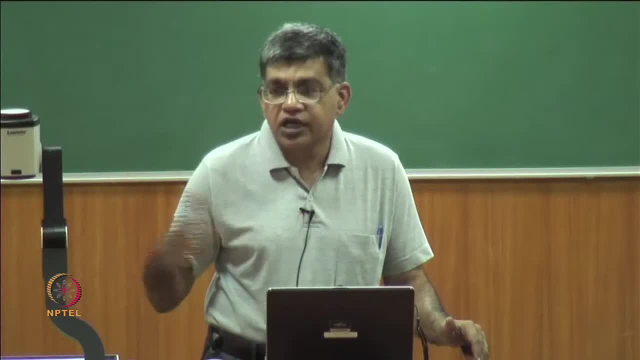 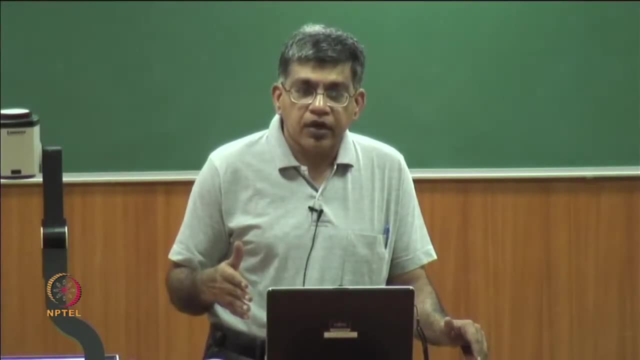 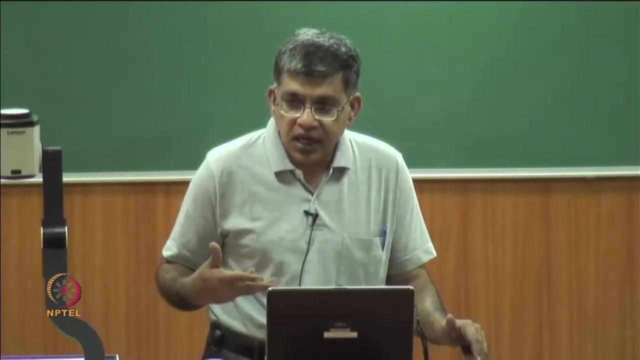 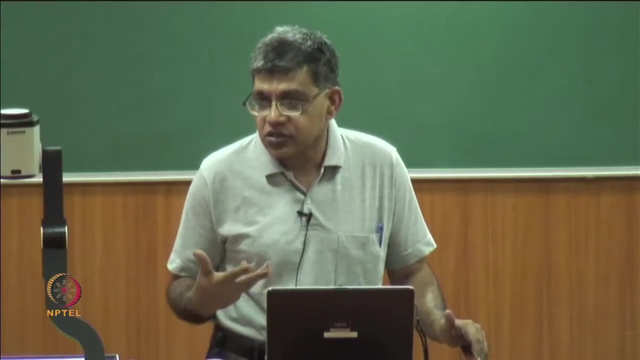 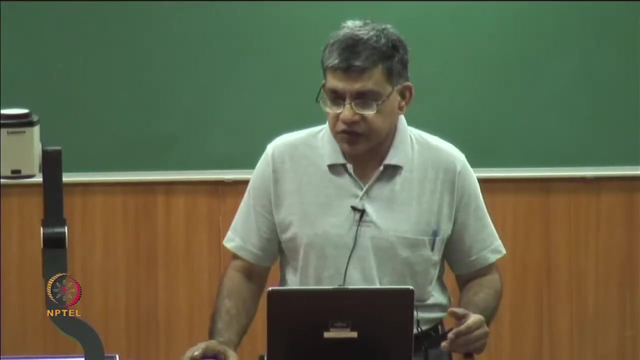 dominated a large part of logic and computer science, And it dominated mathematics to the extent that the fields like topology and analysis were formulated, in some in an axiomatic fashion, after Hilbert's talk, essentially So, the formulations of statistics by Kolmogorov, the formulations of topology by Korotowsky. 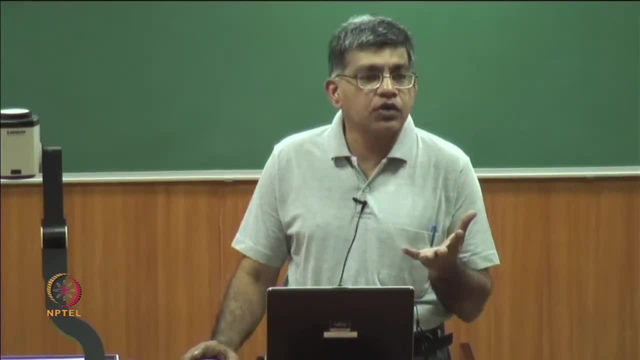 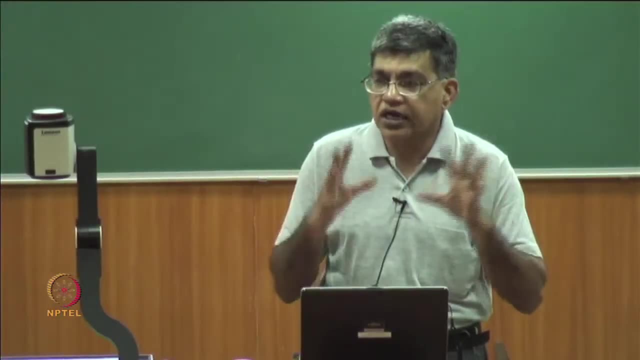 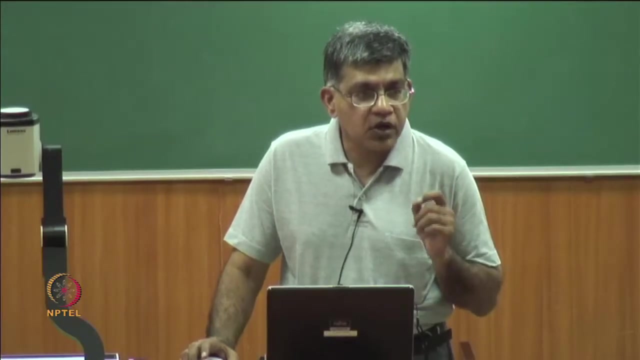 and so on and so forth, as axiomatic systems essentially came up in the 20th century, and before that they were essentially disparate pieces of mathematics and it was not clear how they all fitted together. So the notion of models therefore becomes important. so this is a model, essentially. 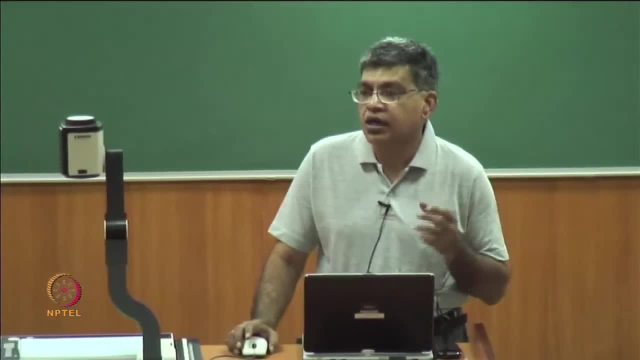 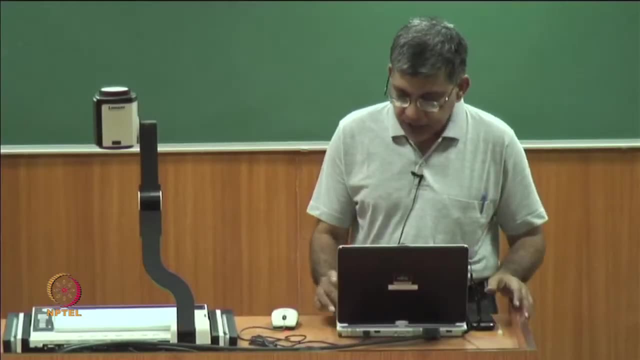 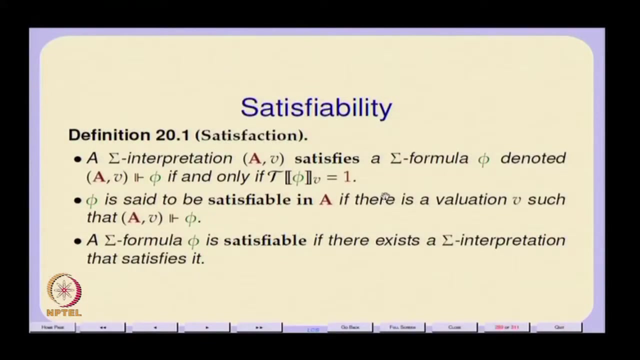 will be as a theory, a mathematical theory for which you are going to give some axiomatization, for example. So we look at that, the notion of models, but before that we have to look at basic things like satisfiability. so the notion of satisfiability is, of course, very simple in the in the case, 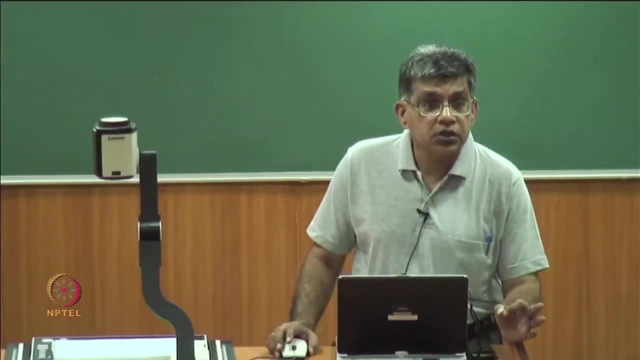 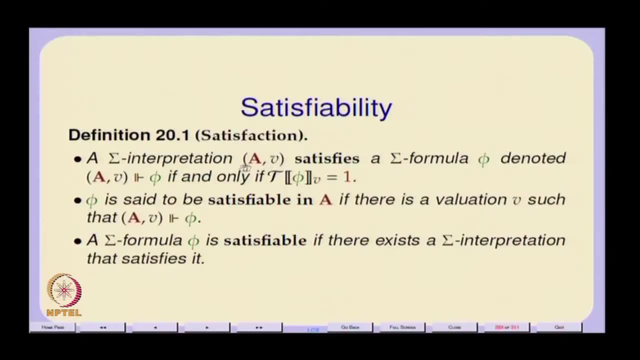 of first order logic. we are looking at a sigma structure And a language of first order logic for the signature sigma. so and then you have the notion of a sigma interpretation, which means you have a valuation for the variables along with the sigma structure and under that valuation you say that this structure a with the valuation. 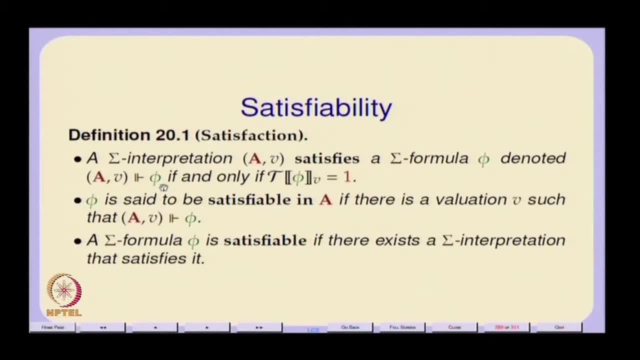 v is. that is an interpretation. this interpretation satisfies a formula phi if, and only if, the truth value of this formula phi under that valuation v is 1.. So phi is said to be satisfiable in a if there is a valuation v which will make it through. 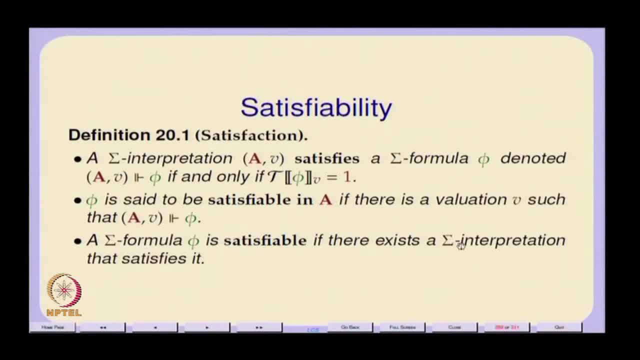 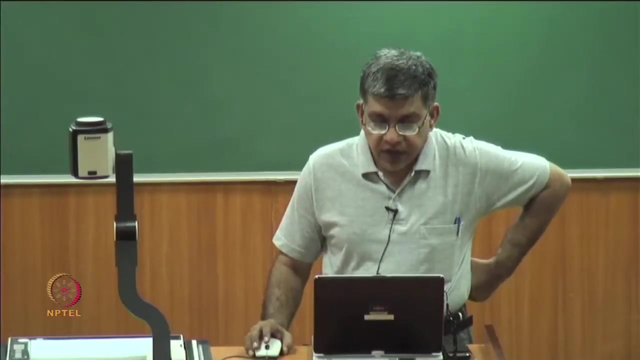 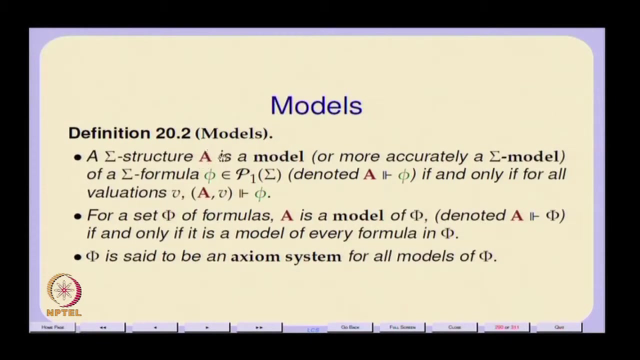 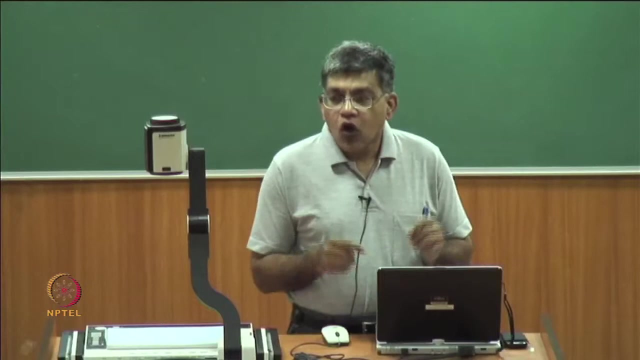 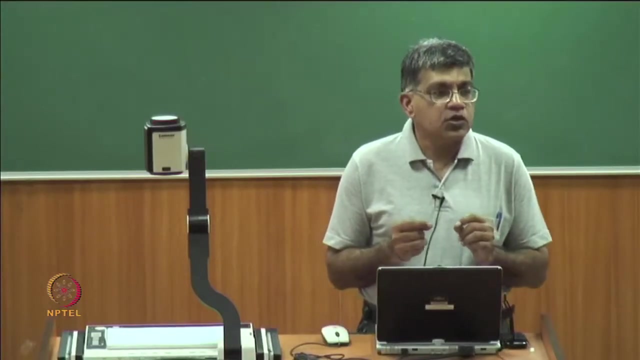 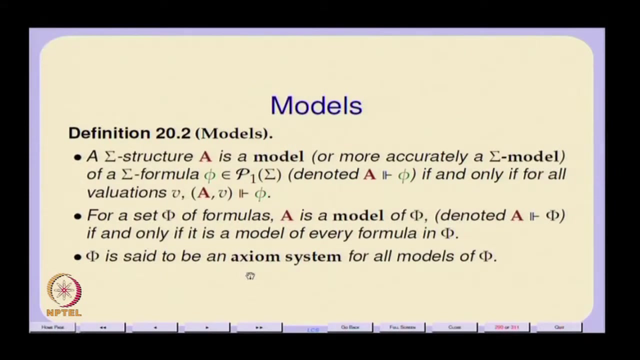 and a formula is satisfiable if there a sigma formula is satisfiable if there exists a sigma interpretation that satisfies it. so, which means a sigma structure a and a valuation v which satisfies it. So that is so. that is so. the notion of a model is then identified with the notion of 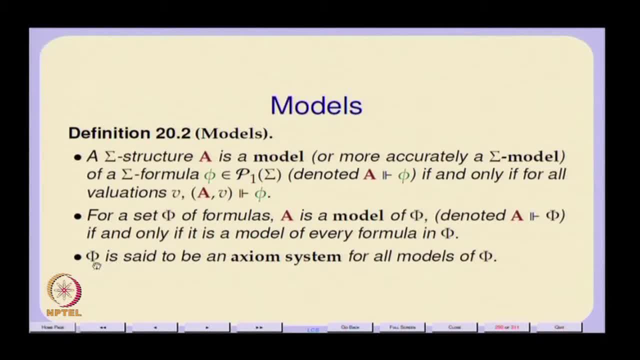 an axiomatic system. so what you are essentially saying, therefore, is that if I can find some models for a set of formulae, phi, then I can think of this phi as essentially defining an axiom system for all those models and which actually is close to what happens in the way. 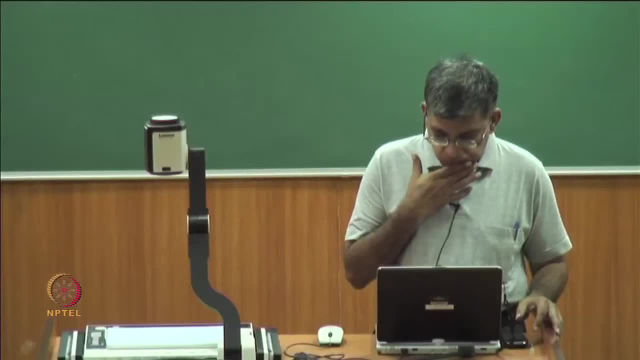 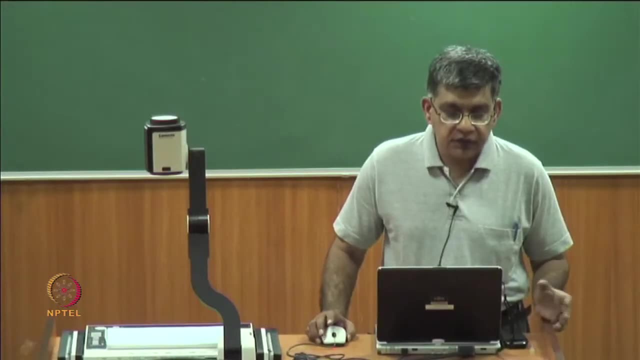 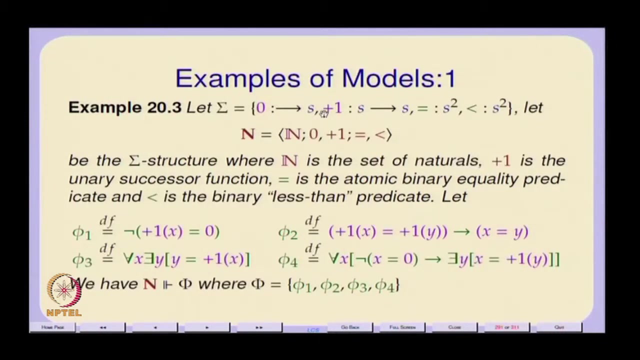 we describe most mathematical theories. So here let us take this is actually an elementary subset of piano arithmetic. basically, you have this set of natural numbers generated from 0 by a successor operation. so here is our sigma, here is our sigma, here is our signature sigma. and then, so, in addition to these two, 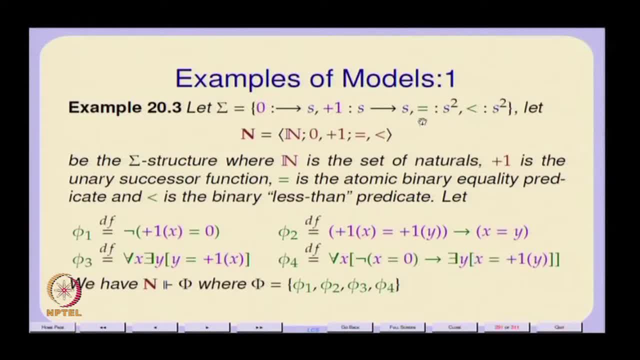 operations. 1 is the equality relation and the other is a less than relation. so far, exactly this is in some sense elementary form of the of piano arithmetic. 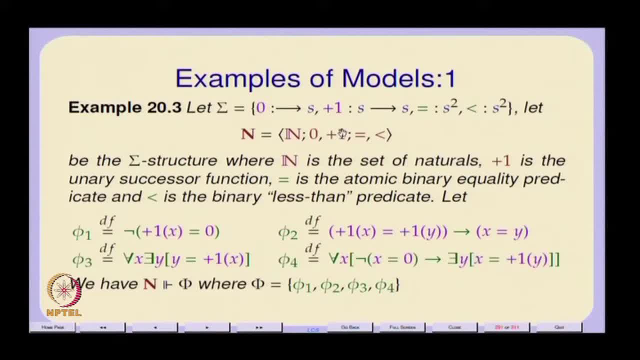 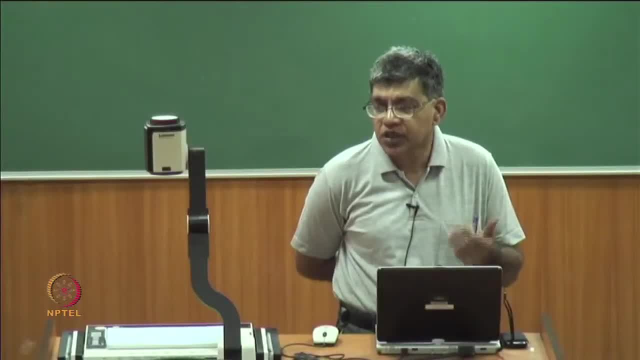 But we will. we will look at the piano arithmetic in greater detail later, the full axiom systems. so the notion of first order number as a first order theory of fine arithmetic is something we will look at later here. So let us take the sigma structure and let us take 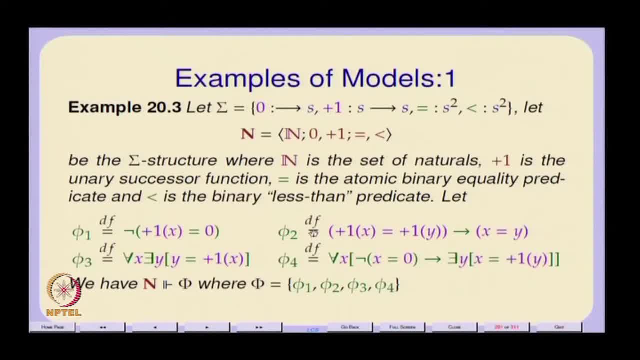 the natural numbers under these operations and these relations. then you have these various formulae. right, Here is this formula which says that essentially 0 is not the successor of any element. So this first formula, phi 1, should essentially be read as the successor. 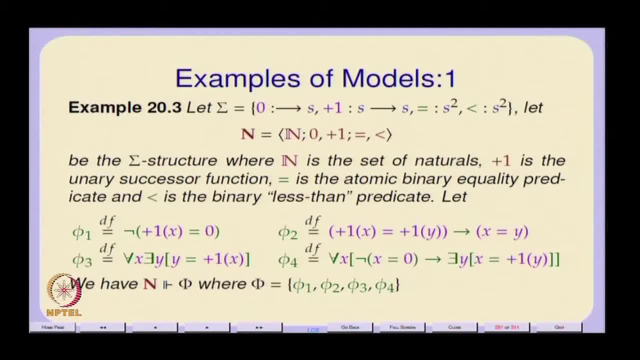 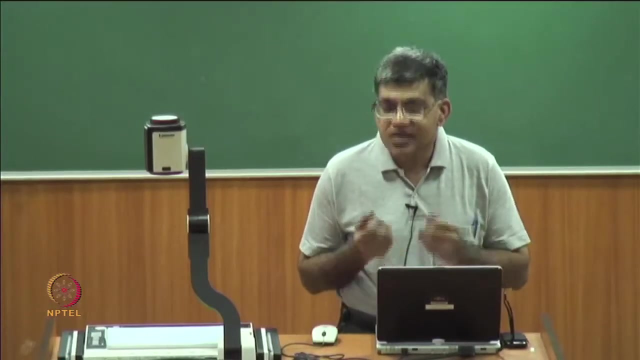 of x cannot be equal to 0 and of course we have x is a free variable here. remember that. but So this is a, so we will just keep that in mind. we will come to that what to do with free variables later. So this essentially says: if I have a pattern like successor of 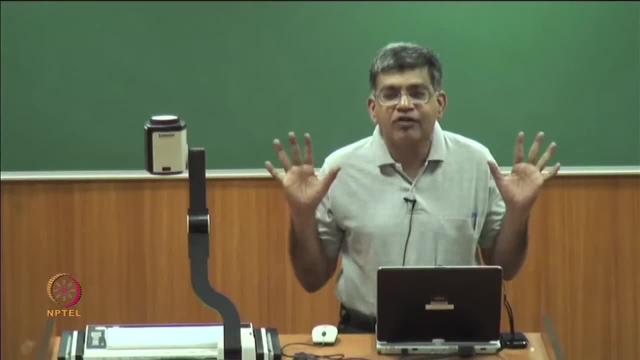 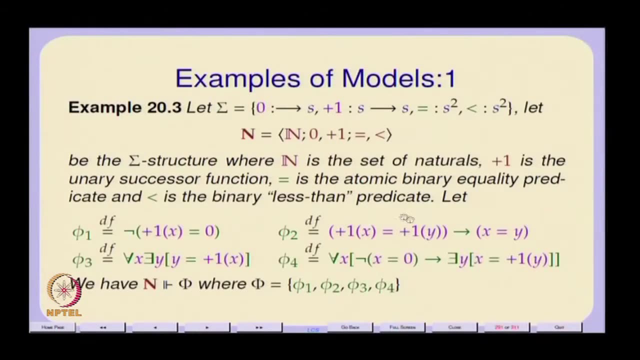 anything, it does not matter, then that value cannot be equal to 0.. Here we have that. here we have one of the one of Peano's axioms. actually, if the successor of x is equal to the successor of y, then x must be equal to y. Here is some, here is a. 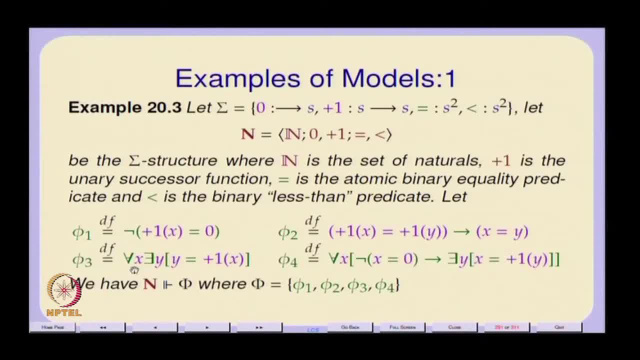 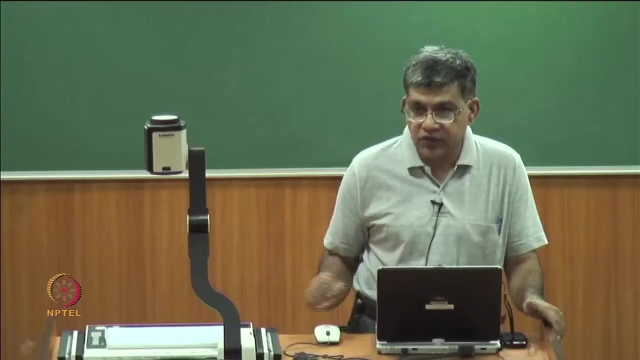 trivial statement: for every x, there is a y, which is its successor. you can, you can sharpen this statement, make it more accurate, like saying that there exists a unique y, but unique y essentially means I will be adding another conjunct which says: for all z, such that z is equal to plus 1 x, x, y is equal to z. That is how one would define uniqueness. 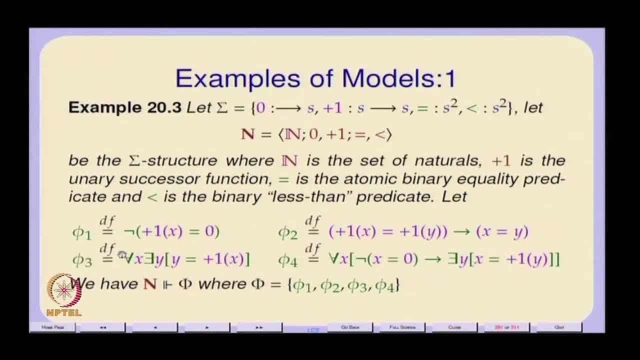 right, But anyway, let us. this is the simple example of a model, and here is a. here is something which says So: if x is not 0, then it must be the successor of some y. So these are the formulations of this. So what is now intuitively clear- though at the moment we do not have a proof- 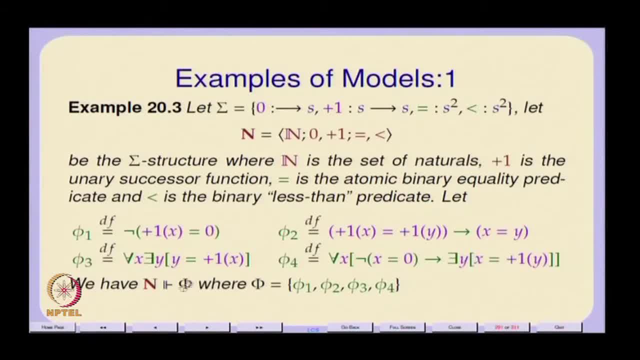 system. So we cannot actually prove it. but what is intuitively clear is that this structure n satisfies these four formulae, phi 1 to phi 4.. So n is therefore a model of this formulae. notice that some of these formulae have free variables. some of these formulae do not have. 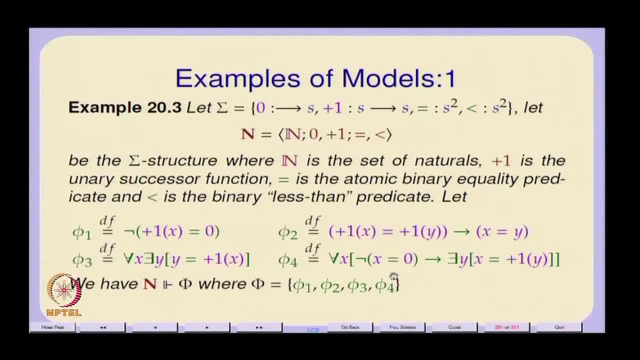 free variables. So phi 3 and phi 4 do not have any free variables, So they universally quantified, whereas phi 1 and phi 2 have free variables. and yet somehow the truth of phi 1 and phi 2 is independent of those free variables, is independent of any valuation. 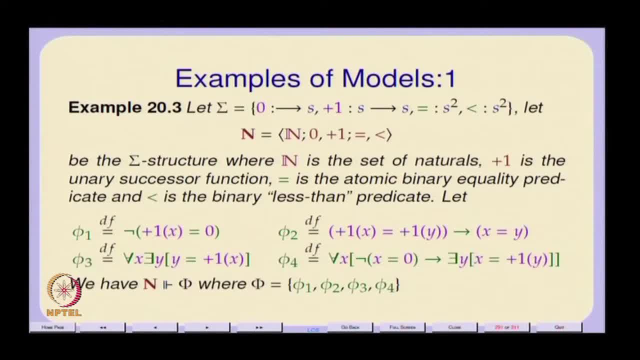 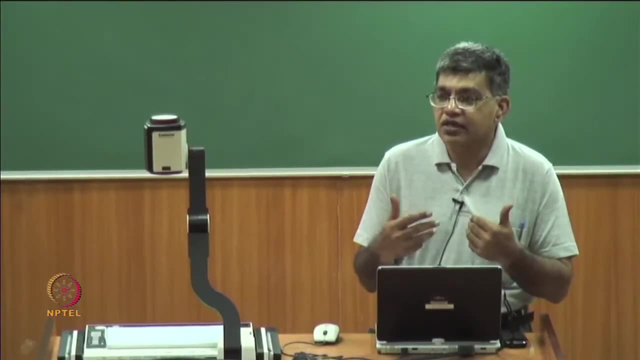 for those free variables. that is important to realize. In fact, that is the key to what most mathematics texts do. they do not actually explicitly give you, put your put a quantifier anywhere in their axioms. they just state the axioms with free variables And it is assumed that they are universally quantified and that 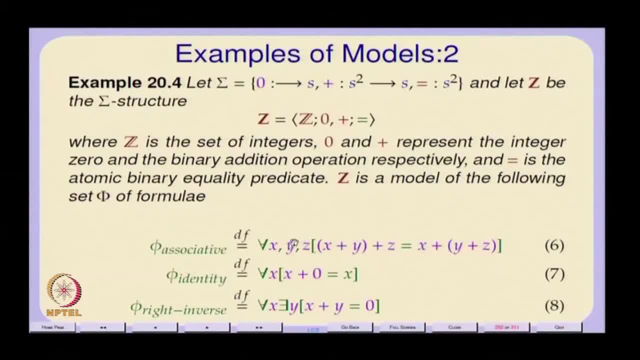 is something that needs to be justified and that can be very easily justified. but let us look at some other examples. So here is an, here is the set of integers, again with 0 and addition. so you have. so I, just so I can actually take any set of operations and any set of relations. 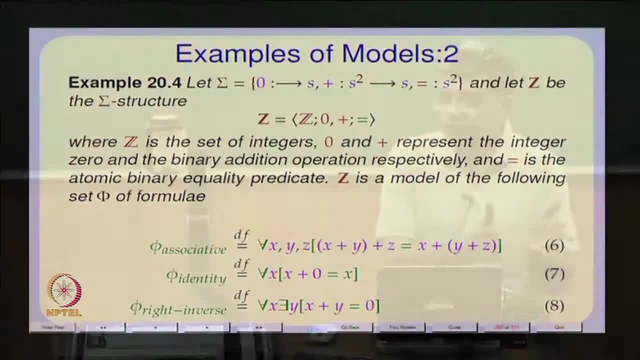 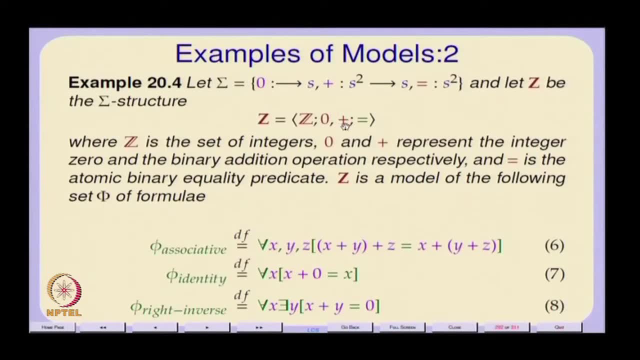 that I am interested in and form a structure, provided I have defined the carrier set in some way. So this z I have taken the set of all integers And I am interested especially in 0 and addition, and this equality is something that 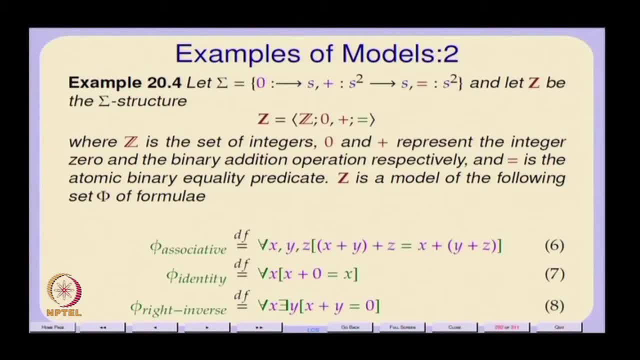 keeps on coming, it will keep on coming up, So that is often a very basic binary predicate that we have to use. in fact, what we will very soon see is that what we require really is not just a first order logic, but a first order logic with equality as a basic predicate, which 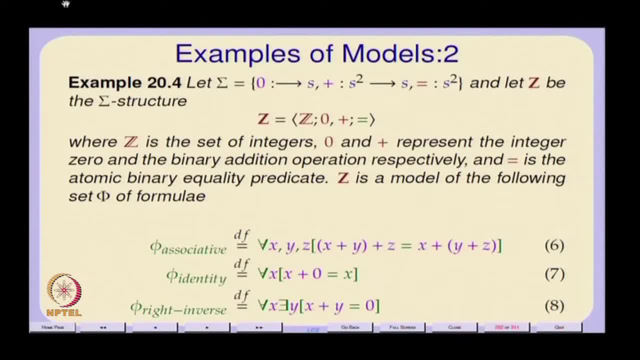 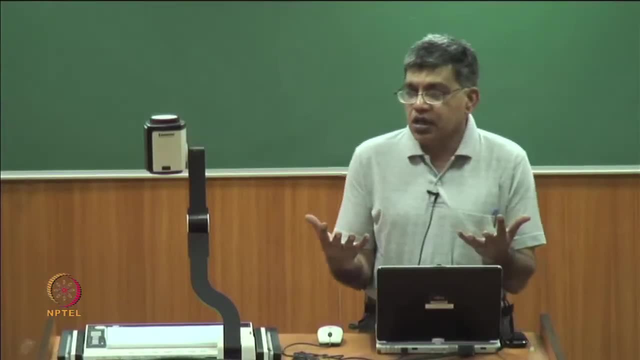 should always be there. So basically, essentially, what the reason for that becomes clear. because in any algebraic system equality is a basic predicate and without equality it is very difficult to do any kind of manipulation. For example, two different syntactical expressions are not really equal. 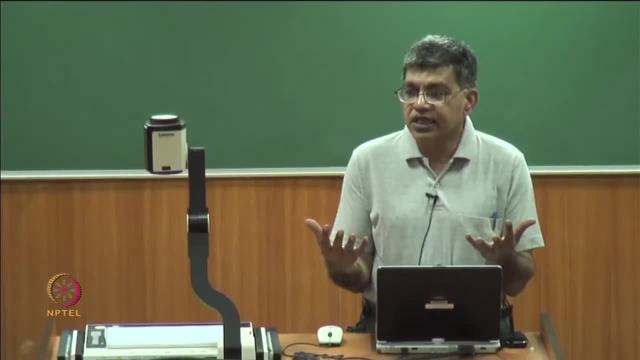 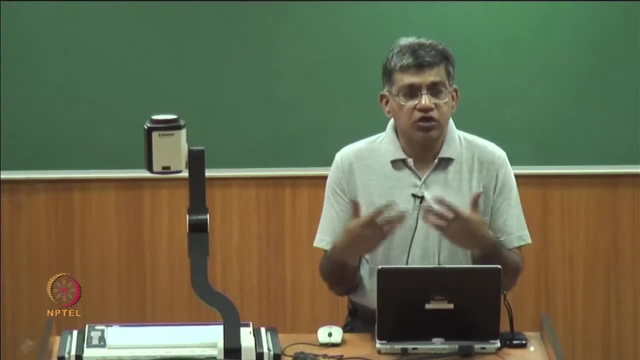 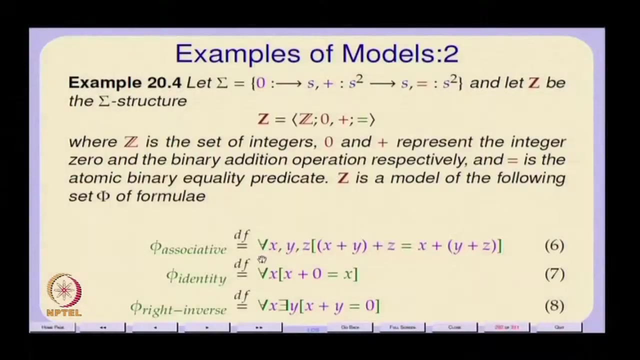 syntactically, but it is quite possible that they are equal in terms of values, when you think of the under all valuations, for example. So the notion of equality is something that is far more basic and we will need. we will require that. So, but before we get on to first order logic with equality, let us first 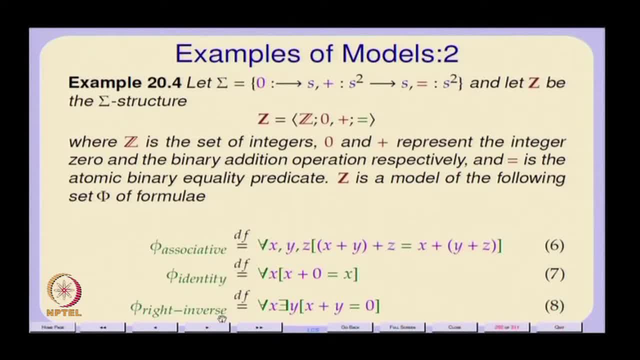 look at this. So I have essentially these are some group axioms. So phi associativity basically just says for all x, y and z. I think I said somewhere that. So this is a short form for all x, for all y, for all z, and I will use a single pair of. 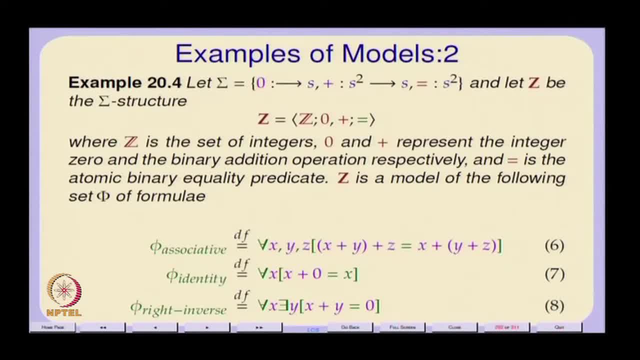 brackets, so that I do not clutter up the notation with too many brackets. So then, this is just the associativity law. now here, in this particular case, I have, of course, universally quantified it on all the free variable, on all the variables that I use in the body. 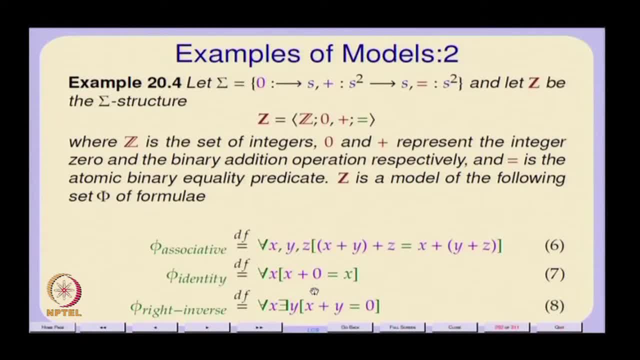 The identity. it should be more correctly called the right identity, but let us call it the identity. So x plus 0 equals x. and then there is a right inverse: for all x there exists a y, such that x plus y equals 0. So y is a right inverse of x and that is important. So this: 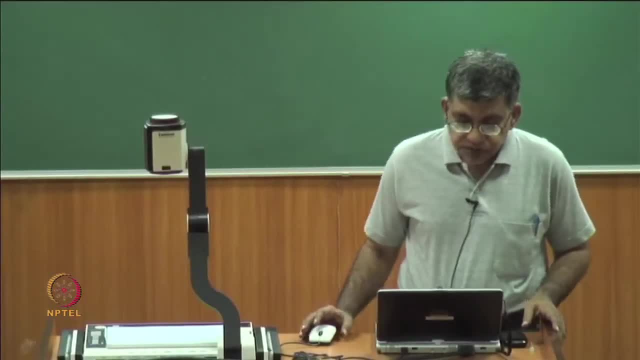 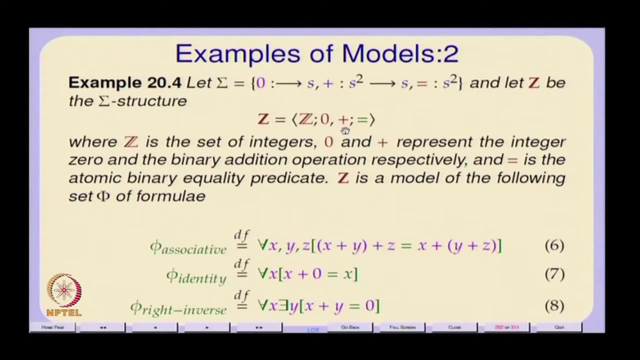 does not say anything about uniqueness and so on. So, if you take this set of integers under 0 and plus, So this is a structure, that is a model. it is a model of these three axioms. So that is essentially so. that is an example. Now, of course, when you are talking about group, 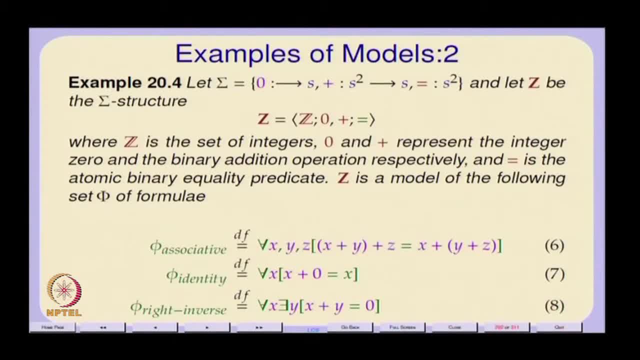 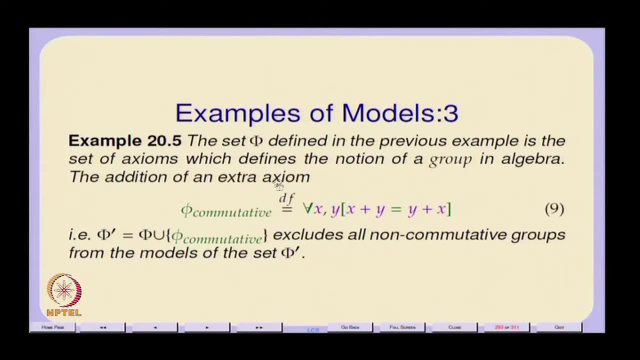 theory itself. you might not be interested in the particular structures, but you might be interested in general properties of groups. Now here is- here is another example where I add in you axiom called the commutative axiom, which is for all x and y. x plus y equals y plus x. 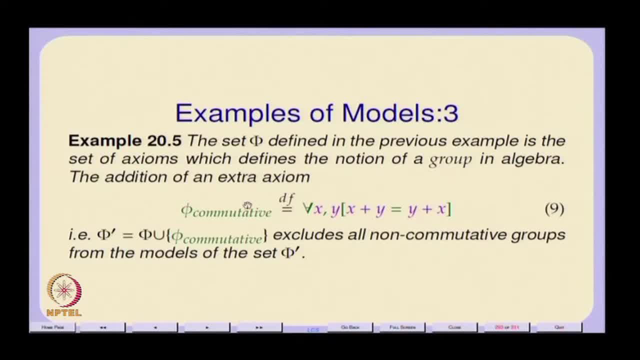 So now, if you look at phi prime- So phi, let us say, contained all these three formulae and phi prime contains everything in phi and also the commutativity- then what you are saying is that: 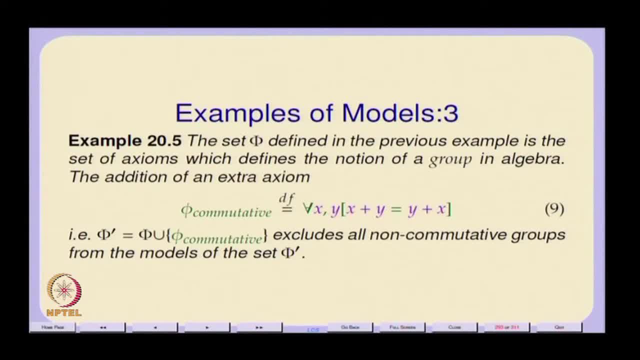 the has as models only all commutative groups, all abelian groups, and there the non abelian groups are excluded from it, Whereas phi includes both commutative and non commutative groups and as models- and of course we have this notion- 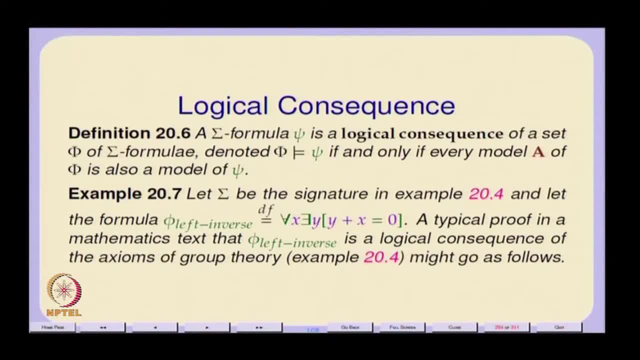 of logical consequence, as we did before. a sigma formula of psi is a logical consequence of a set phi of sigma formulae denoted. phi proves psi is a logical consequence of phi if, and only if, every model a of phi is also a model of psi. So now the notion of logical consequence has 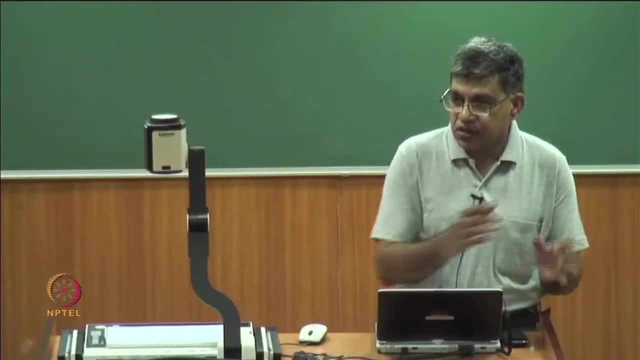 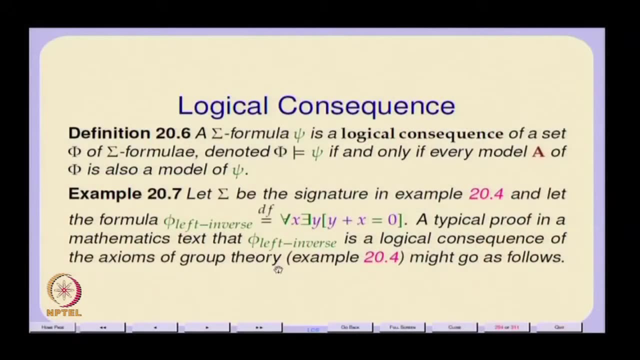 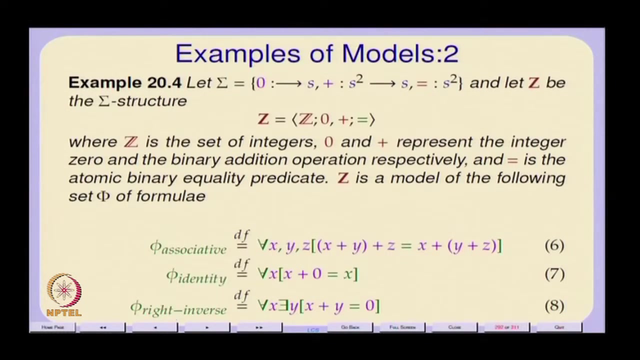 been imported straight from propositional logic, as you can see. So one question is that we had this notion of right inverses and, without worrying about an individual model of these axioms, I might want to show, I might want to prove theorems. 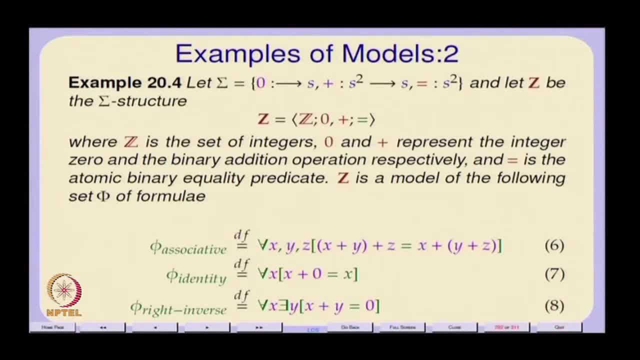 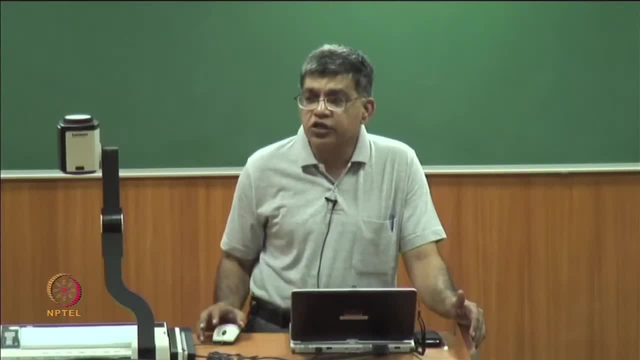 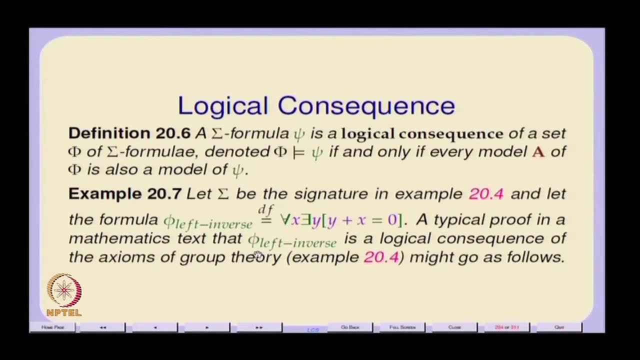 that are true for all models of these axioms. That is the way we work polymorphically in most of the mathematics and computer science, and So one possible logical consequence that you might want to prove is that every that right that there are left inverses also, So this: 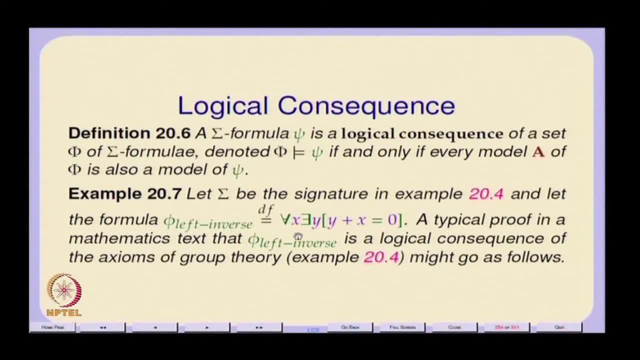 formula phi left inverse essentially says that every element x has a left inverse y, So that y plus x is 0. So The fact that it is a left inverse, that there is such left inverse usually can, is proven. 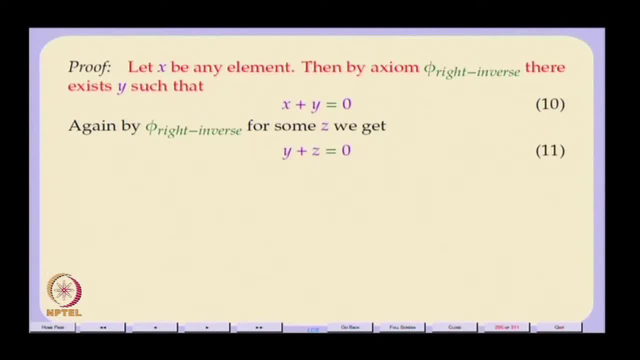 in any mathematics text. by assuming let x be some element, then by the axiom, the right inverse axiom, we get that there is a y such that, which is that x plus y is 0, and again, given that there is a y, again by the right inverse axiom. you know that there. 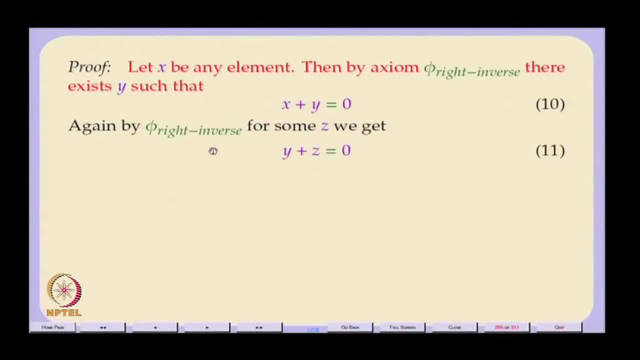 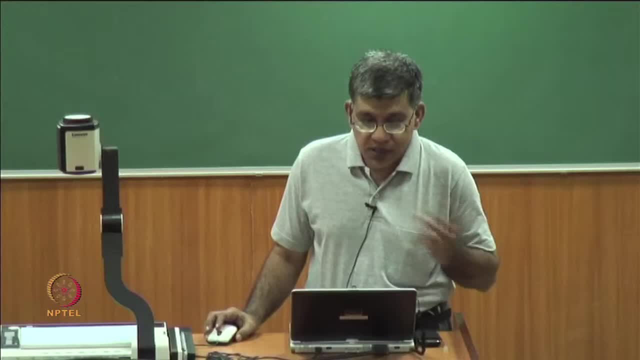 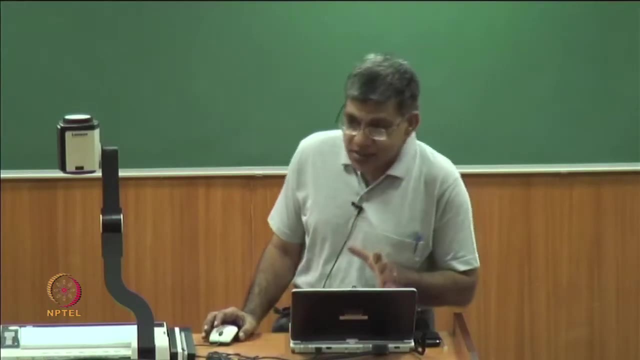 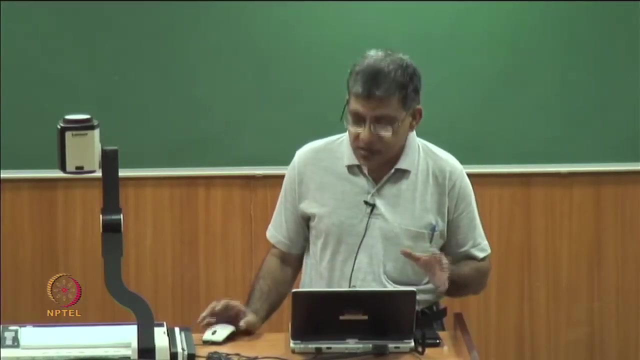 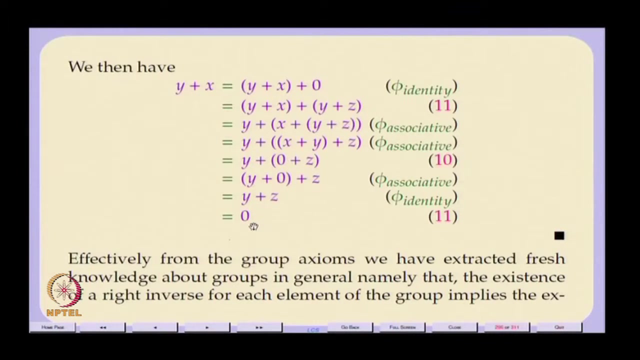 is some z. assume that x is you only know about right inverse is So you have to, so y must be having a right inverse. I do not know what it is, but it is some z. So with these assumptions, essentially what you can show is that y plus x gives you 0 and in all these cases, what we have used, 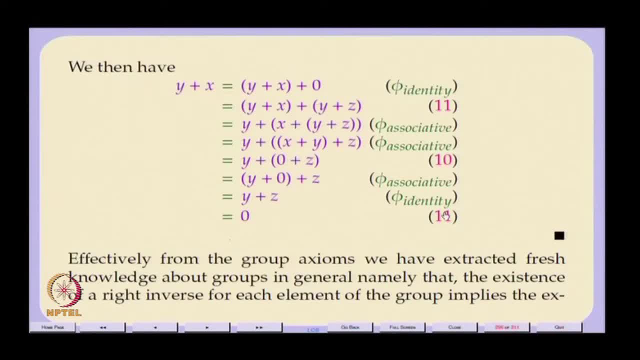 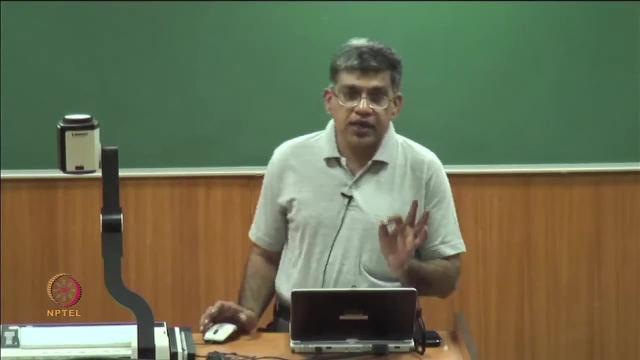 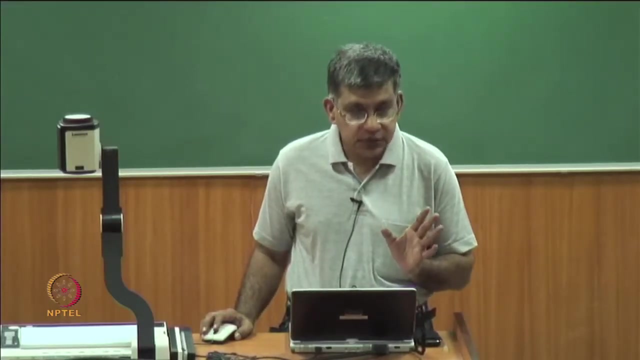 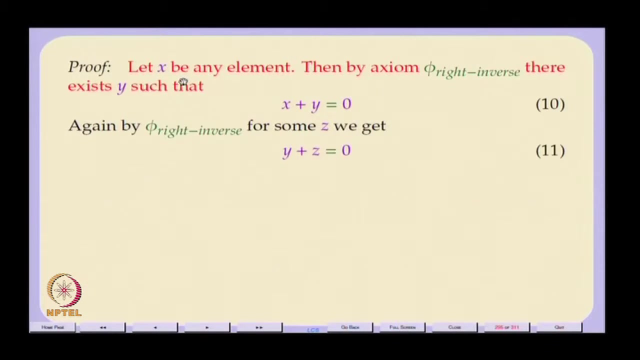 are only these, the group axioms, or these two which have been marked 10 and 11 throughout this. So essentially so, y plus x is 0. so what you are essentially saying is that y is a left inverse of x. So your left inverse formula actually is sort of proved by this proof. but this proof 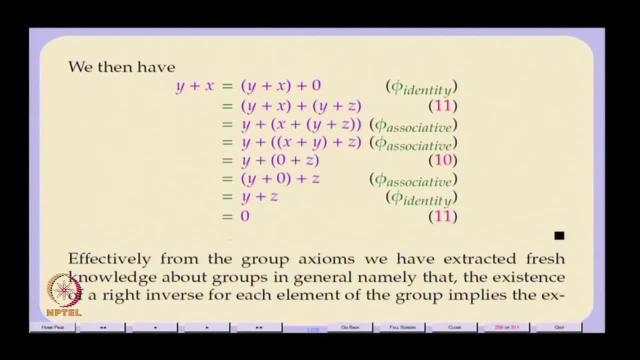 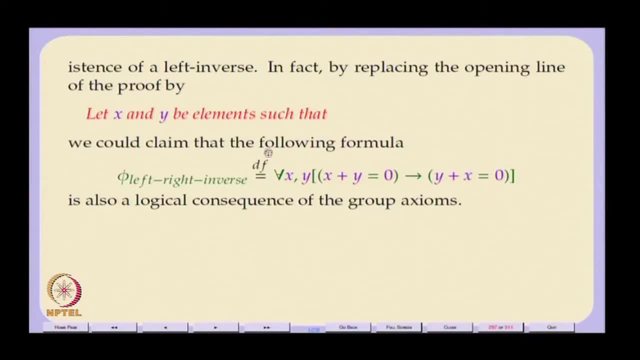 actually is fairly general, in the sense that I can claim that every right inverse is also a left inverse, And the proof for that is between x is. so you take formula left, right inverse, which essentially says that every right inverse is also a left inverse. that is the. 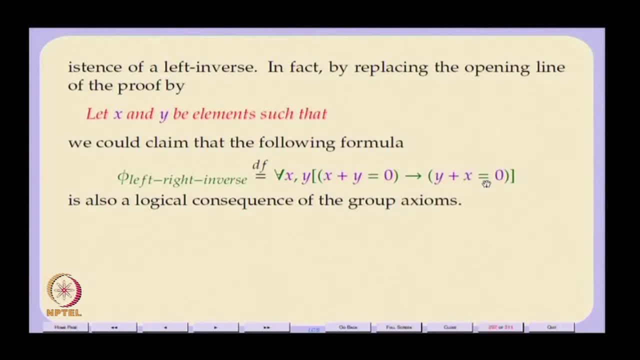 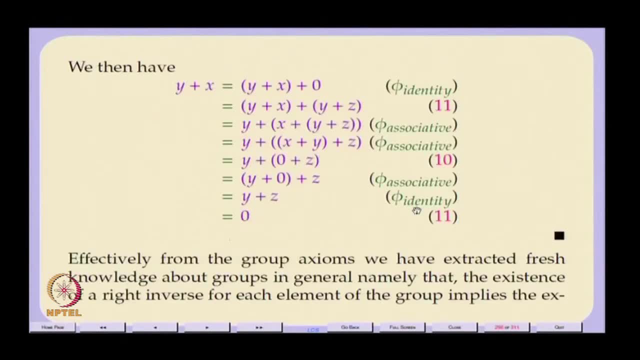 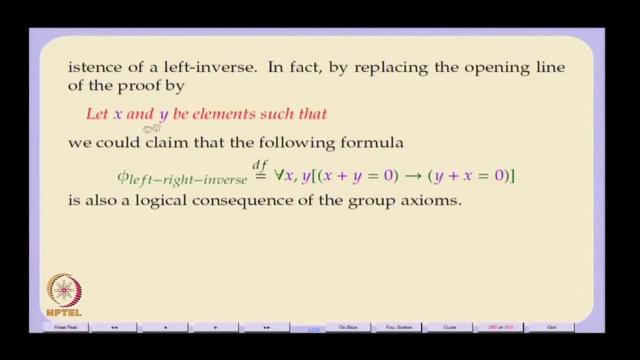 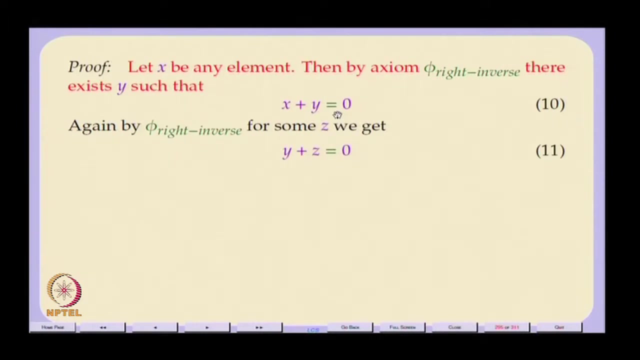 formula for all xy: if x plus y is 0, then y plus x is 0.. So this can also be used the same proof, except that this part and red has to be replaced by something like: let x and y be elements, that x plus y equals 0.. Then by, since there is a right inverse for every element there. 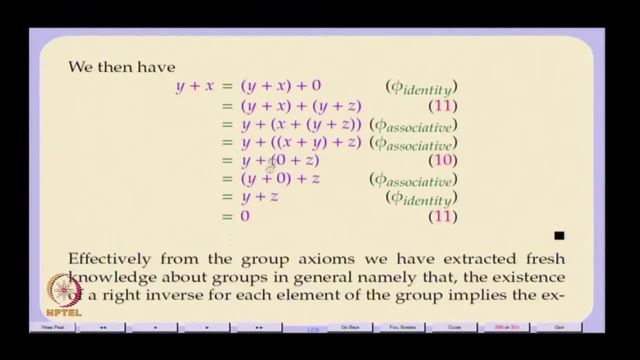 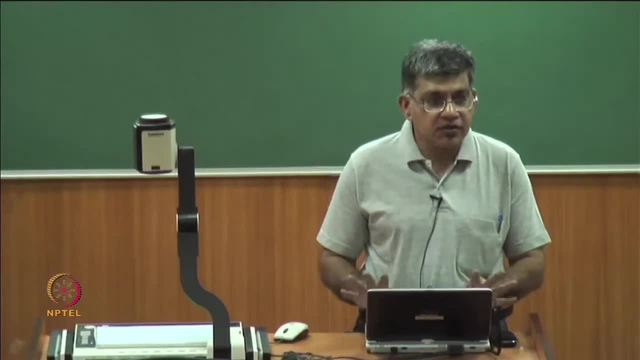 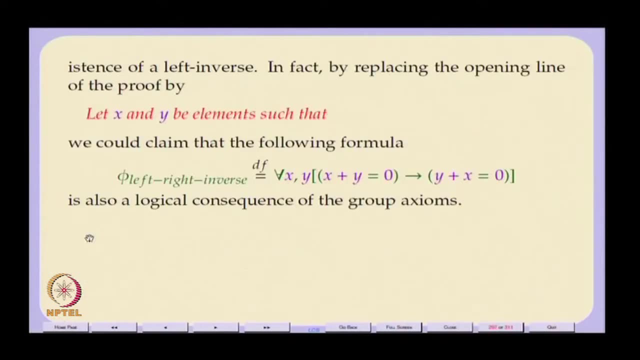 is some z, such that y plus z equals 0.. And then this whole proof goes through and essentially shows that y is left inverse of x. So this is how standard proofs go in mathematics, and often what happens is that essentially the same proofs can hold for sharper statements. 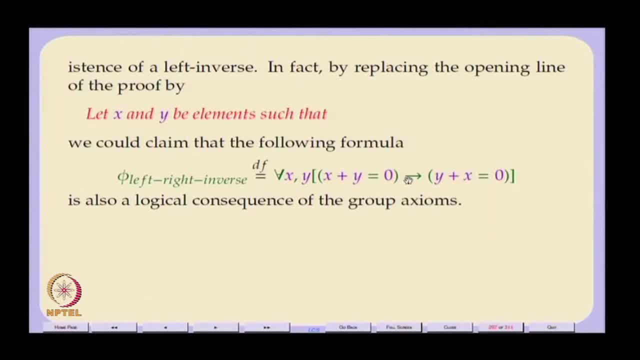 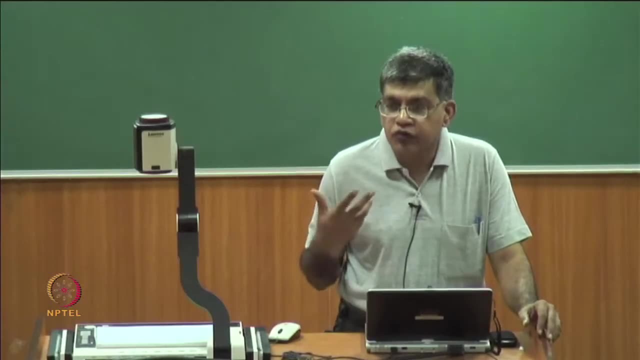 in a certain sense, this is a more. this is a sharper statement than the statement that just says that there exist left inverses. Here it says that every right inverse is also a left inverse and given that every element has a right inverse, you know how to find the. 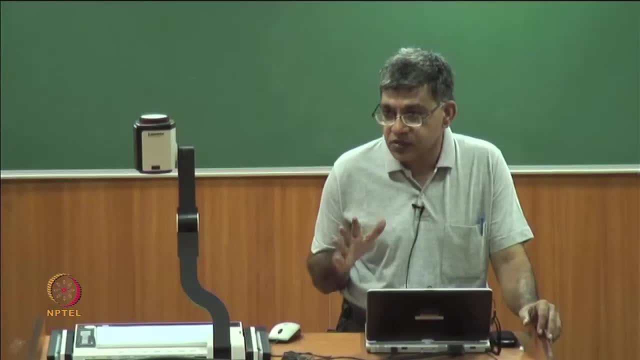 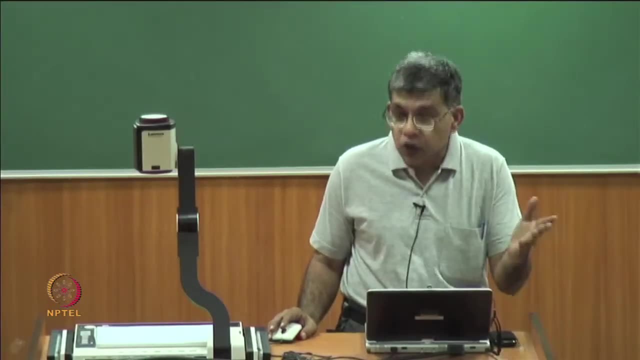 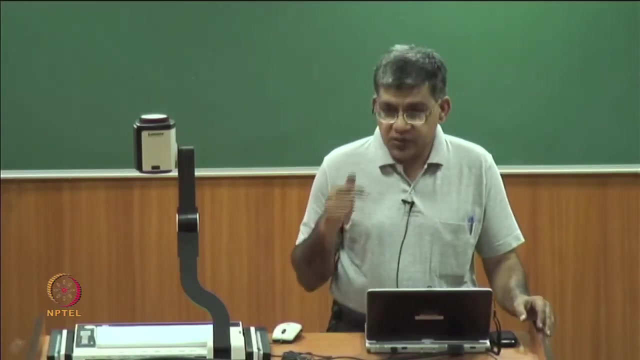 left inverse, because the same element is also a left inverse. So it is, in a certain sense, a sharper statement, and this is also a logical consequence of the group axioms. So this is like a typical proof. So what we are really looking at is: 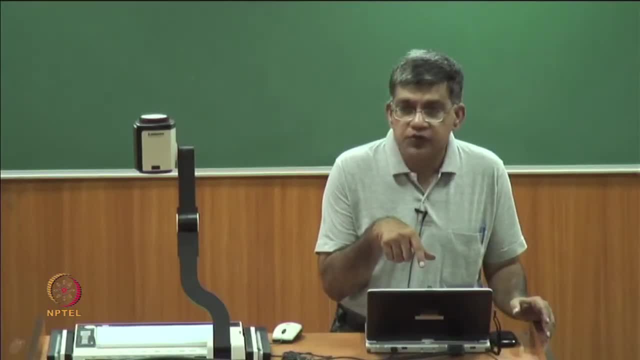 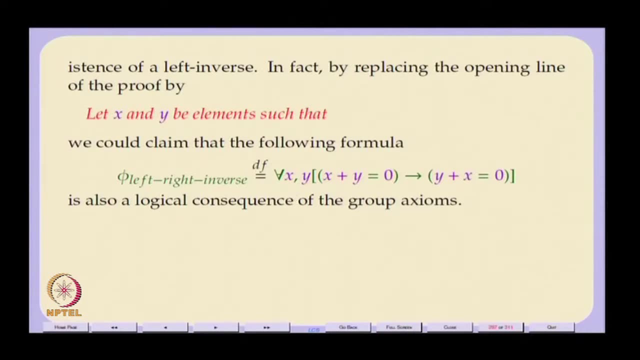 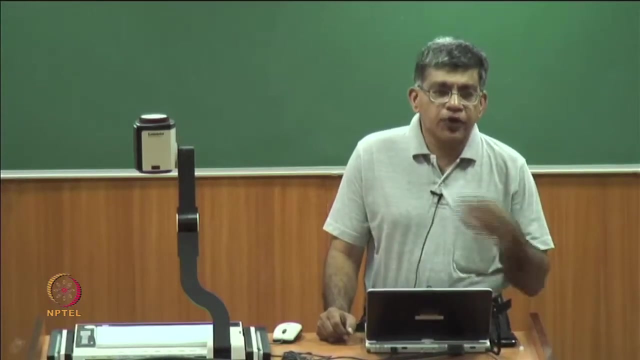 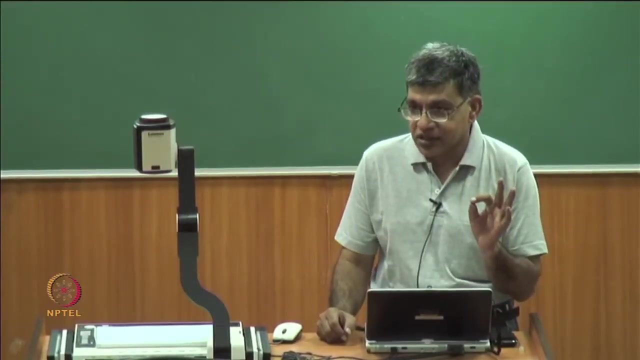 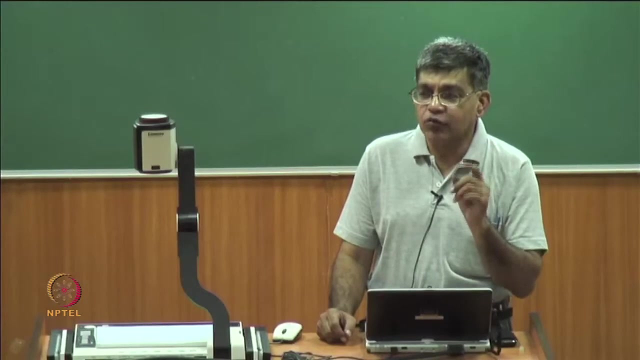 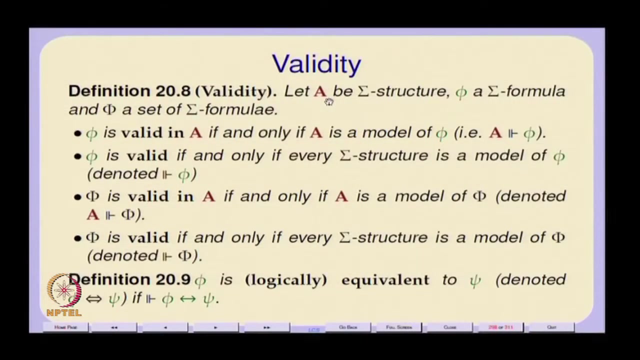 formalizing the notions of these proofs, of such proofs, within first order logic. So then there is this question of validity, Which, approximately, is like tautologousness in propositional logic, but not quite a. validity is a slightly more general notion. So let us take a to b, some sigma structure and phi. 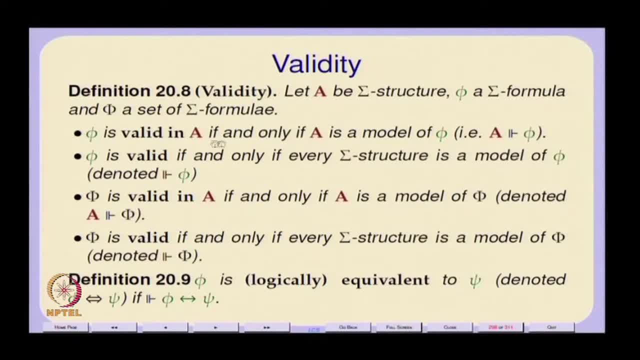 is some sigma formula, then we will say that phi is valid in a if, and only if, a is a model of phi. So that is one thing. So validity comes directly from the notion of a model. phi is valid. now, this is where something close to being a tautology comes in. phi is valid if. 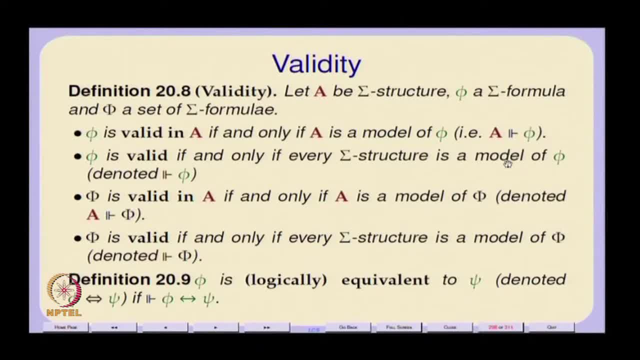 and only if every sigma structure is a model of phi. The reason it is goes beyond the notion of tautologousness is because this phi could have free variables in it for one thing. Secondly, all our language is parameterized on this signature sigma, So you are always talking about validity only in the context of a certain 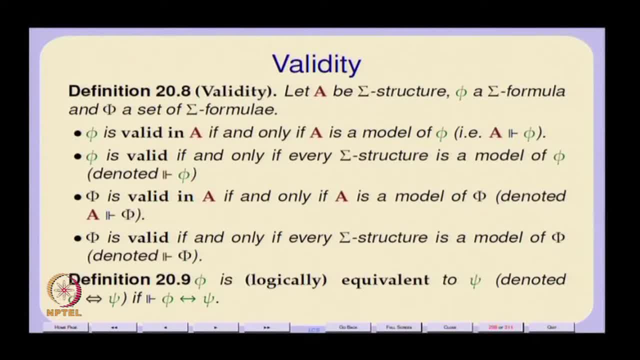 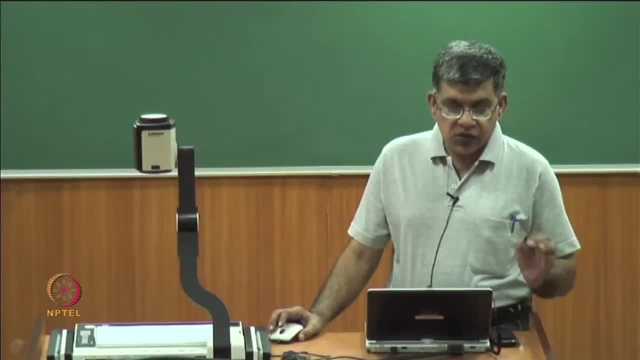 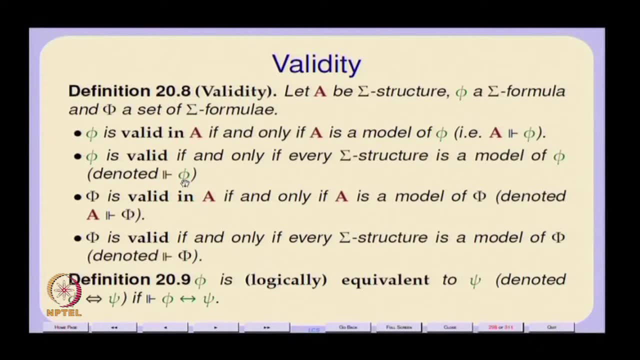 sigma. it is not. So in that sense it is the parameter. sigma is always present, right? So we would say So the notion of validity, and we will. ok, So actually it should be denoted this way. but most books in logic do not distinguish between this symbol and. 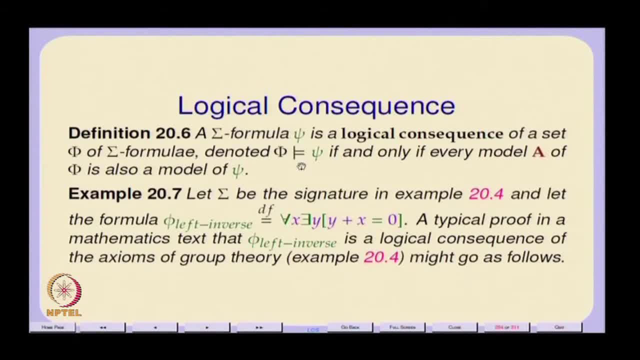 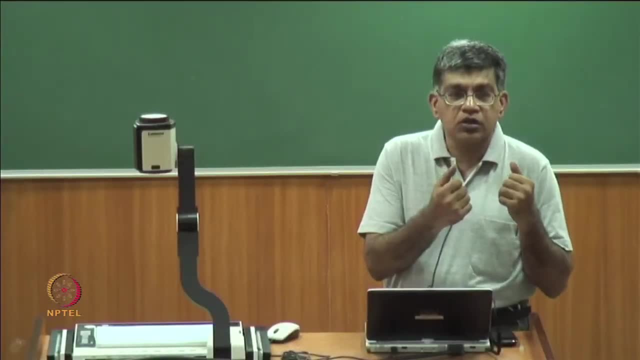 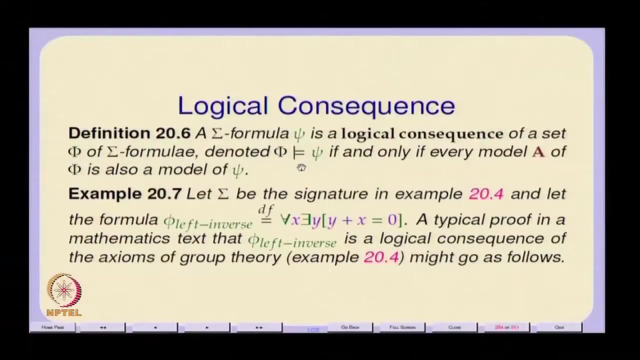 this symbol, But I have tried to distinguish it because in is 1 case you talking about models, truth in models. in another case you are talking about logic is only noise, So logical consequence from a set of formulae. So because of the fact that, notice that if 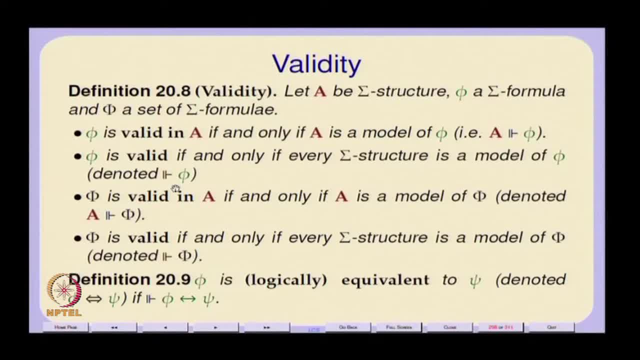 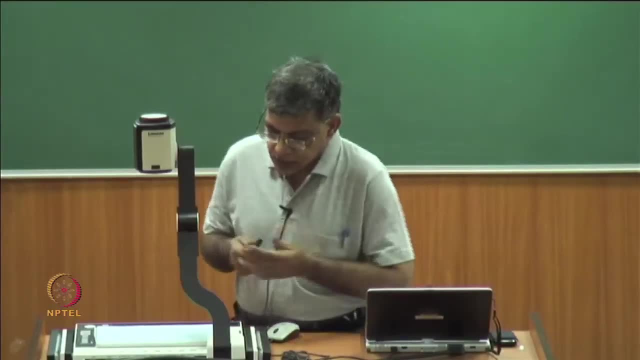 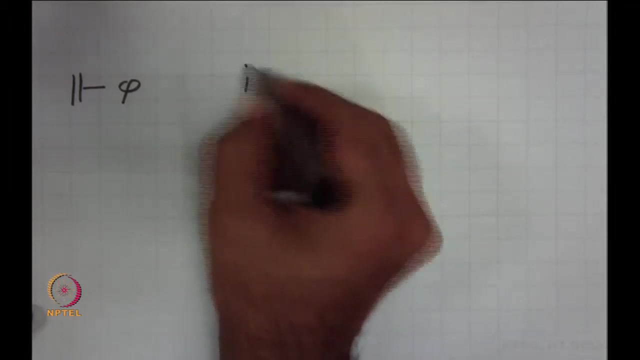 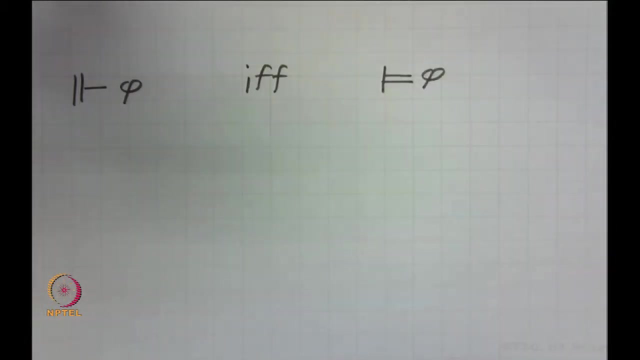 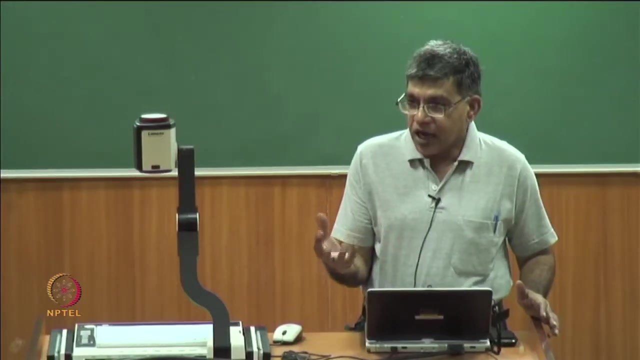 every sigma structure is a model of phi, then what you are essentially saying is that phi is also a logical consequence of the empty set of predicates. In that sense, this is the same as this and because validity is the same notion. So, anyway, you are parameterized on a signature sigma and you are saying: for every sigma, 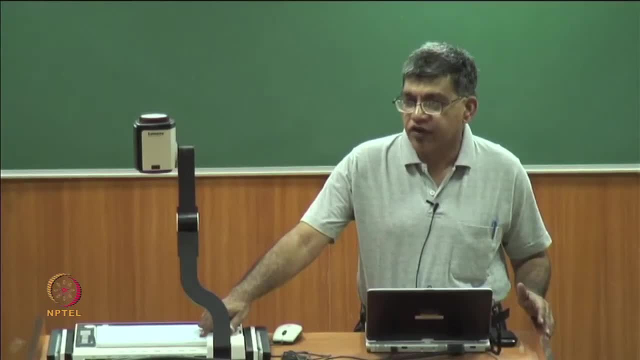 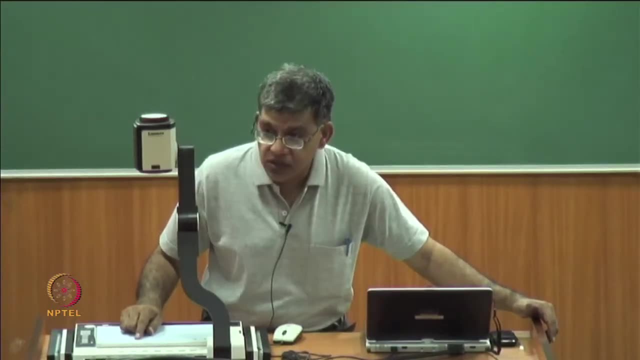 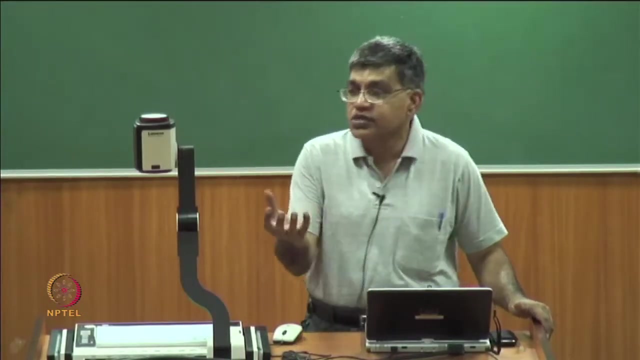 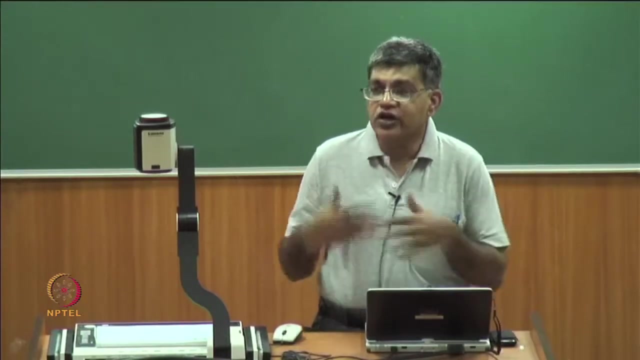 structure phi is. every sigma structure is a model of phi, which means that phi is true of every sigma structure regardless of valuations. So in a certain sense it is a logical consequence of no assumptions. So it is true for all sigma structures without any assumptions. and 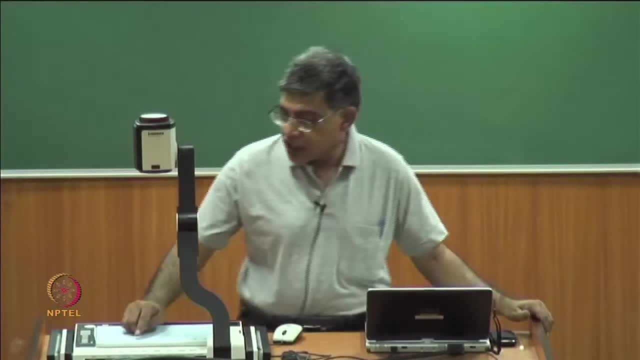 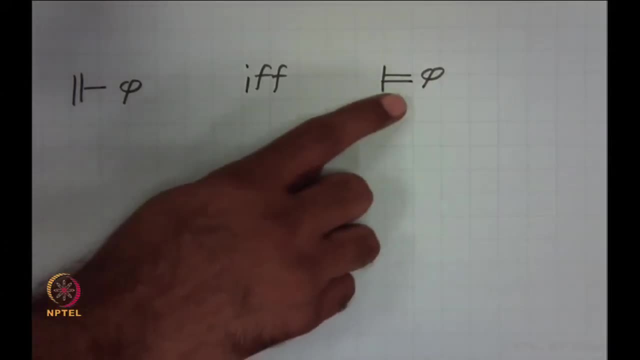 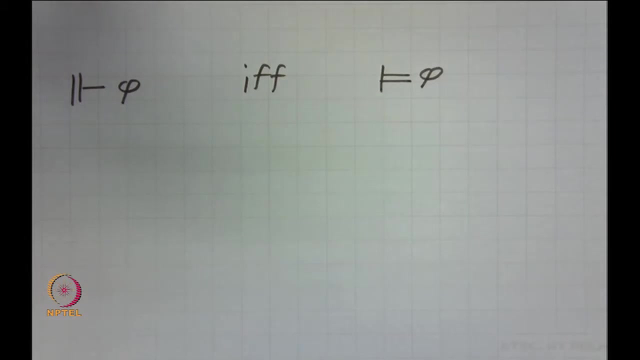 without an independent of valuation. So it is actually a logical consequence of an empty set of assumptions. So most books would actually use this symbol for validity. they would also use this for models, though the types on the left hand side are different in the case of. 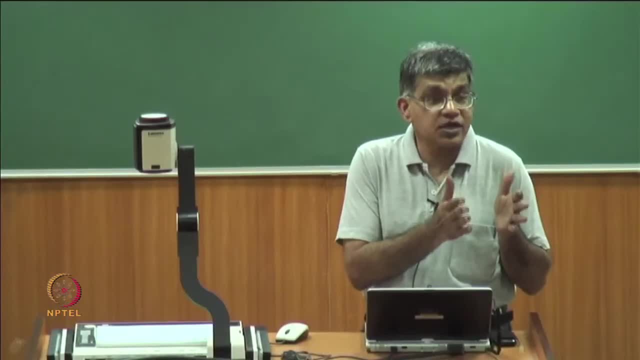 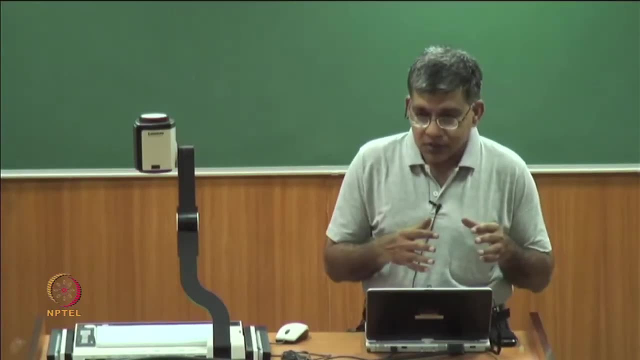 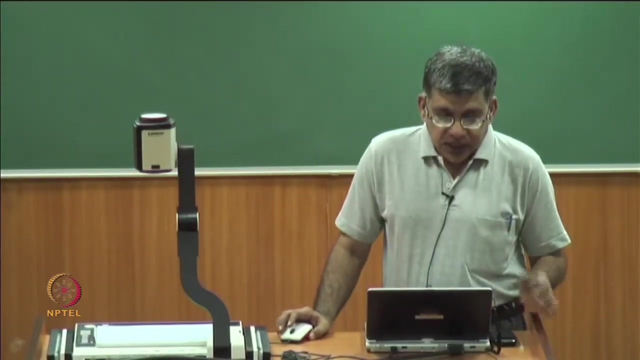 logical consequence. you are talking of the left hand side consisting of a set of formulae as assumptions, Whereas in the case of models, they are some other structures. I mean, there is a color difference right between green and brown, and that is the difference. yeah, So, but however, 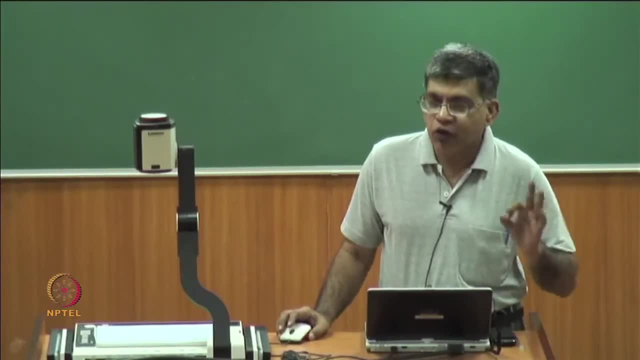 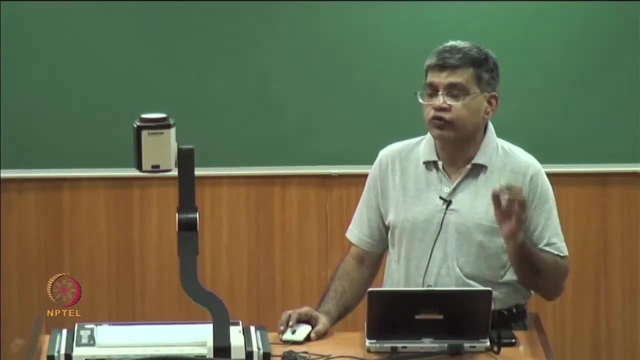 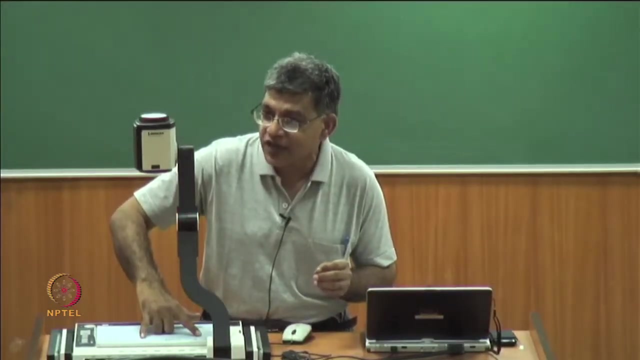 so you have to watch out for that confusion. but once you realize that they are using the same, they are overloading the same symbol for two different concepts. and they are overloading the same symbol for two different concepts precisely for this reason, Because the notion of validity in the two cases will coincide. therefore, you should not. 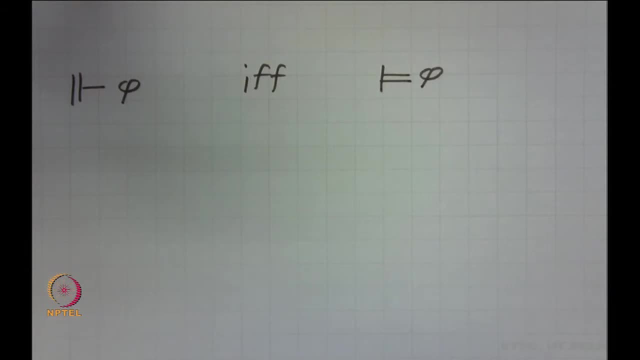 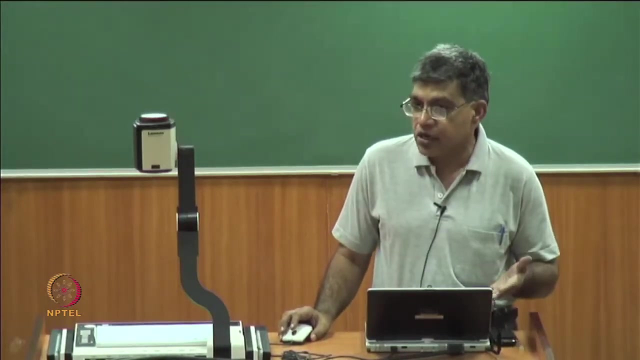 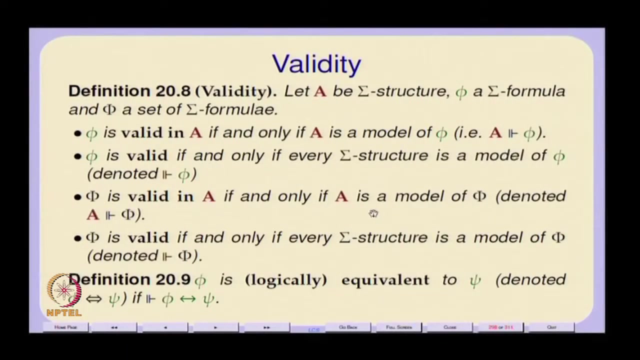 get confused by it. So now, what holds for a single formula is extended to sets of formulae. So we will say that capital phi, which is a set of formulae, is valid in A if, and only if, A is a model of all the formulae in phi. So 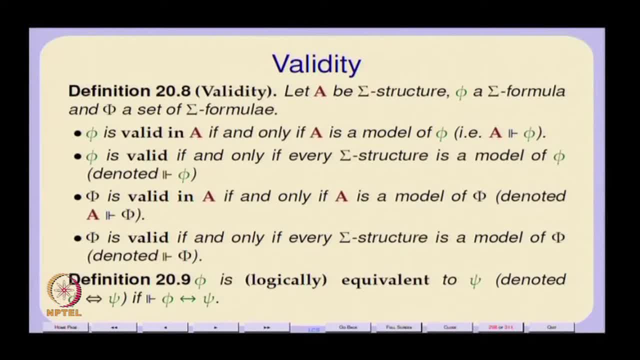 for example, all groups are models of the group axioms which we have seen before, right and all abelian groups are models of, are models of the group axioms, including the commutativity axiom. So, in that sense, all these statements of commutativity, associativity, right inverse, 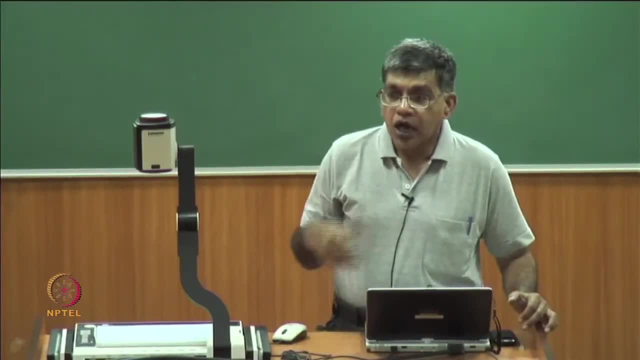 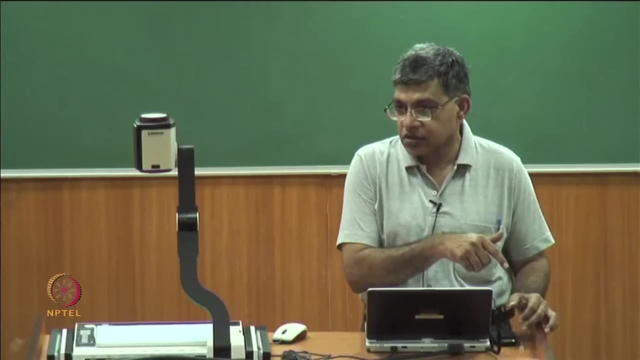 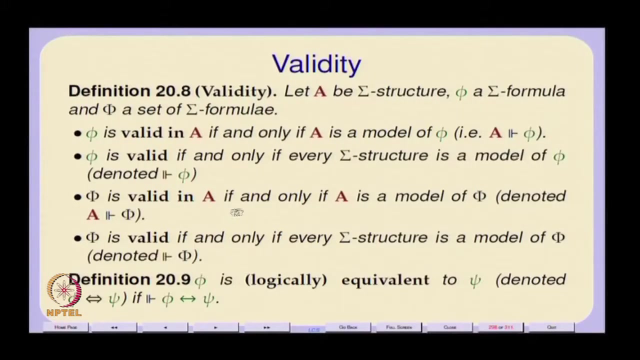 and identity are true in all those, in all structures with that signature. right. So they are valid in all structures with that signature and hence they are valid essentially in all groups, right? So the set phi is valid if, and only if, every sigma structure is a model of phi and this 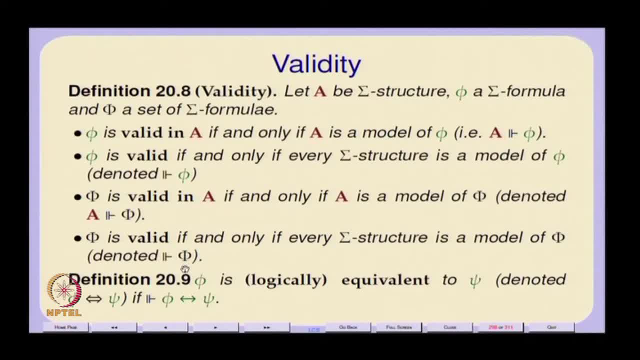 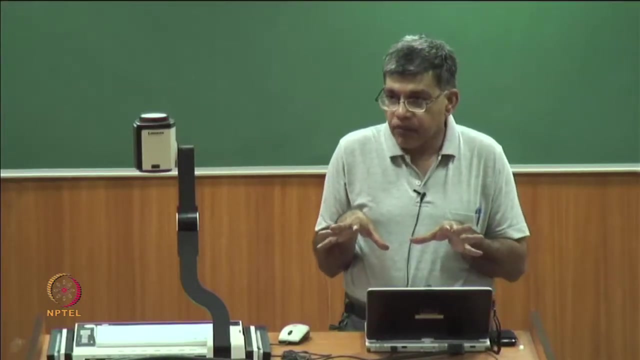 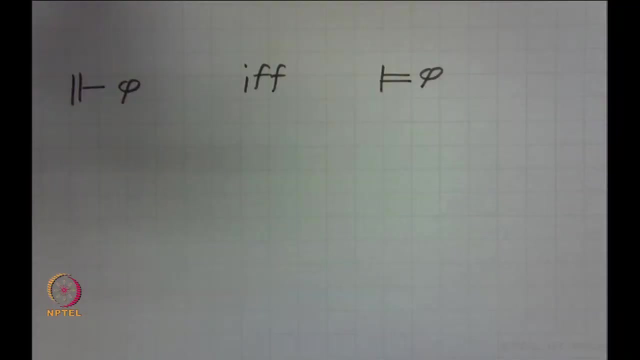 is the closest we come to having a set of tautologies. So this portion corresponds to phi, this lower case, phi being a tautology. So, in particular, you, if phi has the form, has the shape of a propositional tautology, right. so, for example, if phi has, even though 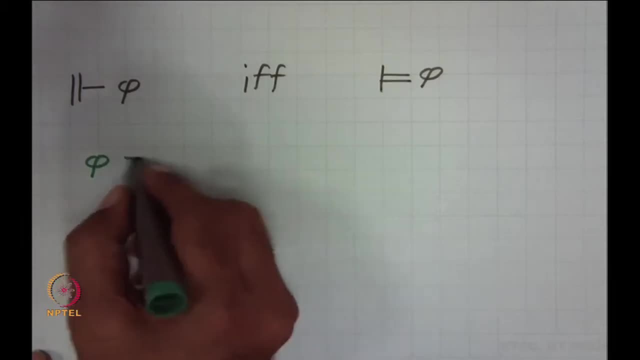 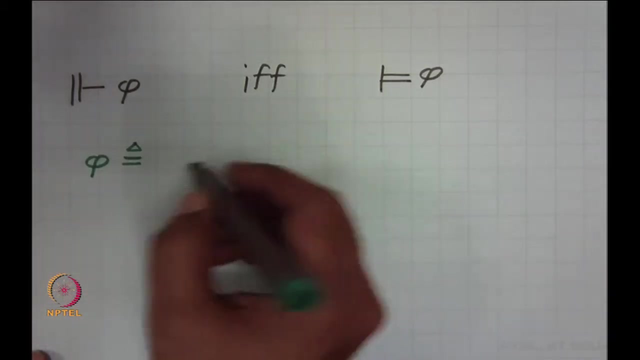 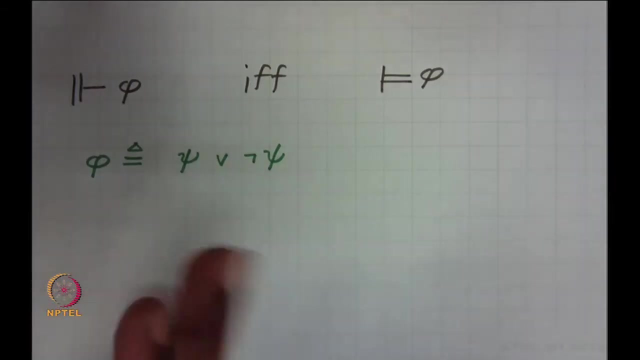 it might have free variables if phi has the same shape as a propositional tautology. and by the same shape I mean, let us say it is of the form, some psi, of phi or not psi. So this is a certain. now I am not really interested in what psi is, I am. 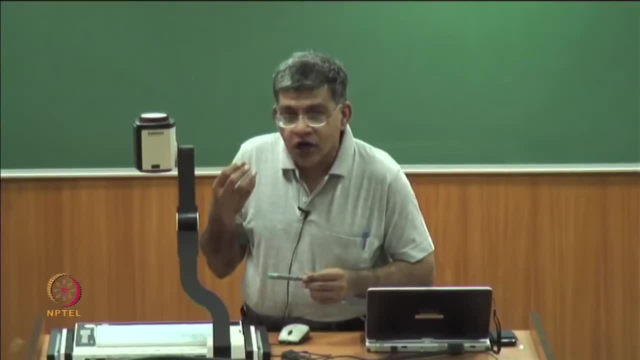 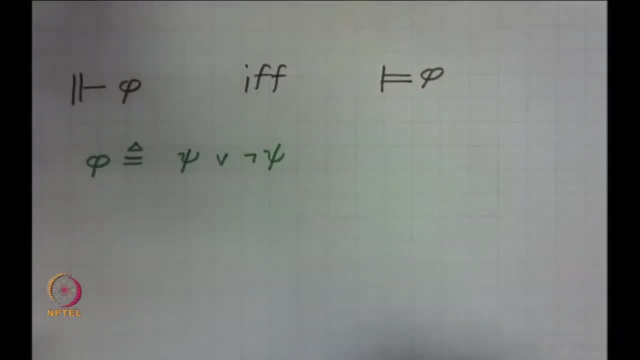 not interested in whether psi is got free variables or not. All I am saying is that the shape of this formula, viewed as a tree, for example, is essentially like this right, where psi itself might be some tree. all formulas of this shape are propositional tautologies And in first order logic they will all be valid. 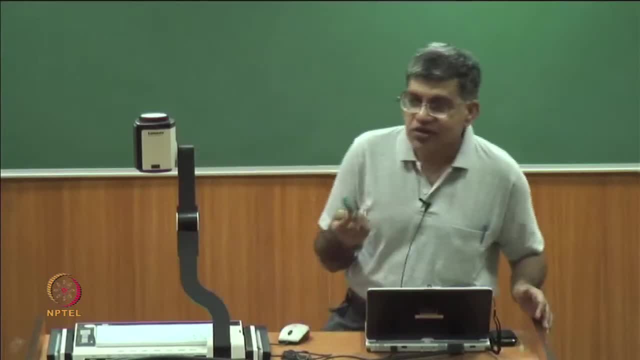 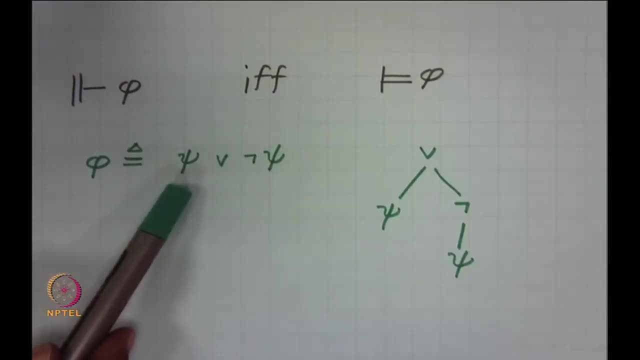 too, because it they, you take. the only restriction is that you have to somehow reconcile the terms, since there it might have free variables, it might have terms. you have to reconcile the terms with some signature sigma, But except for that, it they, all these formulae will also be valid, regardless of whether they 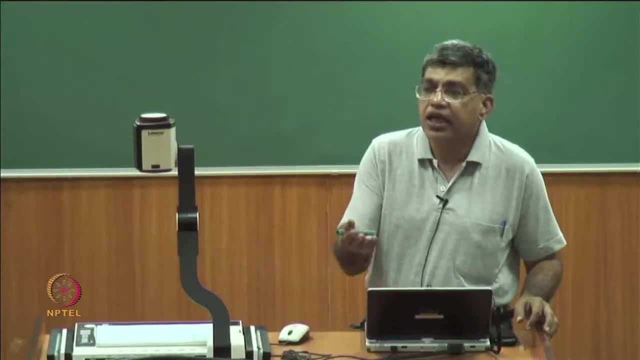 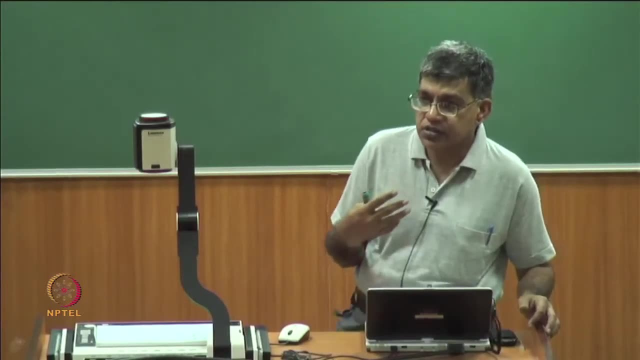 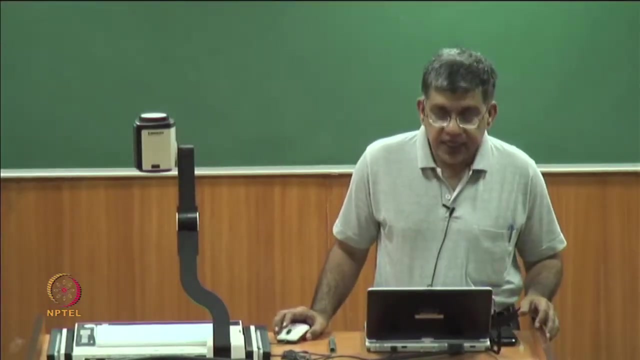 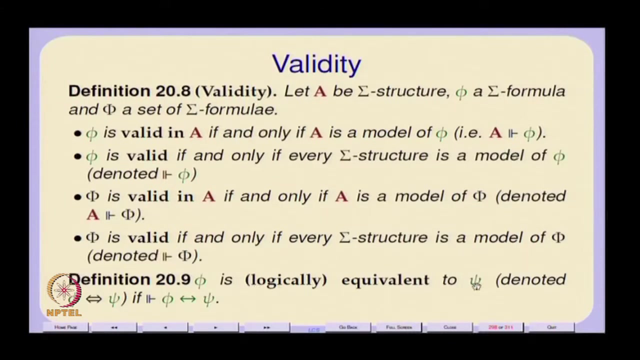 have free variables, or not, right? So validity extends propositional tautology to signatures, arbitrary signatures, yeah. So now, once you have validity, of course, you can also talk about logical equivalence. We will say that phi is logically equivalent to psi and we will use the same notation, phi. 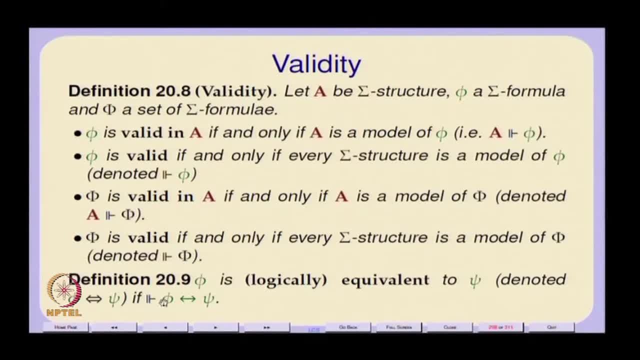 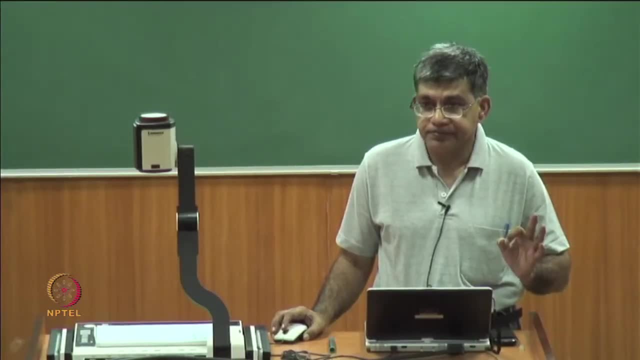 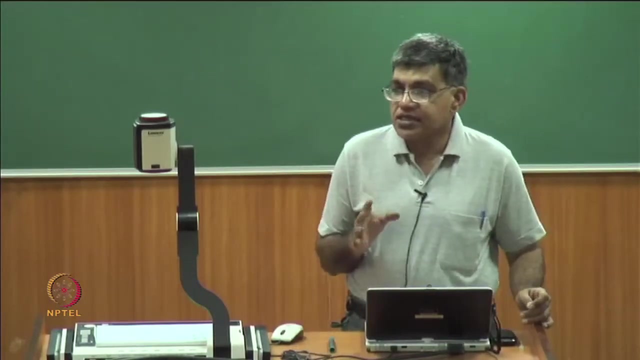 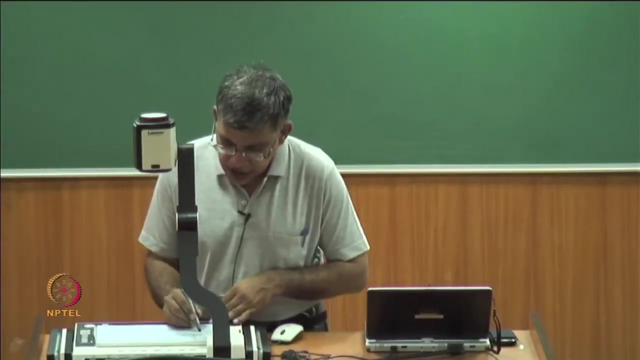 is equivalent to psi if this phi by conditional psi is valid for all sigma structures. So the importance of studying Propositional logic is essentially that now you can take all propositional tautologies, So you take any propositional tautology like this, and what you can, you can think of. I am 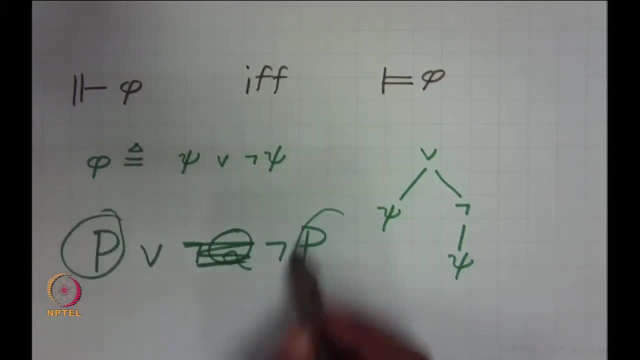 sorry. And you can think of this as essentially defining skeletons into which you can plug in first order logic formulae, appropriately right. So if you take something with more than one, like let us say, If you take a tautology like this, if you take, then basically what we are saying is for. 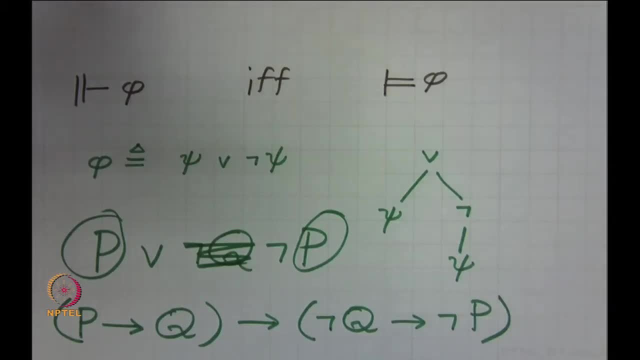 capital P and capital Q. you can substitute it by uniformly by any first order logic formulae- phi and psi may be, and what you will still get is a tautology. So tautologousness in propositional logic will be preserved. 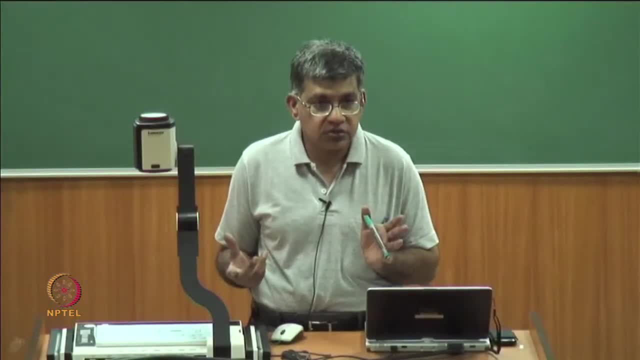 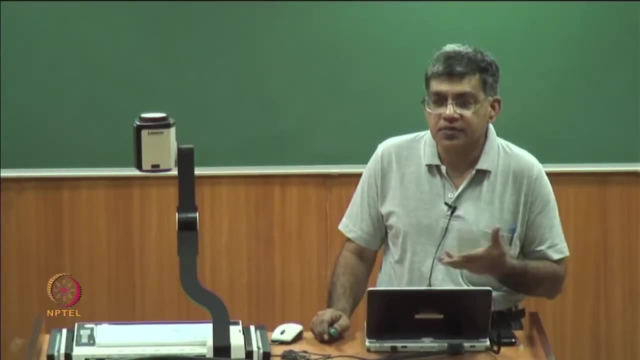 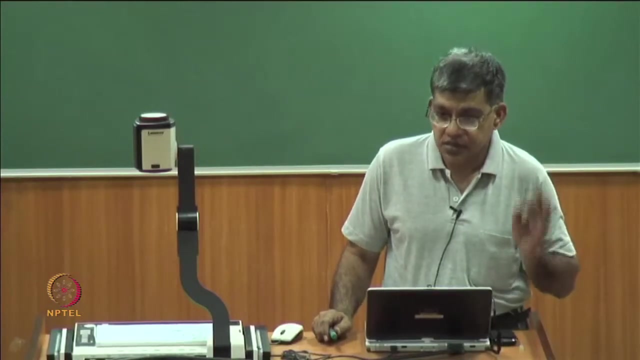 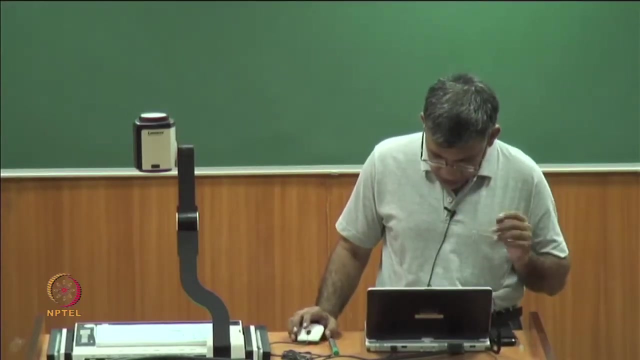 Is also preserved as validity in first order of logic, right. So the only constraint is that the internal terms inside those phi and psi should should conform to the signature given. that is it expect. for that there are no other logical reasons. So that is right. 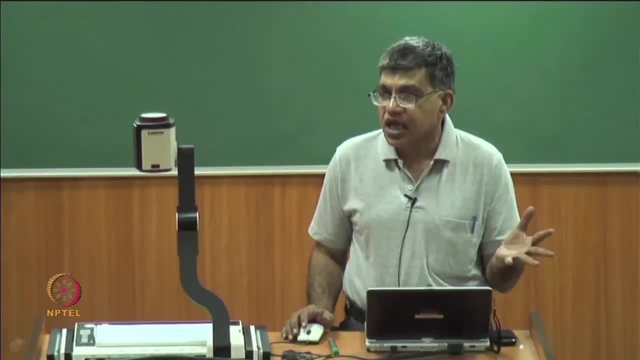 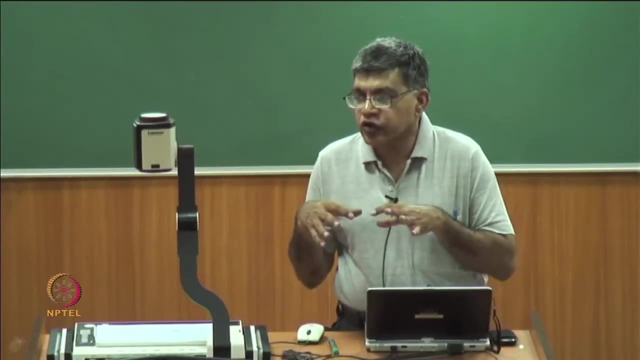 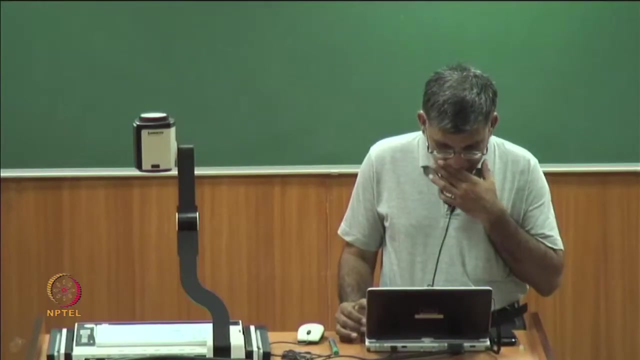 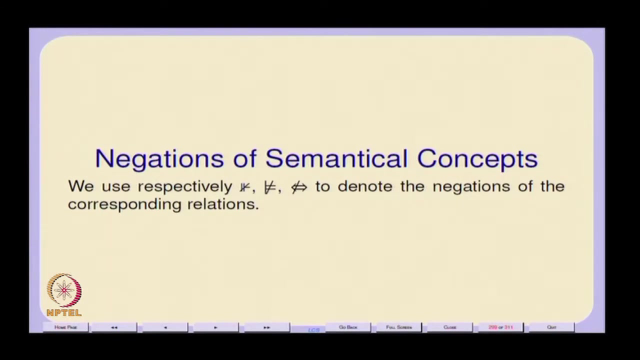 now we can import basically all propositional tautologies, skeletal structures on to which first order logic formulae may be hung uniformly. So we will take the appropriate slash versions as the negations of these semantics concepts basically invalid or not equivalent, and so on and so forth. 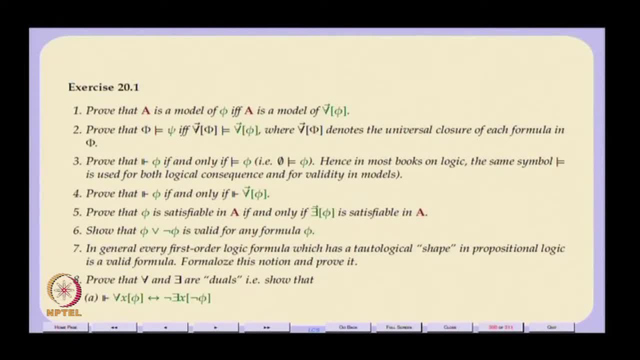 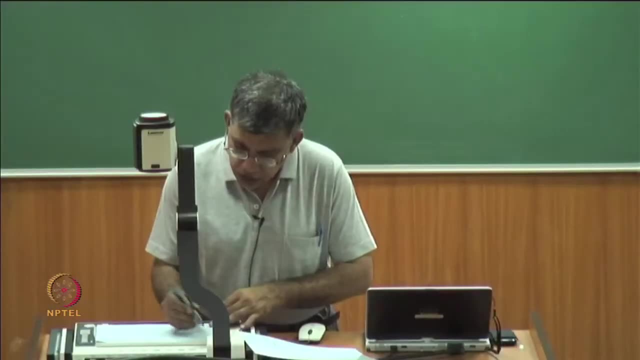 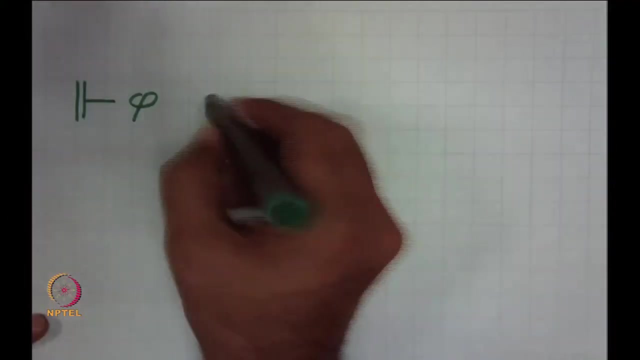 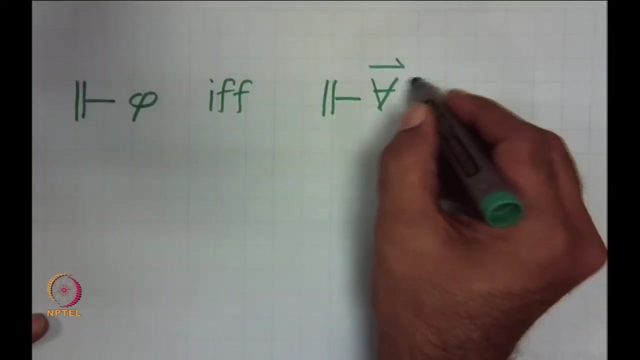 Now I have got a lot of exercises for you to do, of which there is this four. can you see this four one? So this four essentially says that you take, so you take, any formula of phi. this is valid if, and only if, its universal closure is valid. What is the universal? 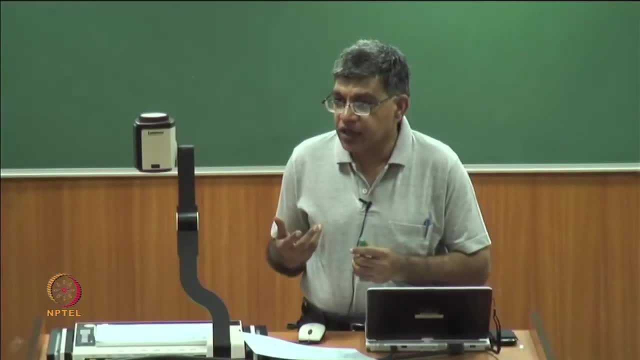 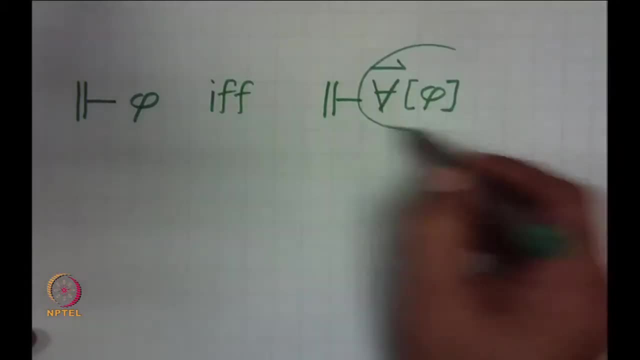 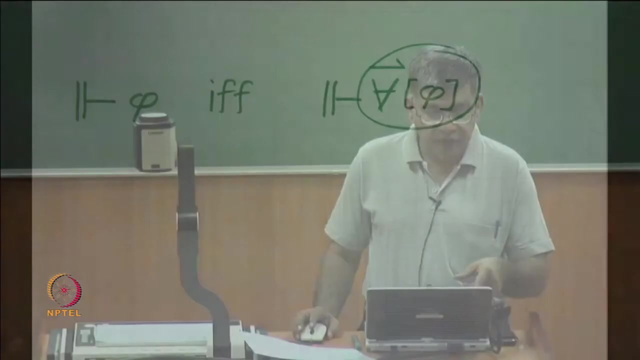 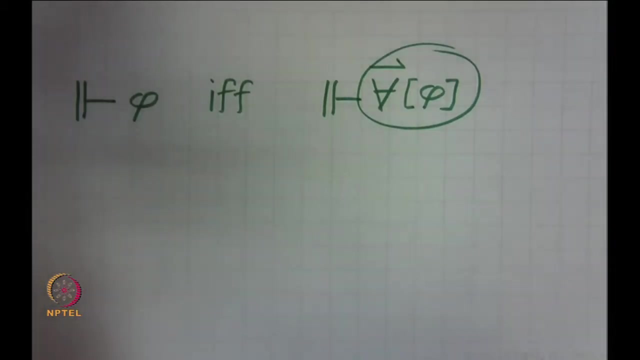 closure of phi. you take all the free variables of phi and you put a universal quantifier for all of them, So that this one has no free variables left, And this essentially the fact that validity of phi is independent of its free variables. 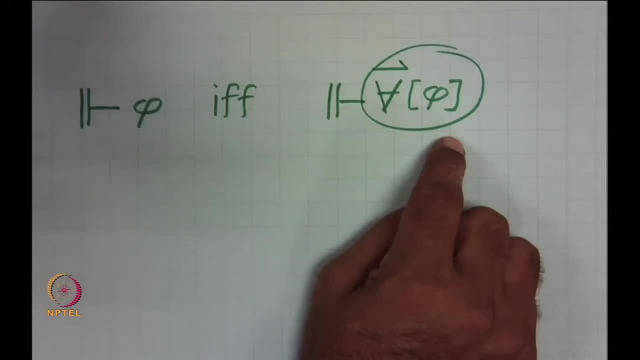 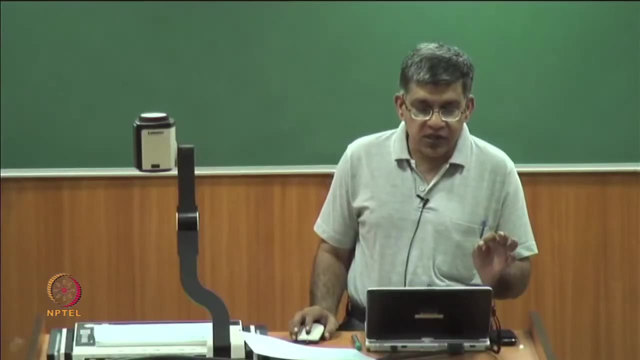 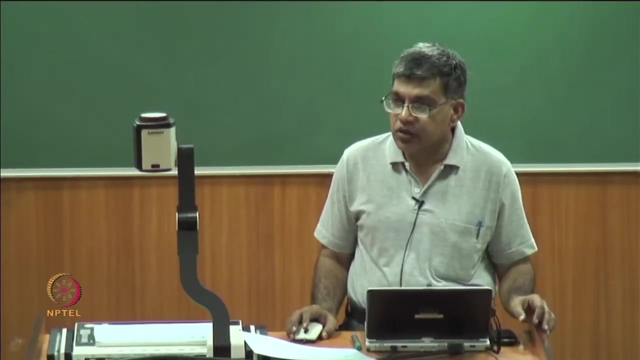 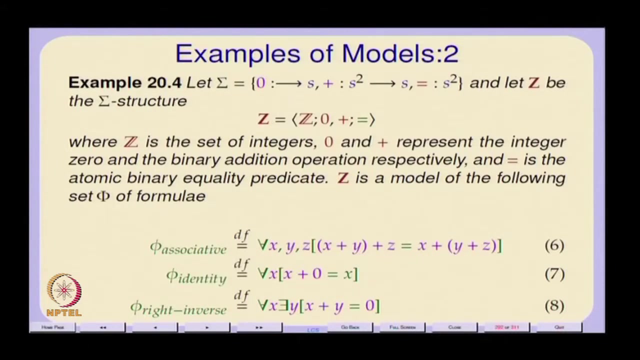 means that if you universally close it also that it remains valid. So validity is preserved under universal closure. which is why- which is good justification for why a mathematics books do not put these quantifiers before the axioms And we just, they just state the axioms with free variables, but they are essentially saying: 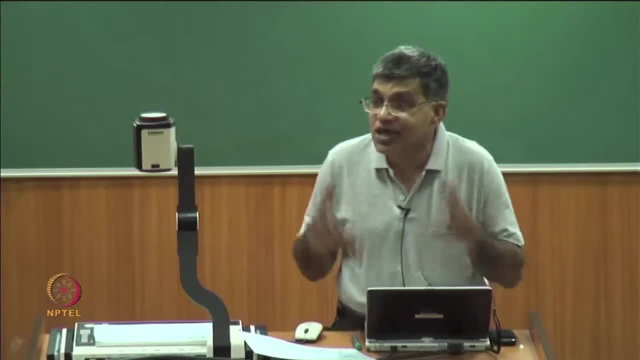 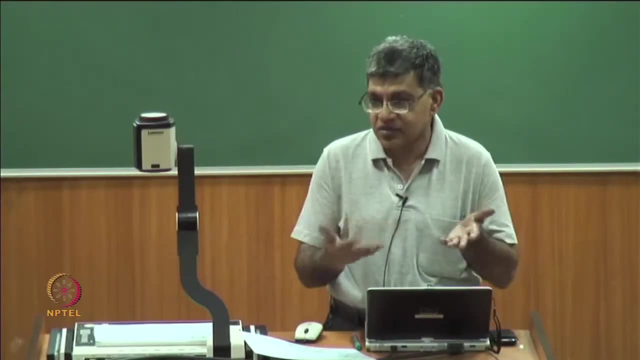 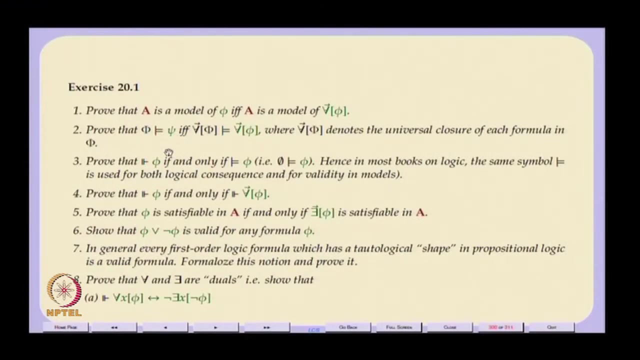 that they considering only all those structures in which these axioms are valid. So they are valid with free variables if, and only if, their universally quantified versions are also valid. so, and therefore it is perfectly consistent, right, and of course the same thing also holds for sets of formulae. 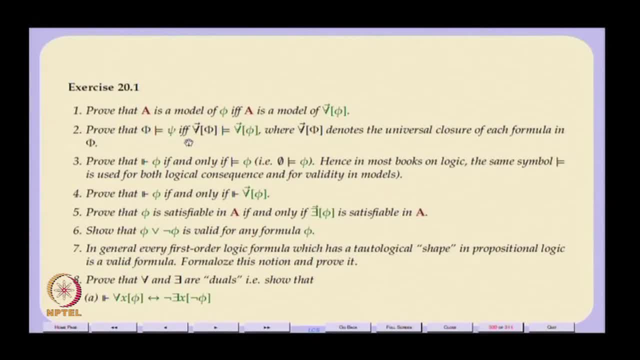 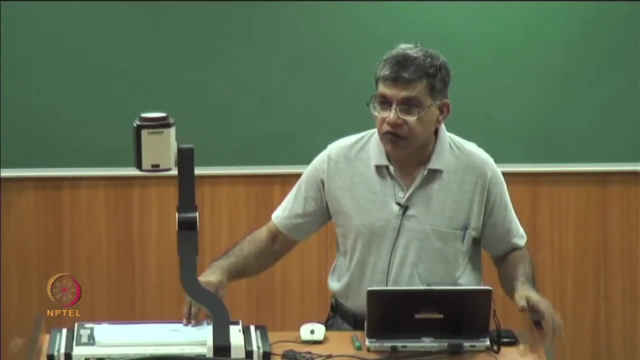 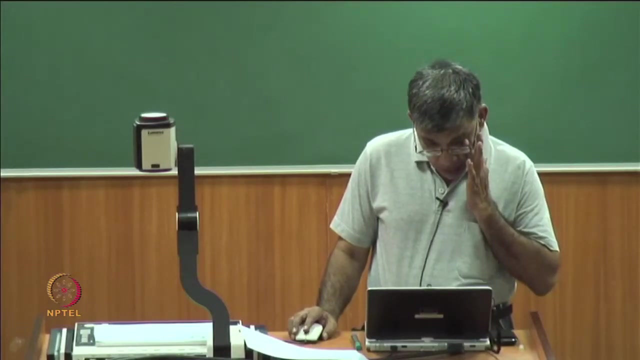 I should have probably put this, I should change the order of these two, but anyway. And the other question three essentially identifies these two concepts. so you can, but you can- prove all this from an underlying semantical model. The other important things that you have to prove is that the existential and 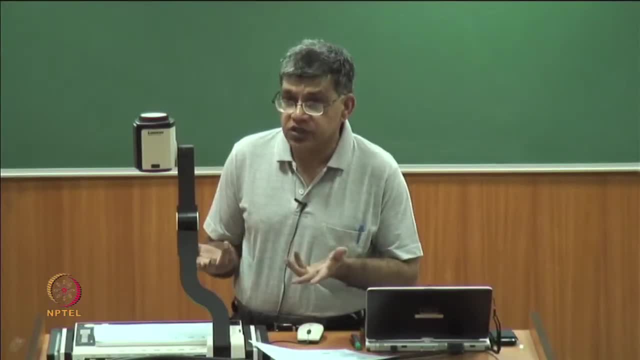 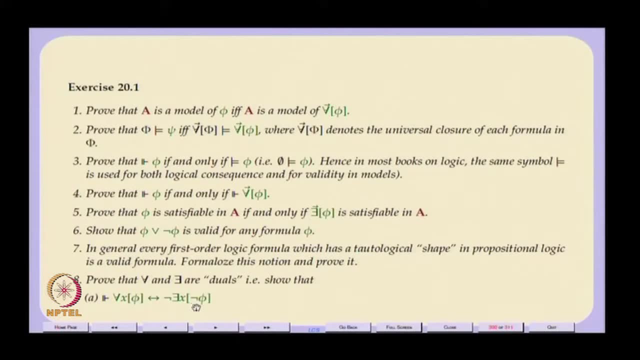 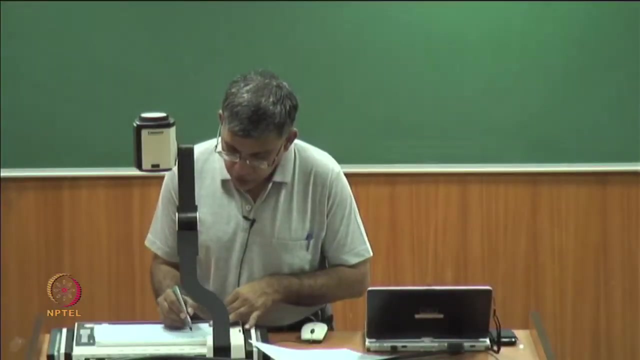 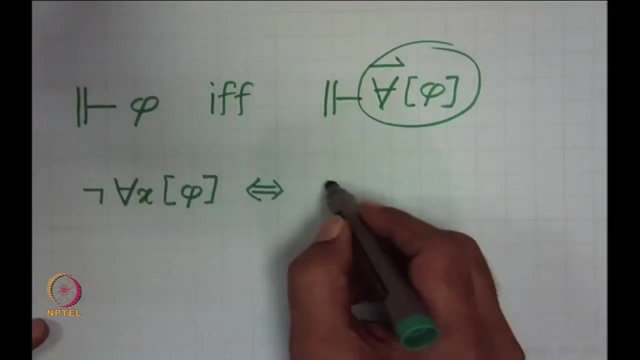 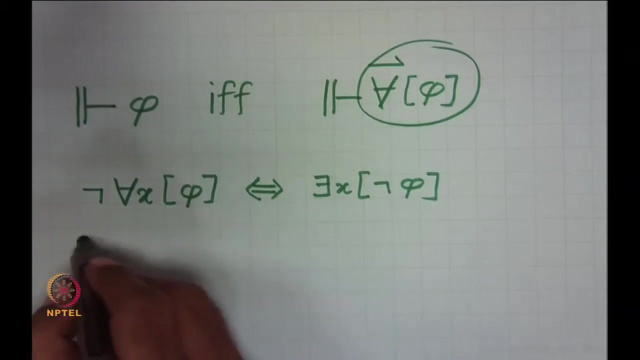 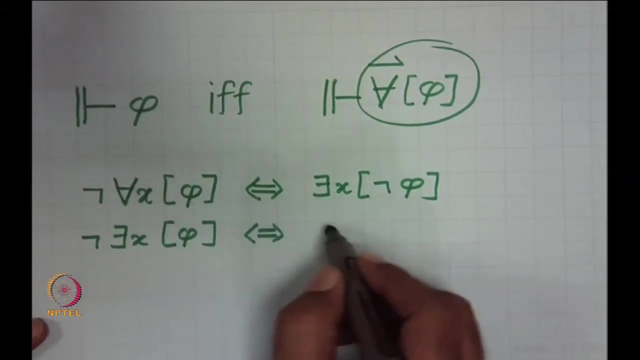 universal quantifiers are duals of each other, So they satisfy an extended De Morgan's law which essentially means that not of for all x phi is logically equivalent to there exists x, Not of phi, and similarly, not of there exists x phi is logically equivalent to for all x. 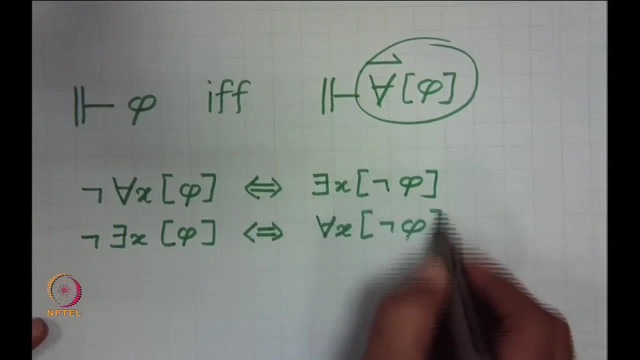 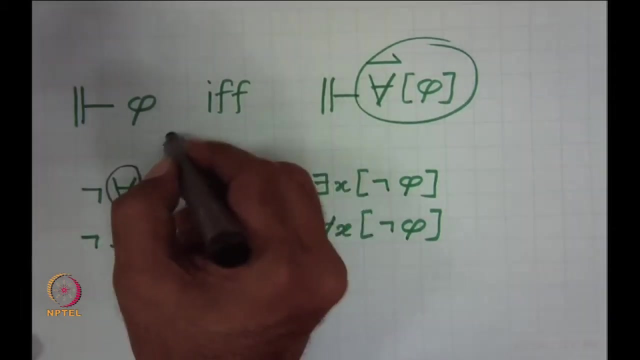 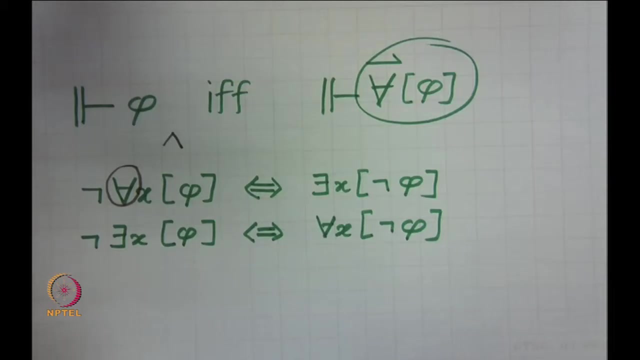 not of phi. So one way of so this is essentially like, so in a certain. so this universal quantifier is really like, and extended to a possibly infinite number of indices. Similarly, this is essentially like, or extended possibly to an infinite number of indices, So the 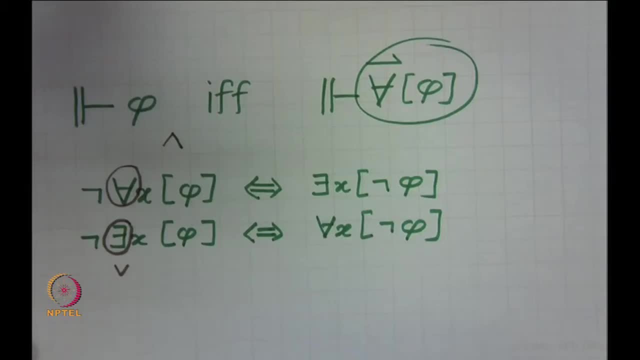 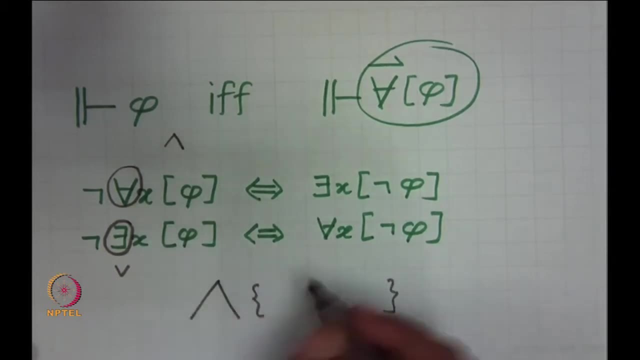 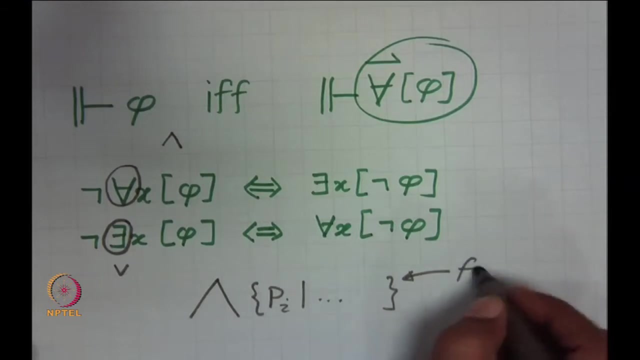 fact that The fact that a big and commutative and associative allows you to define a big and in propositional logic, but you can take a big and of various propositions only for a finite set. this has to be a finite set. what for all allows you to do is that your models are infinite sets. 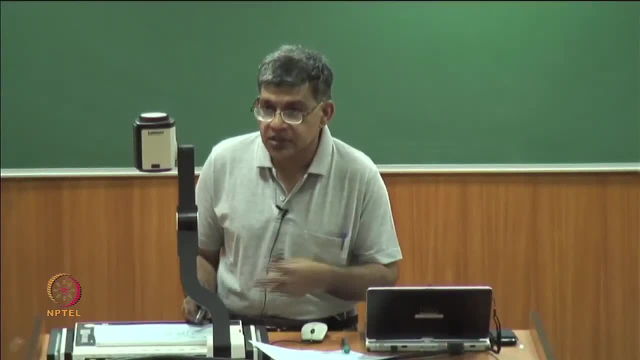 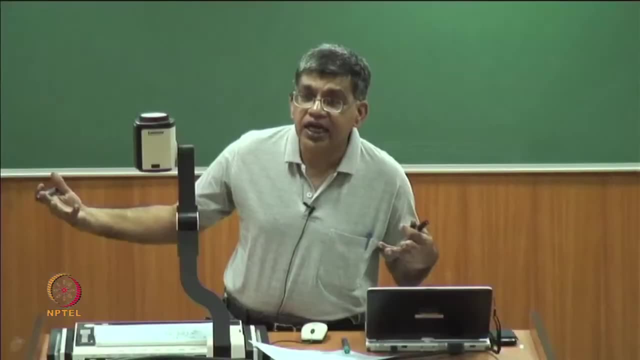 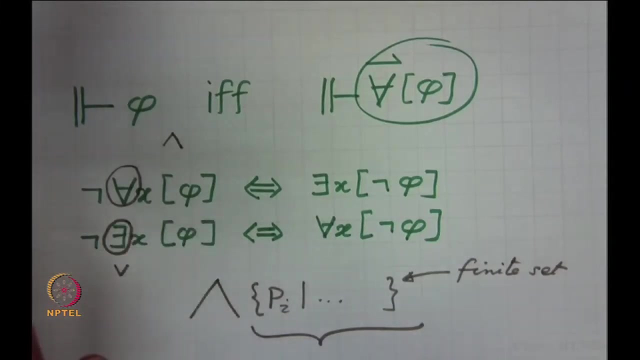 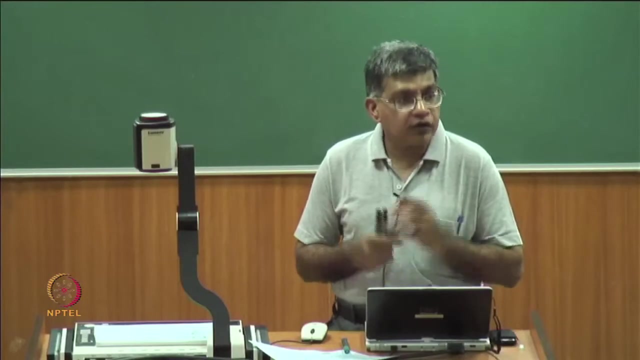 like integers or reals, then what this allows you to do is it essentially allows you to state an infinitary conjunction in a finite sentence, So you can think of the quantifiers intuitively as dealing with a finitary representation for an infinitary conjunction, or 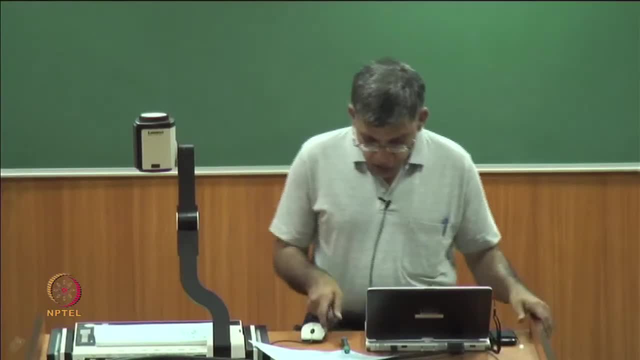 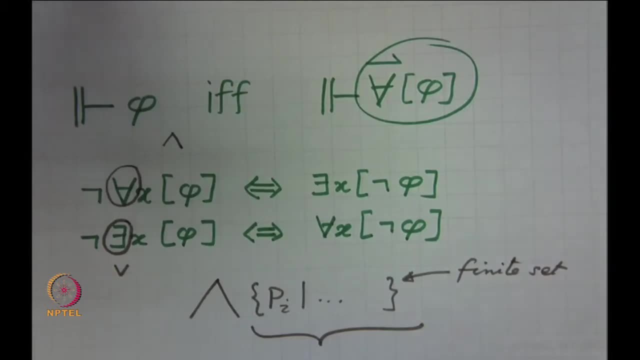 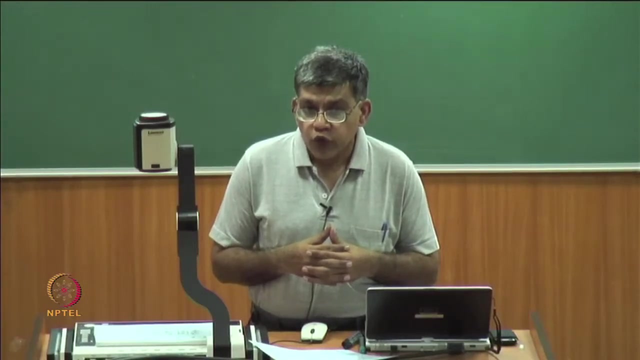 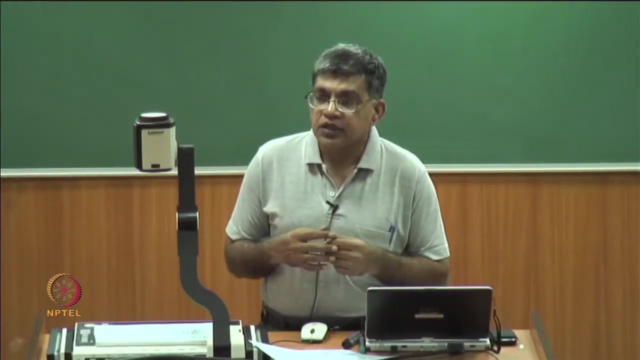 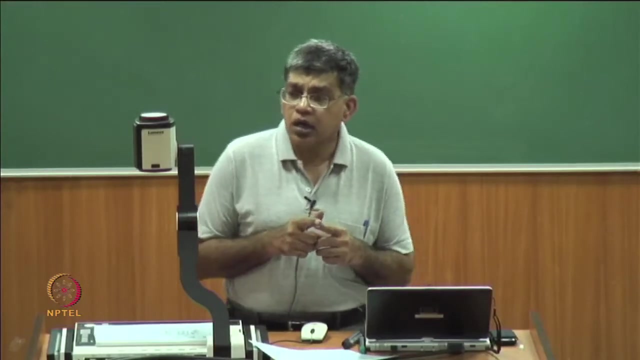 an infinitary disjunction. and so it is. so one obvious thing: supposing you have a sentence, a universally or an existentially quantified sentence, for which has only finite, which has only finitary models, Then then everything in the, in that finitary model. So every first order logic sentence can be translated into: 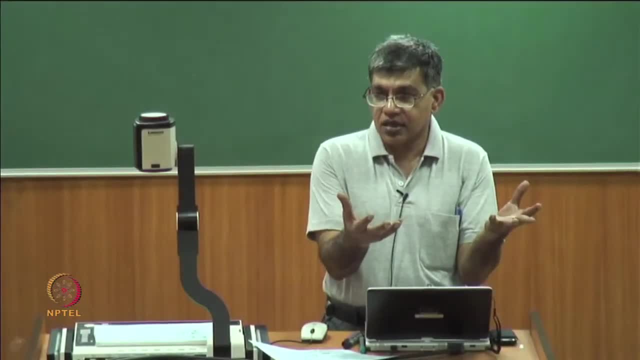 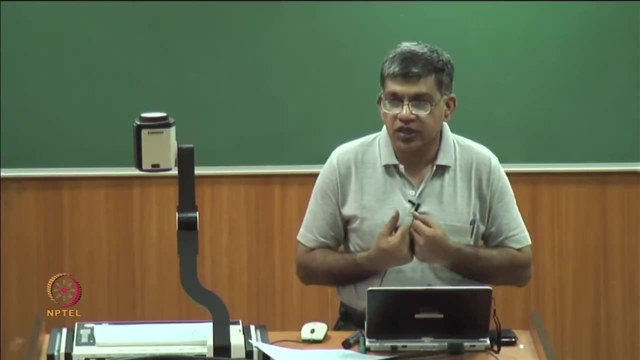 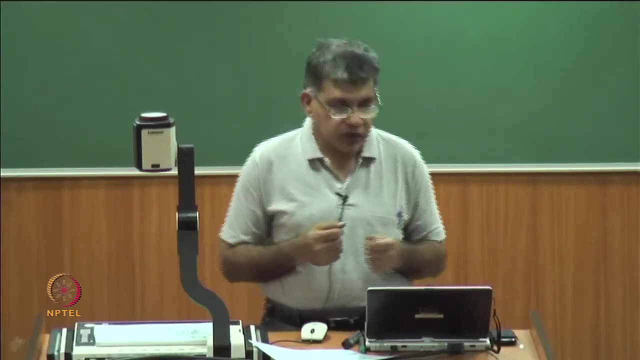 an appropriate propositional sentence there with: except for the occurrence of free variables, right. So every closed first order logic formula can be expressed in terms of a purely propositional logic formula. So one thing is, you could think of one simple example. you could. 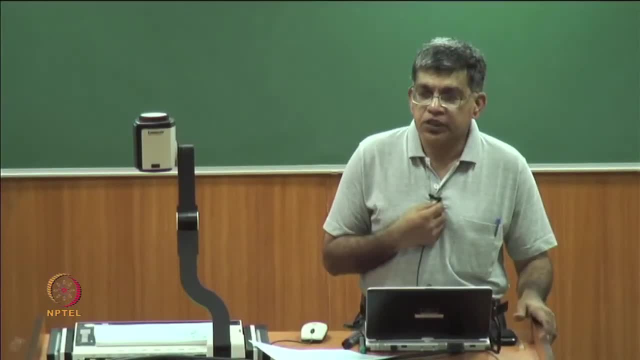 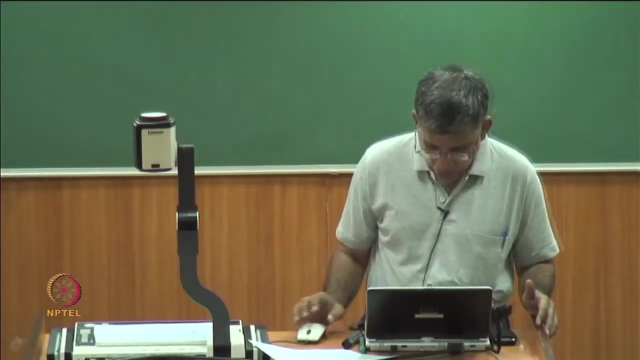 think of is supposing, I take the theory of Booleans, it is a finitary model which just its carrier, set with 2 values. So take this itself as your sigma, right? I mean? so where is that? So we had, we had something. 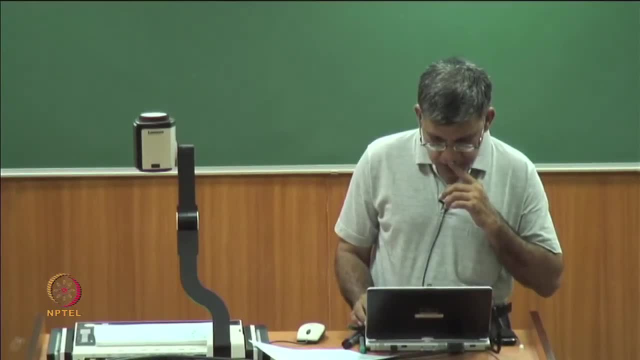 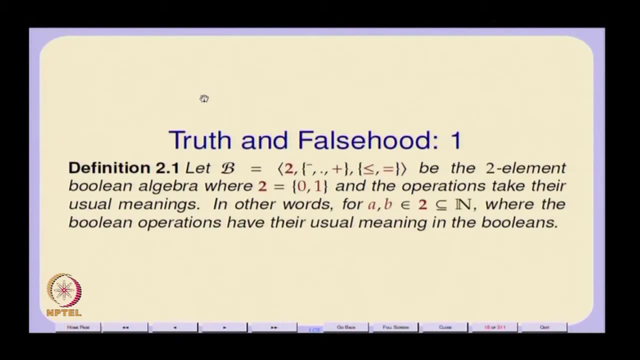 we had the entire algebra specified somewhere right, that was in the notion of truth. here is the signature. So you take this signature of Boolean, which is just a two element carrier set. all expressions in this can be evaluated and they will evaluate only to this, to one of these. 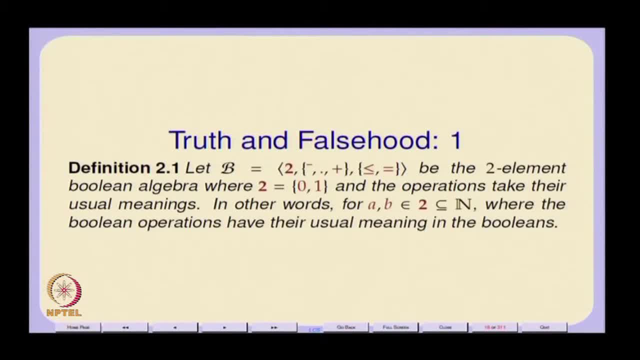 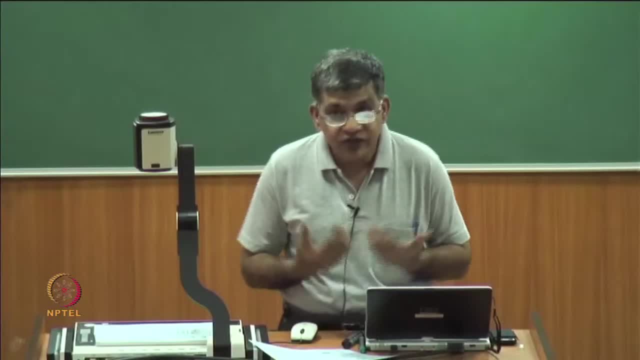 two values, You take a first order logic of Boolean algebra. I mean, after all, our signatures are arbitrary. there is absolutely no reason why we cannot define a first order logic of Boolean algebra. So if you take a first order logic of Boolean algebra, what you can actually do is: you can 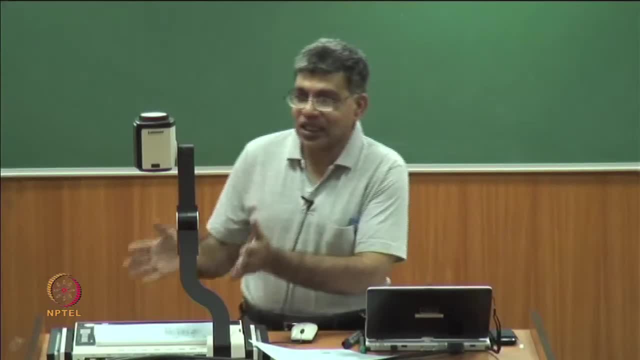 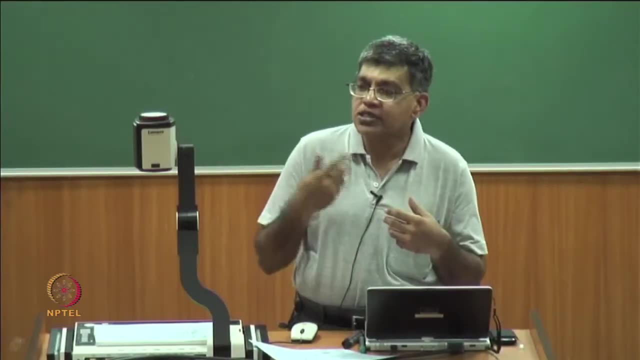 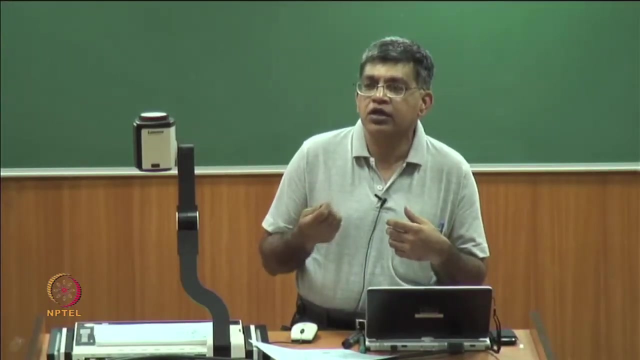 take all universally quantified sentences in the first order logic of Boolean algebra and translate them into purely propositional sentences by replacing all the variables by the values for 0 and 1. they, whatever are your violet versions of 0 and 1, because those are. 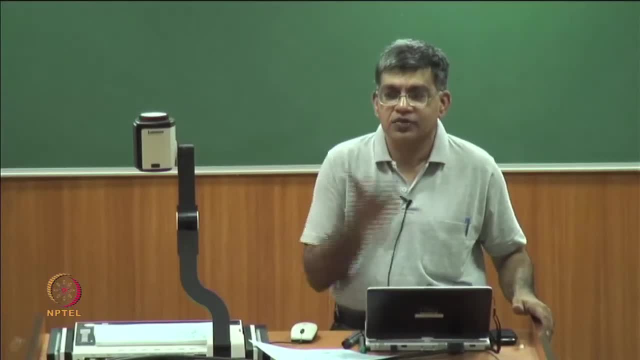 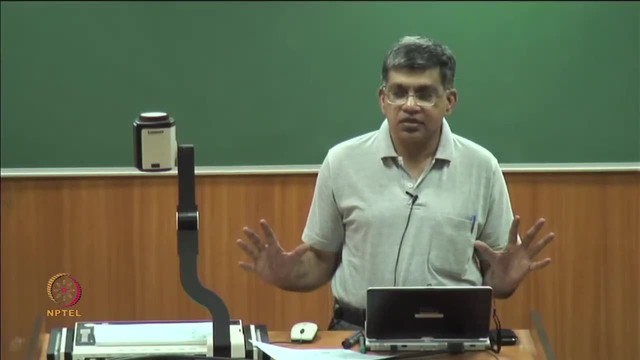 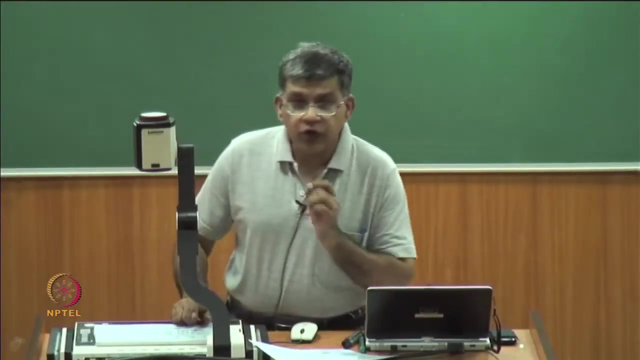 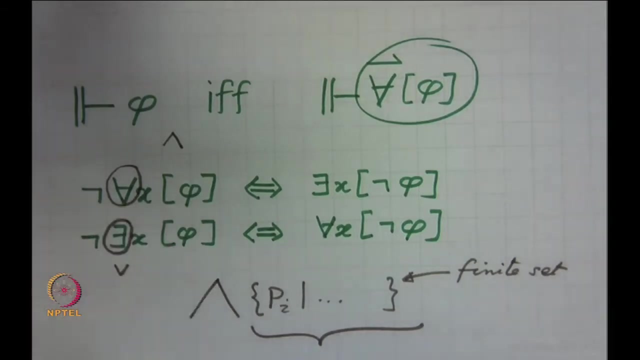 the terms. it has two constants: 0 and 1.. So you have a violet 0 and a violet 1 and you replace it and you have purely propositional statements describing Boolean algebra. So, for finitary models, for finite models, all your universe, universally quantified formulae. 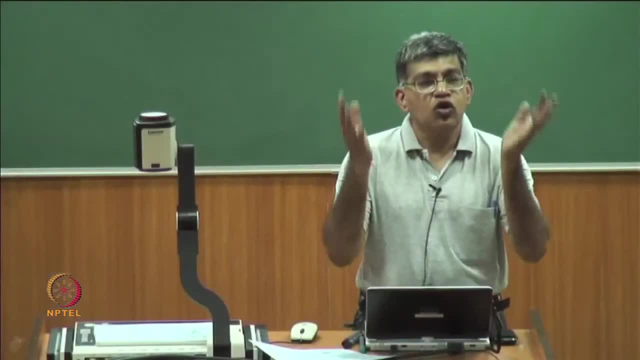 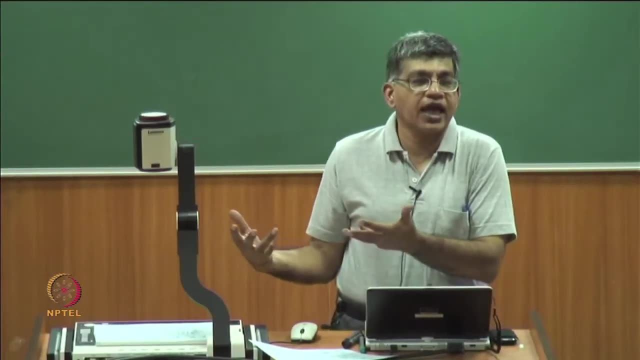 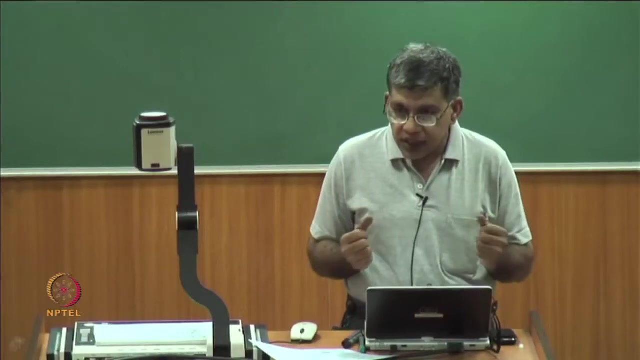 and your existentially quantified formulae will reduce to pure propositional formulae, with just being replaced by all the possible values from that carrier set. that is it So. that is so you can think of, therefore, one thing. so the idea of parameterizing propositions, 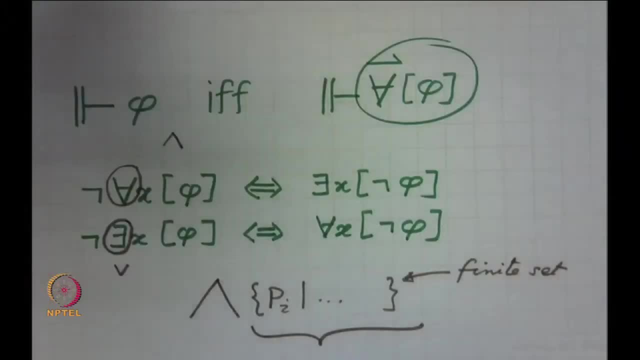 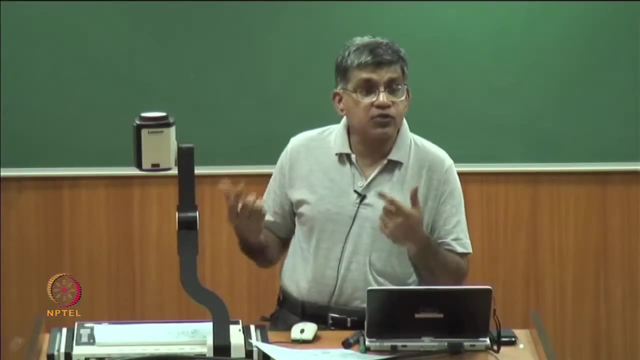 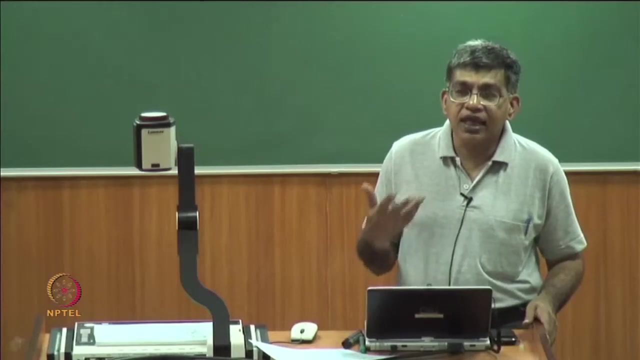 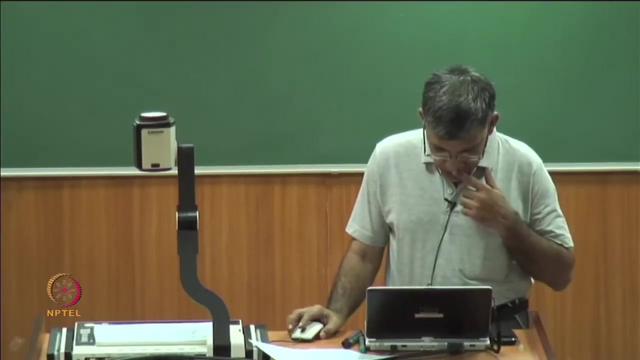 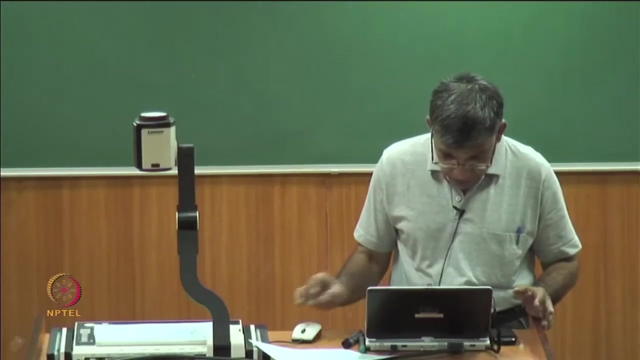 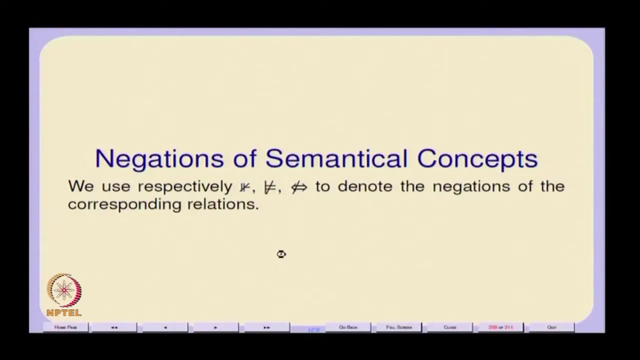 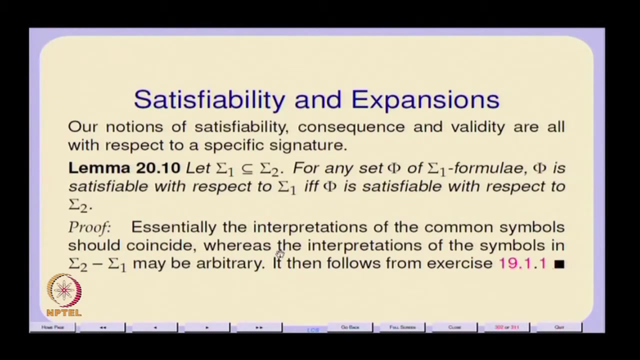 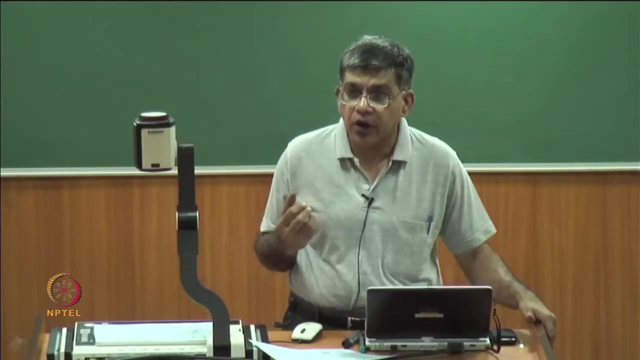 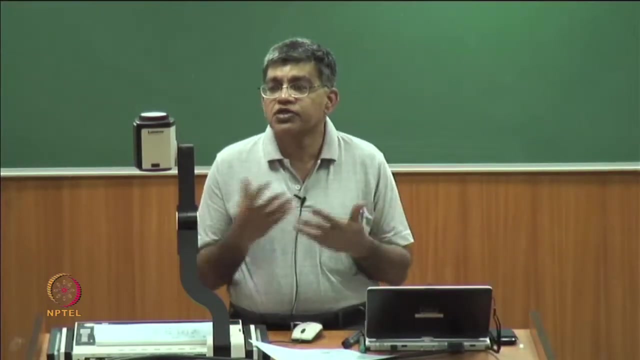 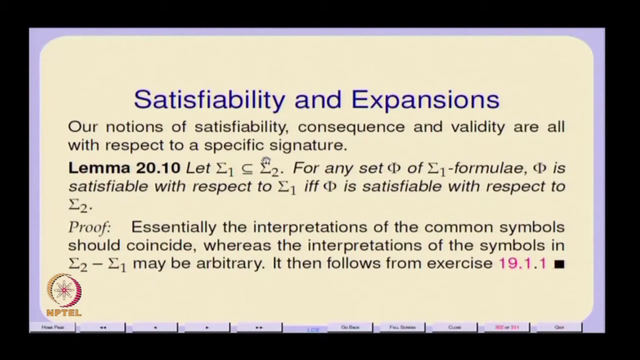 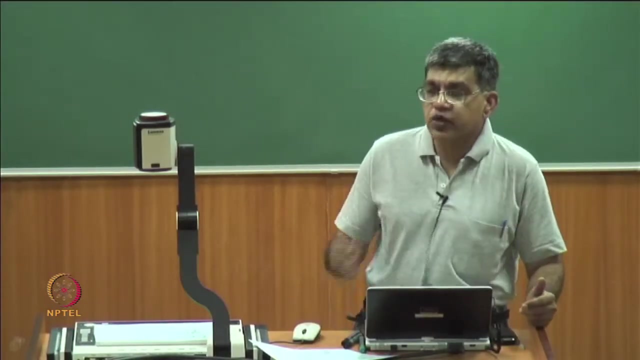 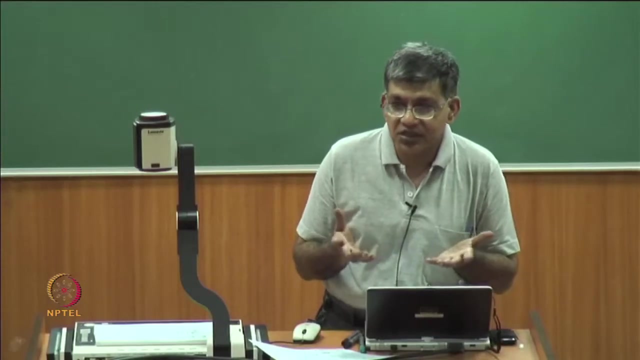 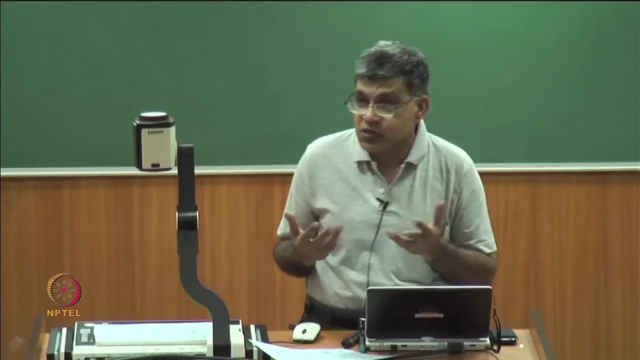 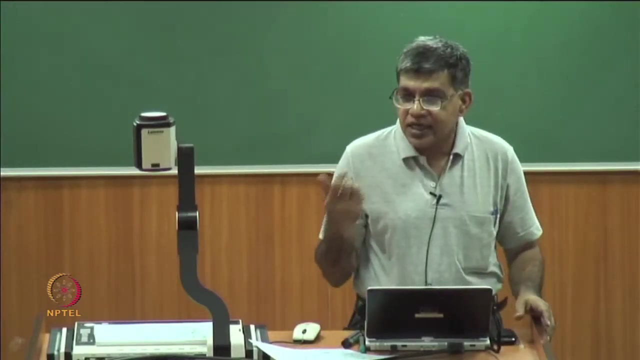 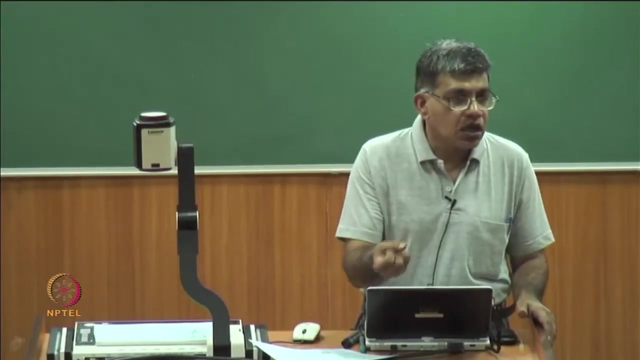 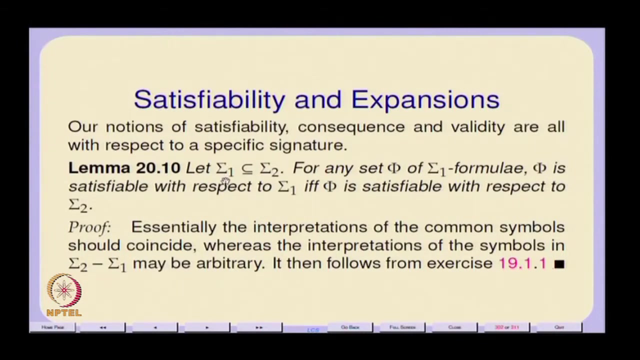 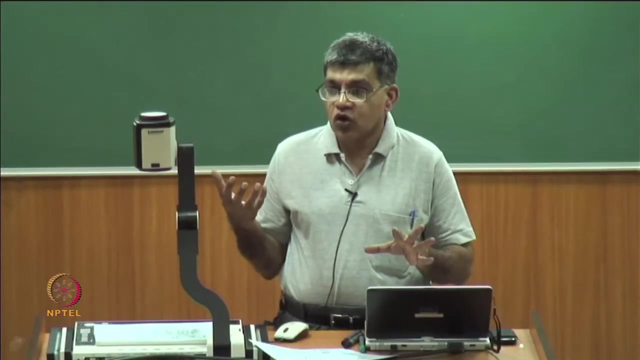 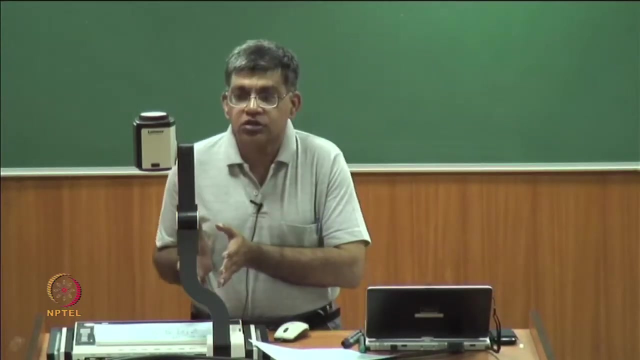 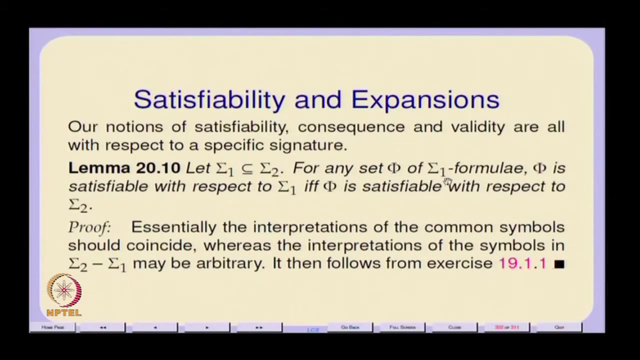 to get predicates is to allow for the fact that we want finite, we want to, we want finitary representation of sentences, for formulae or facts which might be infinity in nature. So any arbitrary interpretation, it does not matter, and then you can prove that.